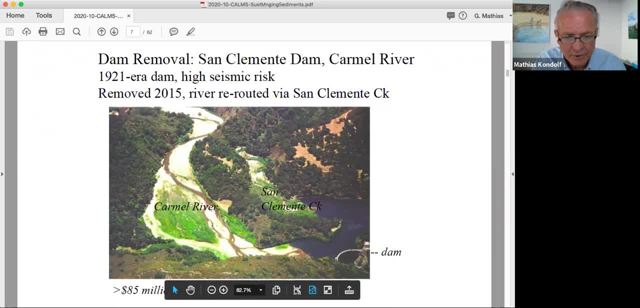 it was basically filled with sediment, but you can see this huge wedge in the lower part of the Carmel River flowing into the dam. This is a huge wedge in the lower part of the Carmel River flowing into the reservoir. And then here is San Clemente Creek, a major tributary. 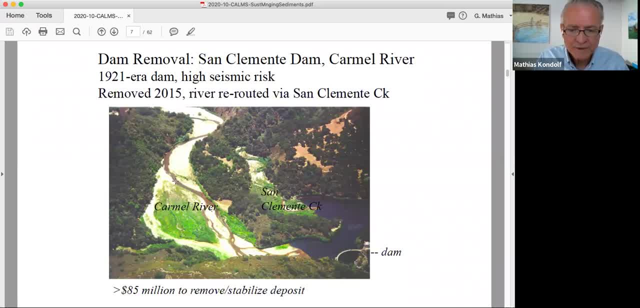 Well, the issue with removing a dam like this and San Clemente Dam was seismically unsafe. It seemed that the foundation didn't go all the way down to bedrock, It was in gravel, basically. So there was some urgency to remove the dam And that finally happened in 2015,. 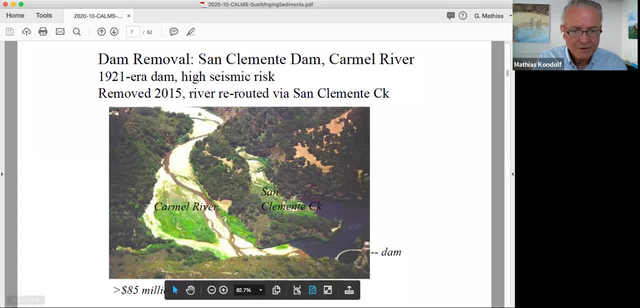 and the way they managed it was that they had to manage the sediment. They couldn't just let all this go, So they stabilized the sediment in place. They cut a channel through this ridge so that they could reroute lower Carmel River through the bed of San Clemente Creek and then 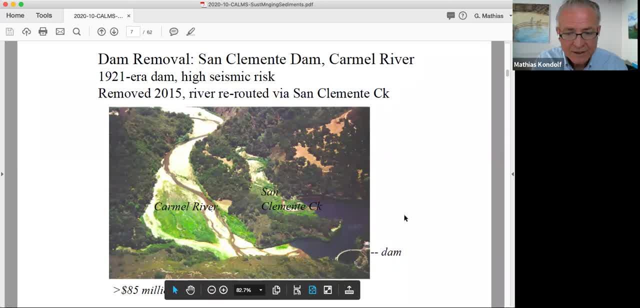 it rejoined the original channel bed down here. So it was actually a pretty clever solution to a very difficult problem, because there would be no way you could truck all that sediment out of there, given the state of the roads and the political swing of. 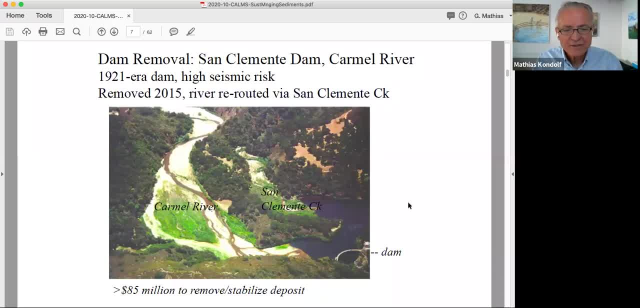 the people who own the biggest states around there, And even things like a conveyor belt or a sluice pipe that would carry it over the ridge, that just seemed to be infeasible. So this was a pretty successful dam removal And in this case, 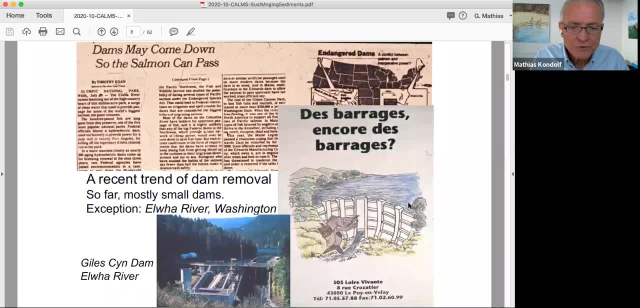 they had to stabilize the sediment in place. Now, more and more, we're seeing this trend of dam removal in the global north. It's quite the opposite in the global south, where dams are being built like crazy. But there have been other examples, most notably on the Elwha River. 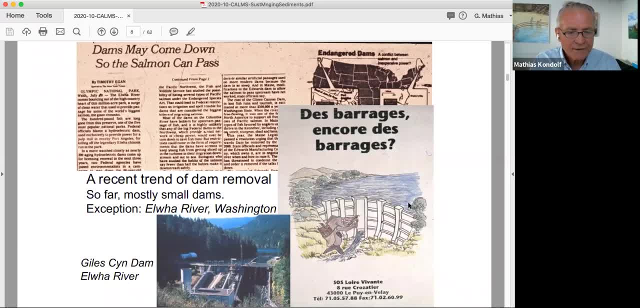 on the Olympic Peninsula in Washington, where the Elwha and the Glines Canyon Dam were removed, And this is a very different situation because, unlike the dams in California that I mentioned, all of which have very high-priced real estate downstream, right along the banks of the river. 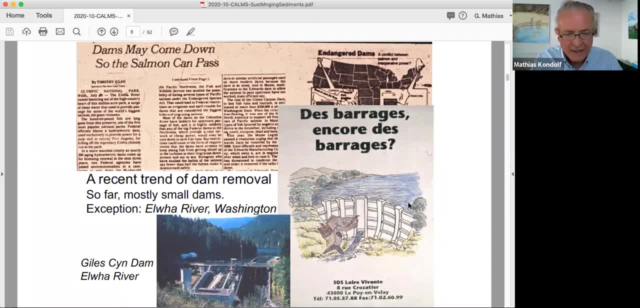 and sediment issues. So as sediment comes downstream, you're going to have all these problems. On the Elwha, the downstream reaches were not populated and they were mostly owned by the Indian tribe- Klallam Indian tribe, who was pushing to get the dams removed. 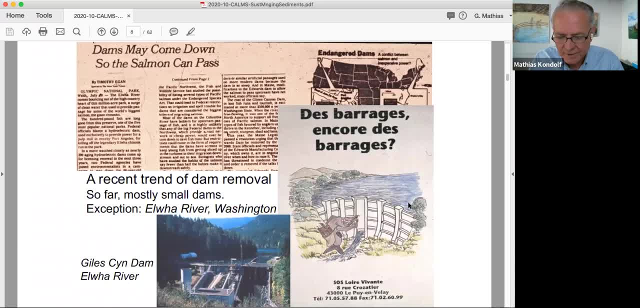 And in this case, the dams were owned by a lumber mill and they were perfectly happy to accept some substitute power and have these dams taken off their hands Because, in terms of trying to relicense those with FERC, that would have been a nightmare for them. But we see also this tendency. 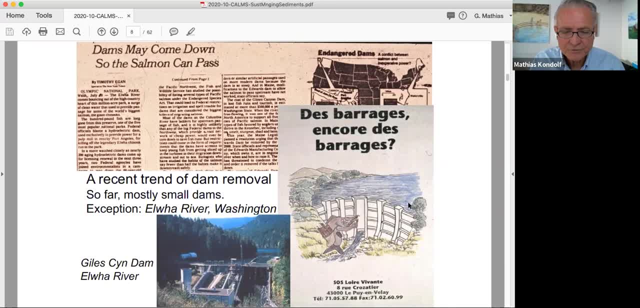 to remove some dams in Europe. This is a poster from an NGO in France on the Loire River, where they have been removing some dams to try to open up habitat in the upper Loire and the Allier, a big tributary. 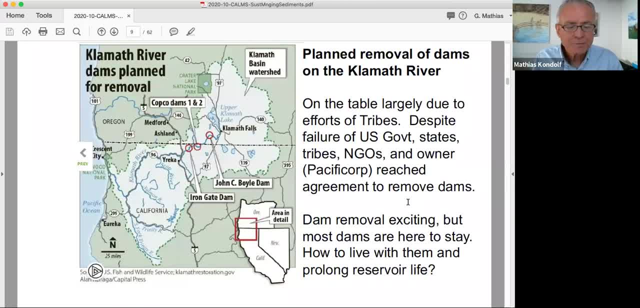 Okay, but the biggest project so far, the Elwha is the biggest dam removal we have, certainly in the US, but that will be dwarfed by the Klamath River dam removals which are planned for dams on the Klamath And originally the US government was going to contribute to this. 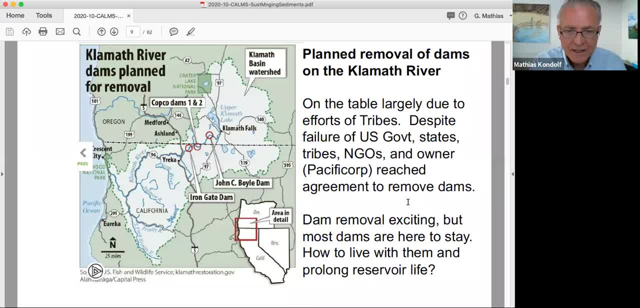 Congress never came through for political reasons, But the other parties- the tribes, the states, the NGOs and the owner of the dams Pacificor- reached an agreement to remove the dams anyway And that's been set back about a year because of COVID issues, But I think it will finally happen. 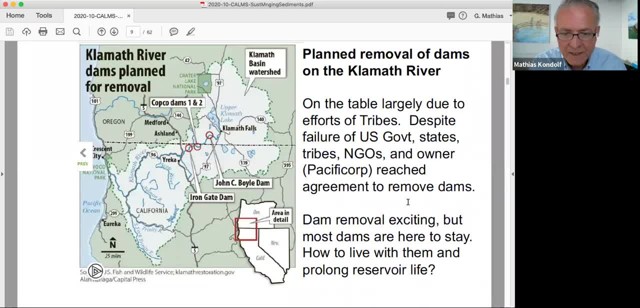 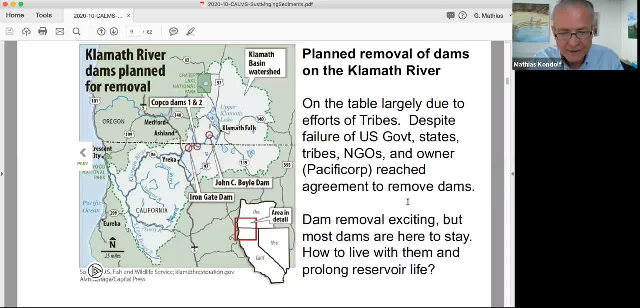 to get rid of them, And we are going to have to get rid of them, And we are going to have to get rid of them. And new dams in the Global South way faster than any dams are being taken out in the industrialized world. So really, the question is: how do we live with these dams? 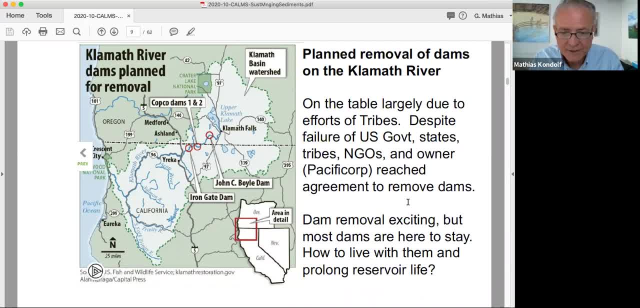 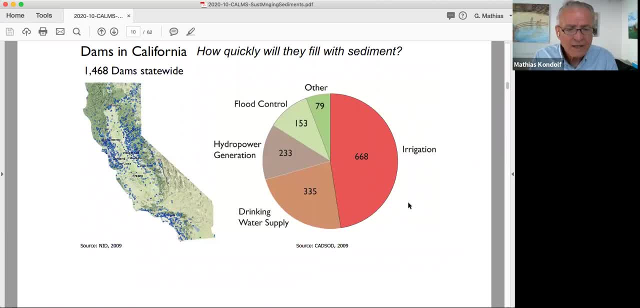 and how to prolong the reservoir life, which is threatened by sedimentation in many cases. So we will come back to that in a moment, But I wanted to look a little bit at the dams in California. My PhD student, Toby Mynee, and I asked the question: how quickly will they fill up? 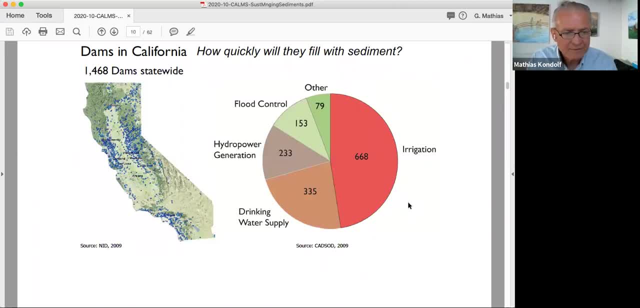 Toby Mynee and I asked the question: how quickly will they fill up? we were motivated by by places like the Matilaha and San Clemente. How common is this? Well, we have over 1400 dams statewide. These are dams large enough to be regulated. 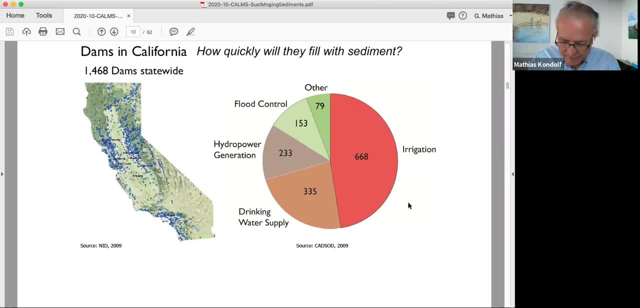 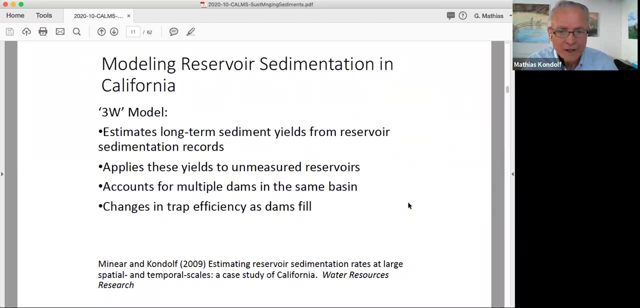 by the Division of Safety of Dams And, as you can see, mostly for irrigation, but all sorts of purposes. We developed something called the 3W model, which estimates long-term sediment yields from existing sedimentation records in this case. So we scoured the databases and the literature. 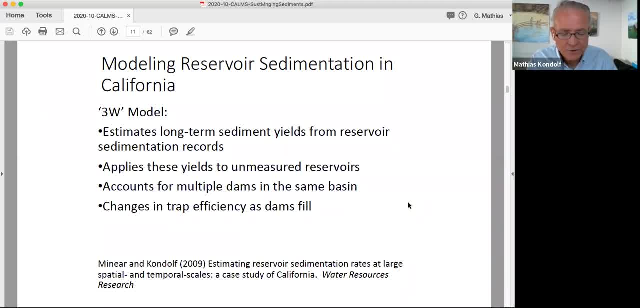 and contacted some agencies to get sediment yields for as many reservoirs as we could in the state of California, And then we used the existing geomorphic province delineations that have been developed before by the California Geologic Survey and other experts, And then, within each of these geomorphic provinces, 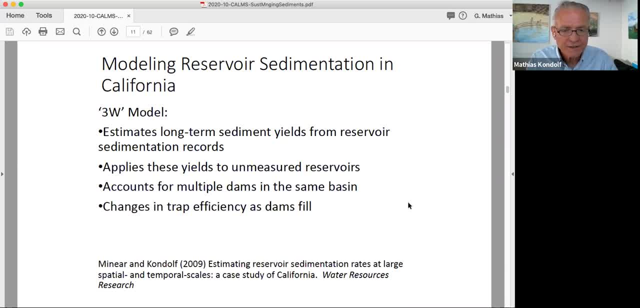 we compiled all the reservoirs of sedimentation data so that we could come up with median sediment yields for those regions, for each province, And the kind of disappointing thing was how few data there are out there. Very few of these reservoirs have had sedimentation surveys. 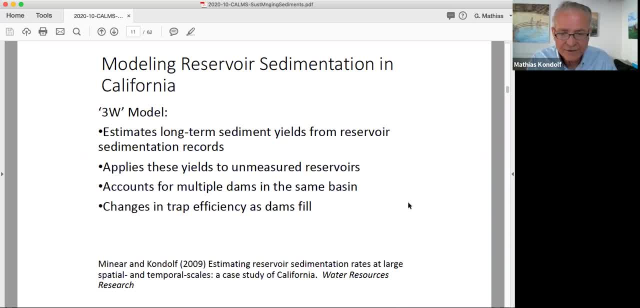 And many of the sedimentation surveys that you can find. now the data, they're from the 40's or the 50's, which is really kind of surprising because, anyway, the data was brought from the 40's or the 50's, which is really kind of surprising because, anyway, 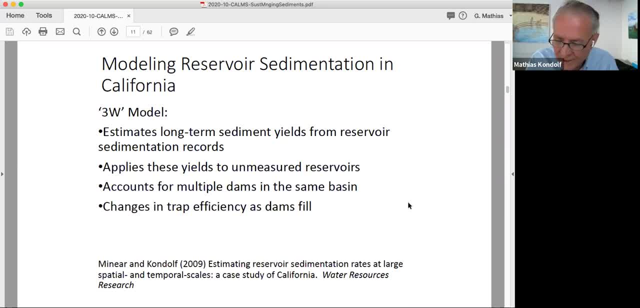 anyway, people were more concerned about the issue then, evidently, than they are now, and it was a way more work to do it at that time. i mean, today we've got sonar, we can go out, i mean our. our biggest error now is just trying to reconstruct what the pre-dam topography was. 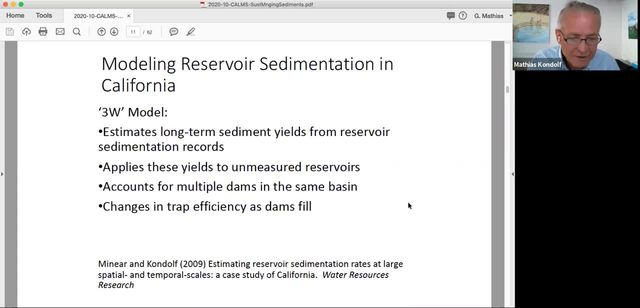 because we have, you know, you know, at best 20 foot contour maps to, to, to deal with uh, for the pre condition. but we can get the current condition very quickly and easily, cheaply and and accurately. but but very few reservoirs have had sedimentation surveys. 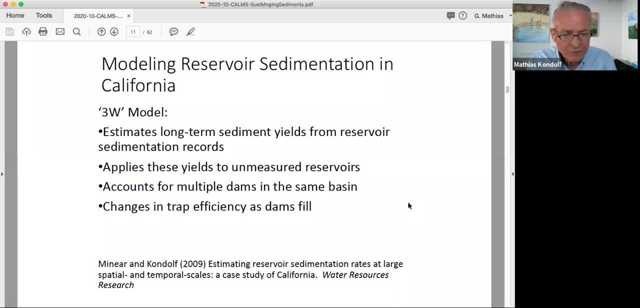 but anyway, we took the rates that there were and then we applied those to, uh, the entire province and unmeasured reservoirs within the each geomorphic province, and our model accounts for having multiple dams in the same basin. so so, if you are trying to estimate the sediment yield, 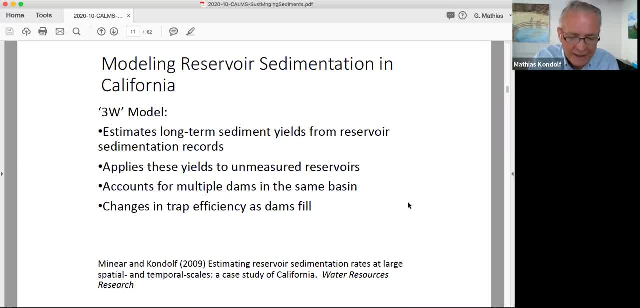 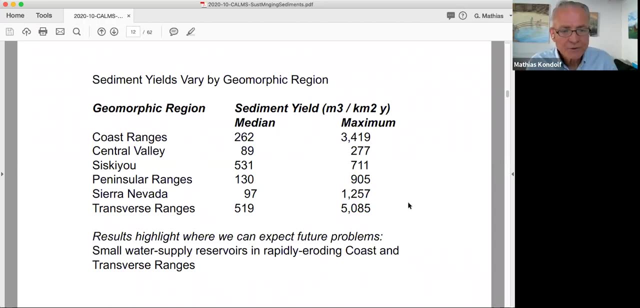 from the sediment that's accumulating in reservoir a. you take into account that there's reservoir b, c and d upstream and those are already trapping sediment and then, as these uh reservoirs fill with sediment, their trap efficiency changes. so we came up with the sediment yields by geomorphic region. 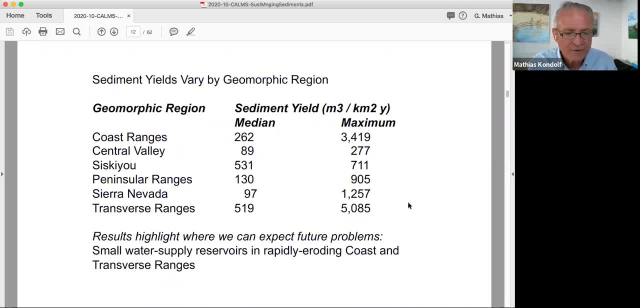 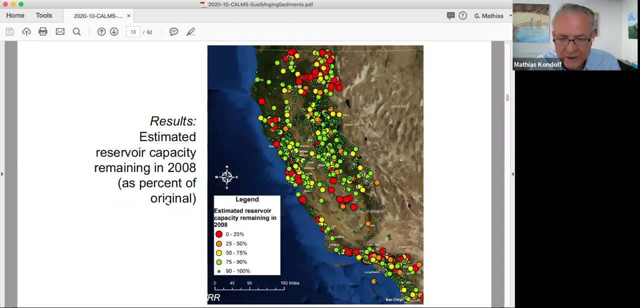 some of these are influenced by, you know, uh, very low ends, but uh, but we use these to highlight where we would expect future problems, and they are basically in the transverse and coast ranges of california where we see a lot of the problems emerging, and that's, of course, where 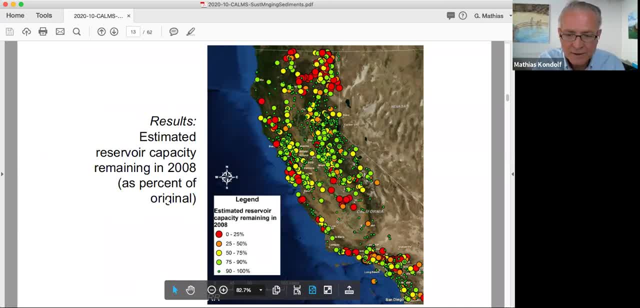 we have the big four already: malibu, uh, matilla ha, san clemente and and searsville. but if you see, here these are our projections for reservoirs that would have less than 25 percent of their capacity remaining today or 10 years ago. this is 2009, so these would be the the red dots and, uh, some of 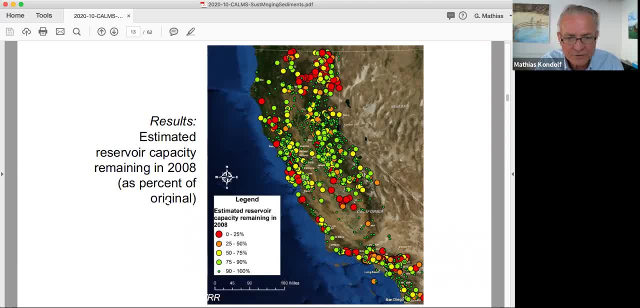 these up here are really um, small, um kind of inconsequential reservoirs, but a lot of these are are, you know, are enough to create problems. uh, the matilla ha dam is estimated to that'll cost 111 million dollars to remove. uh, the san clemente dam of the carmel: the price tag was given at 85 million, but that was over that. 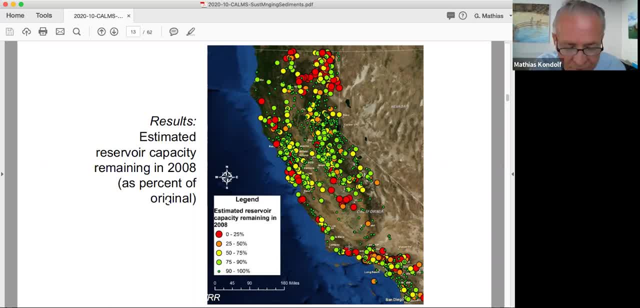 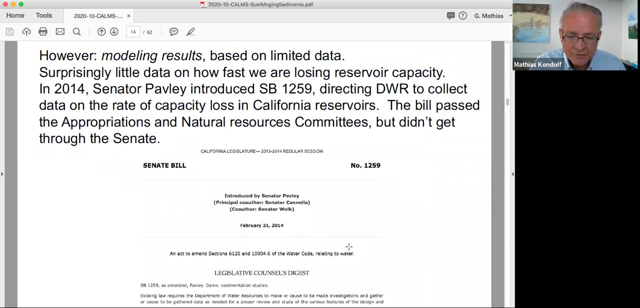 was price tag was out there like five years before the dam was actually removed. i'm sure it turned out to be way more than that. yeah, so these are very expensive things to deal with when they fill up and, as i mentioned, our study was extrapolating from very limited data. 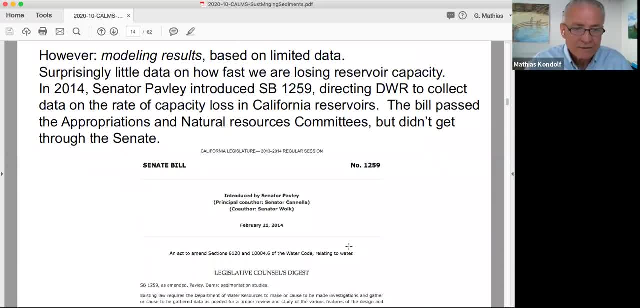 and we were surprised at how little data there were. um inspired by these results, senator pavley introduced sb 1259 in 2014, which would have directed dwr to collect data from the san clemente dam. and to collect data from the san clemente dam. 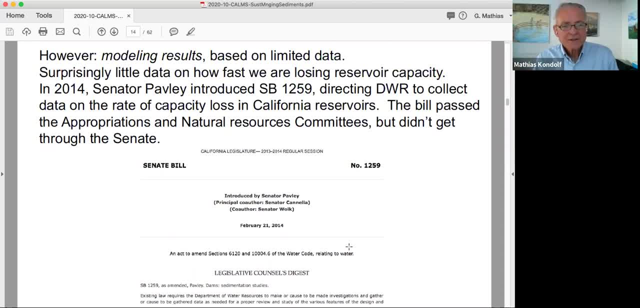 on the rate of capacity loss in california reservoirs. so the bill made it through the appropriations and natural resources committees, but it didn't get through the senate itself, so it died. so i i was surprised that collecting data on something as basic as this was controversial. but 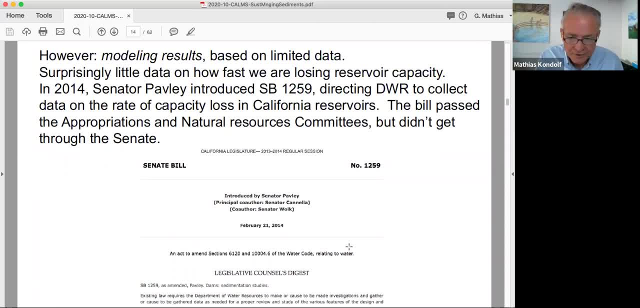 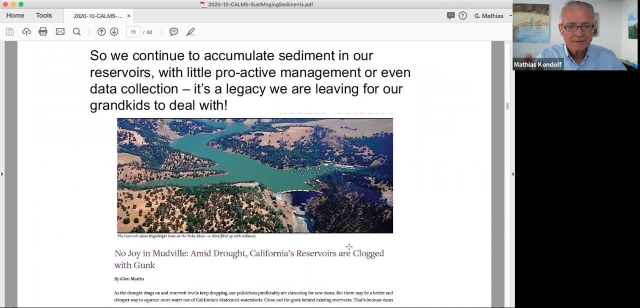 anyway, there there were some interests that were opposed to this. so we can blissfully go on in ignorance and, uh, you know, we don't have to worry about it. we have no information, so therefore the problem doesn't exist, but our grandkids will be able to deal with it in due time. 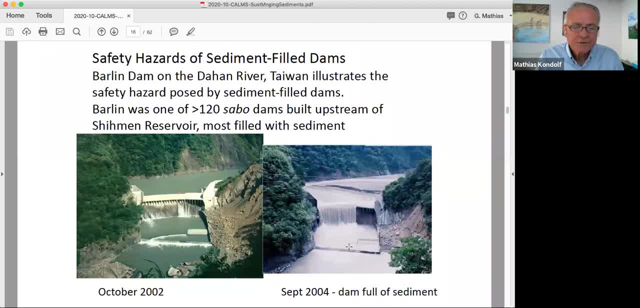 now, um, there are a number of safety hazards with sediment filled dams, especially in uh, in seismic country. um, and uh, and i know, uh, you know, anderson dam on coyote creek is a perfectly good example, uh, but looking at uh this dam, i find this uh. 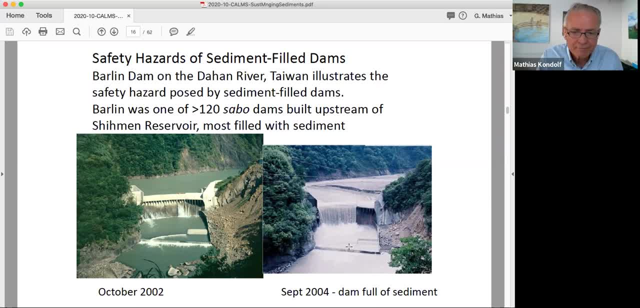 a fascinating case study. this is barlin dam on um on the dahan river in taiwan. so the there's a big reservoir in the dahan river called the shuman reservoir. it provides water for taipei and also for the taichung area, the the silicon valley of of taiwan, which is near the taiwan international. 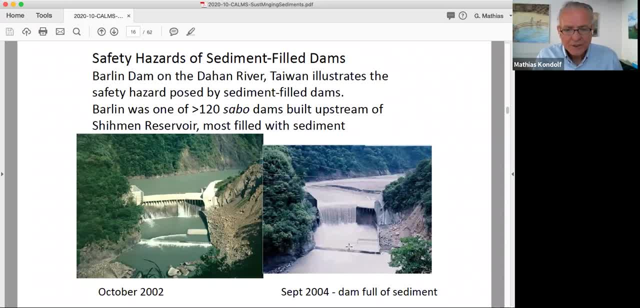 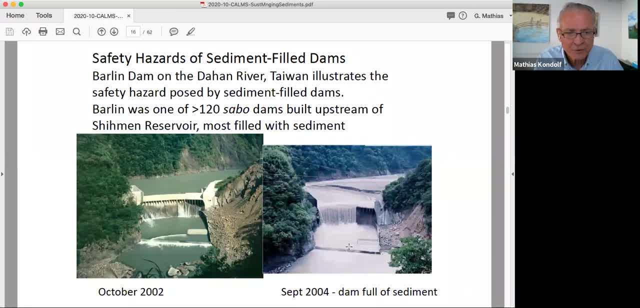 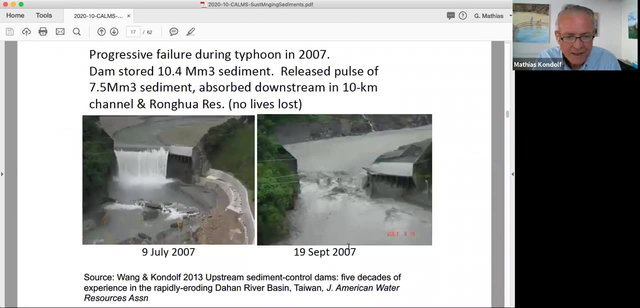 upstream to capture sediment before it would get to the reservoir, and this borrow the name one of these wars an original capacity of 10 million cubitors. it was built in the 1980. by september 2004 it was full, isn't it? in july 2007, you see, it's full of. 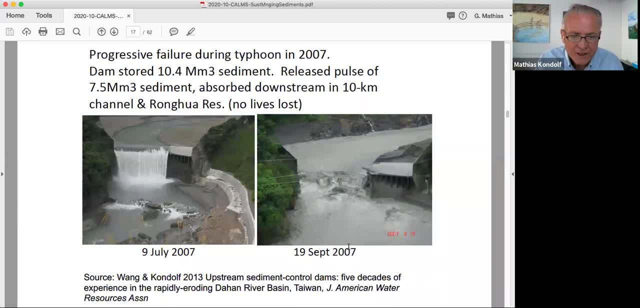 sediment, and there was a typhoon in september of that year which caused the dam to fail. so within a few hours it released most of that- 10 million cubic meters of sediment, so about three quarters of it. and what happened? there's a 10 kilometer reach before. 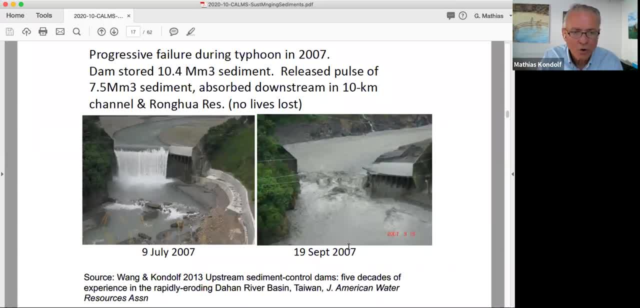 you hit the next uh dam like this called rongwa reservoir, and the sediment uh settled out in that reach and in rongwa reservoir and basically filled up rongwa reservoir. we used to joke that this is the wrong way to uh to manage sediment in a river like this. uh, this idea that you would 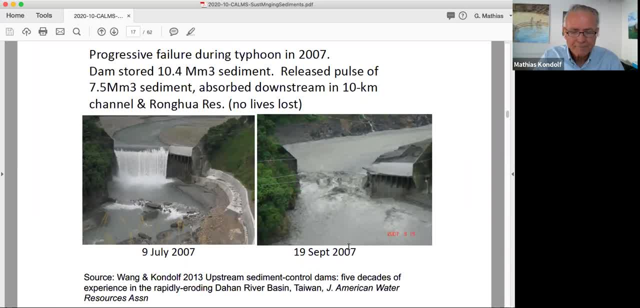 build a bunch of small dams to trap sediment, um, and then just leave them there and uh and not, and not creating just a whole bunch of new problems across the landscape that you're going to have to somehow maintain or deal with. uh, anyway, this, this approach, has never really made much sense to me. 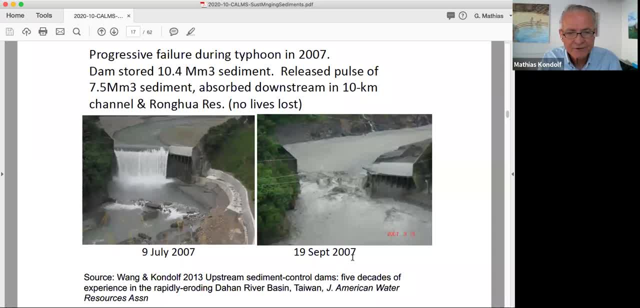 we're very lucky in this case that no one lives in that canyon. downstream there are just like a couple of road crossings, no one was killed, and the downstream channel and rongwa were able to absorb that sediment. so there was really, uh, no consequences of this except the fact that it was a 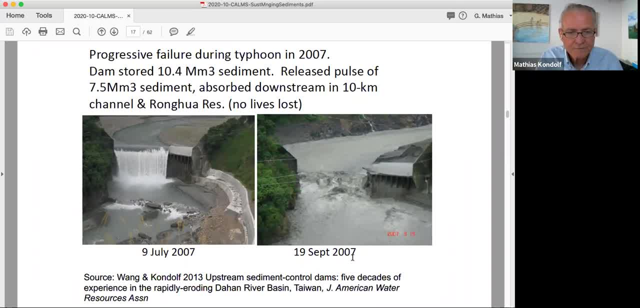 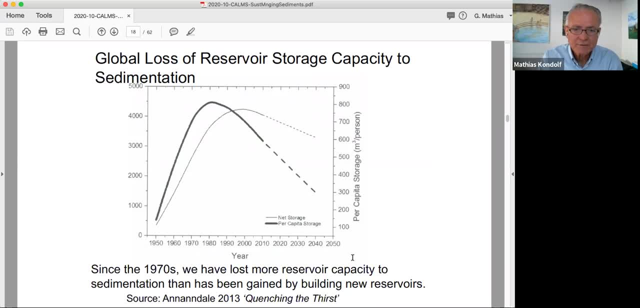 cause of life for this uh measure, so that was a little bit more interesting for the taiwan water resources agency. globally, we are losing a lot of reservoir capacity to sedimentation and even- i think even with the current dam building boom- although maybe, maybe we're going to be building- 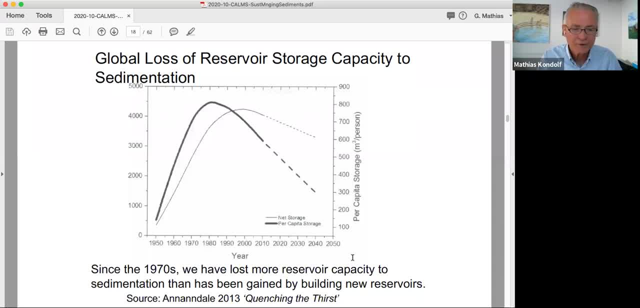 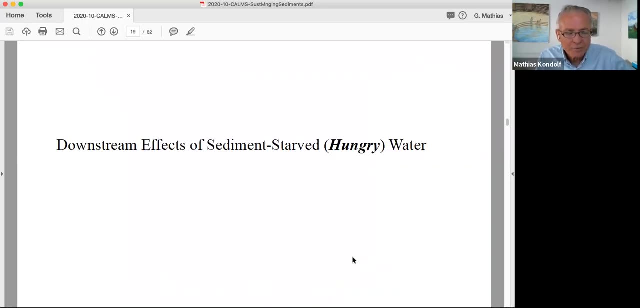 dams so quickly now that, uh, we'll actually start to compensate for this, but, uh, temporarily, but since sedimentation that has been gained by building new reservoirs. This is from George Annadale's book Quenching the Thirst. So it's a global problem, this loss of reservoir capacity. So 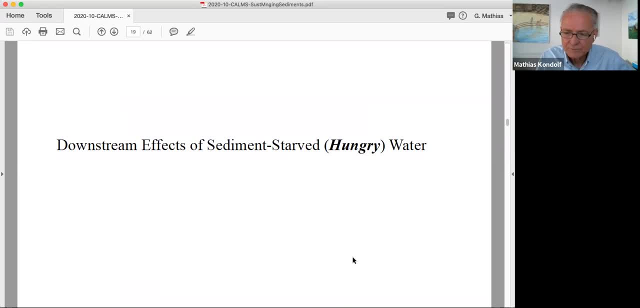 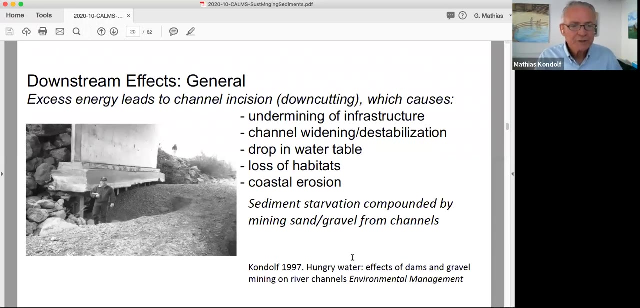 that should motivate some interest in sustainable strategies to manage sediment, which I'll get to later. But now I'd like to talk about the downstream effects of trapping the sediment in the reservoirs and releasing sediment-starved water. So, in general, when you release sediment-. 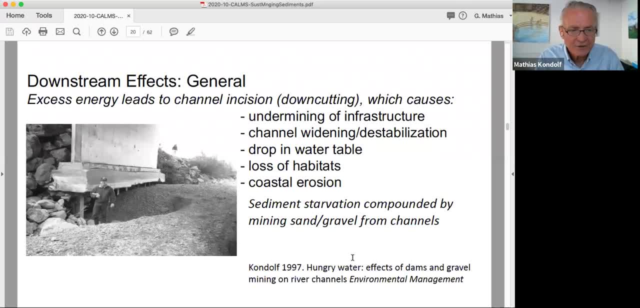 starved. flow from the dam, you have excess energy. that leads to channel incision and that will undermine infrastructure, cause channel widening and destabilization. drop in the alluvial water table adjacent, which has been a big problem in many places, including France. loss of habitats. 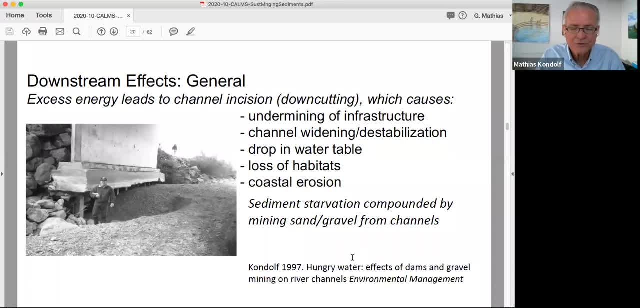 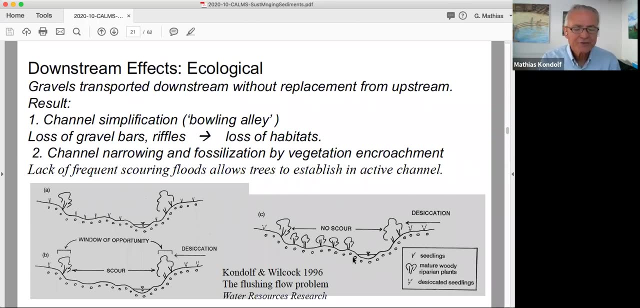 and ultimate coastal erosion because of the loss of sediment supply, And this sediment starvation is frequently compounded by mining of sand and gravel from river channels. There are many ecological effects as well, mostly channel simplification, because the gravel that creates gravel bars and riffles 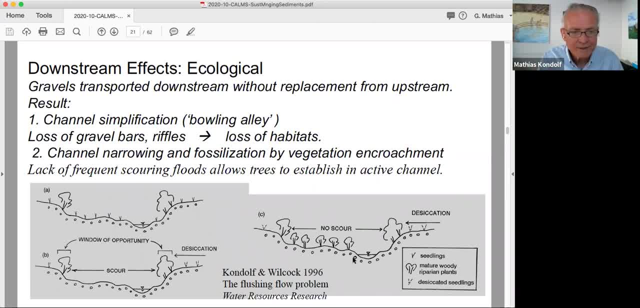 undulations in the bed that gets blown out downstream and you are left with a greatly simplified channel And you often see the channel narrowing and fossilizing by vegetation encroachment And where the dam is large, and it also reduces the frequency of scouring floods. 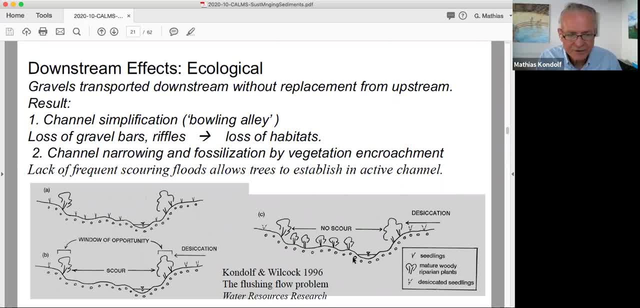 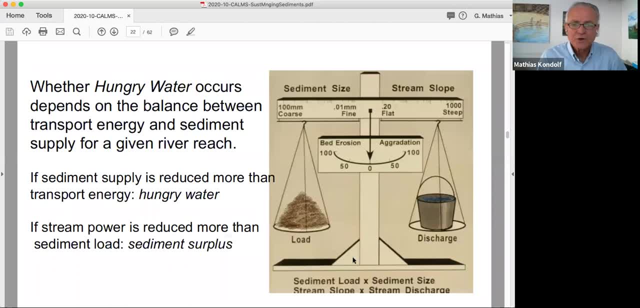 that could allow trees to establish in the active channel and you get this vegetation encroachment problem. Now you don't get hungry water, as we call it, sediment-starved hungry water below every dam. It depends on the balance between the transport energy and the sediment that's available for a given river reach. 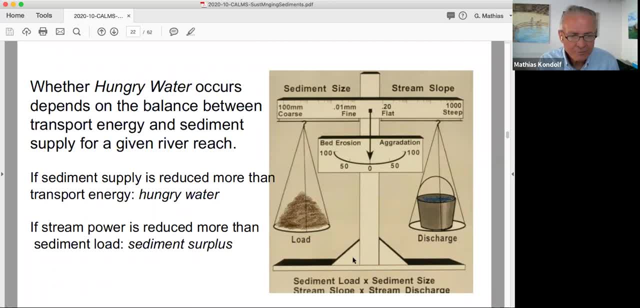 So if the sediment supply is reduced more than the transport energy, then you get hungry water. so there's more energy to move sediment than the sediment is still available. But on the other hand you can have a dam that's it's so big that it cuts off the floods. 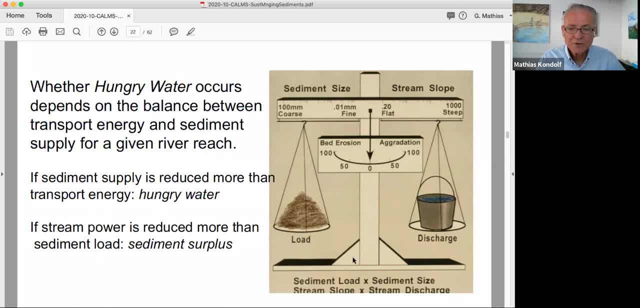 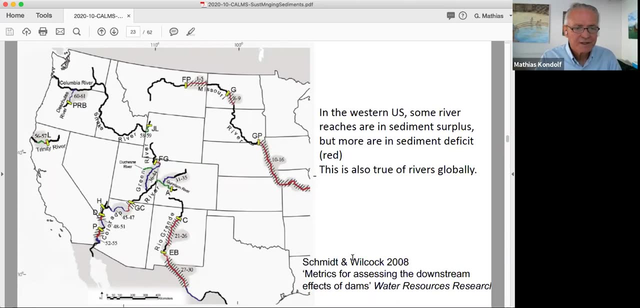 cuts off the high flows and maybe you have a big tributary downstream that's delivering sediment to sediment and the river's no longer to move that. So these would be a case where you have sediment surplus below the dam. Jack Schmidt and Peter Wilcock did an analysis of a number of major 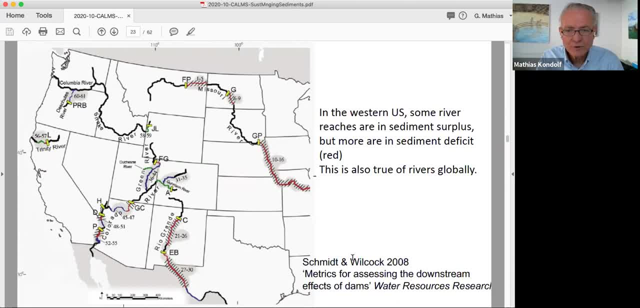 rivers in the western US to identify reaches that were in sediment surplus and some in sediment deficit. The ones in red are sediment deficit and I'll draw your attention to this reach right here. This is Glen Canyon Dam and this is the beach downstream in sediment deficit, down to the. 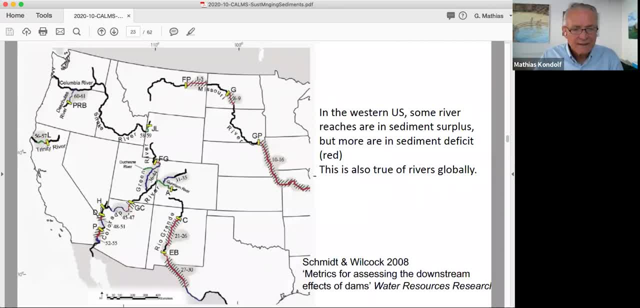 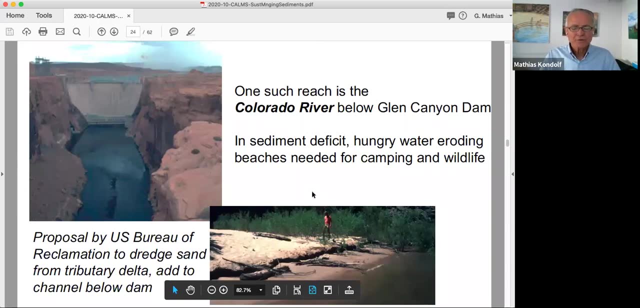 confluence of the Little Colorado And, by the way, mostly we are seeing reaches in sediment deficit. That's certainly true of rivers globally, But this reach below Glen Canyon Dam is interesting because in the Colorado River that goes through Marble and Grand Canyon, you have 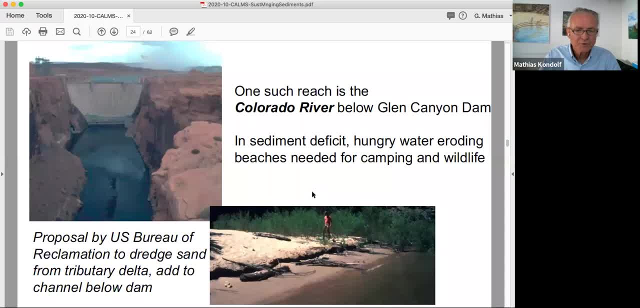 these sandbars that are essential for the river rafting trips. I mean, there are species that depend on these as well, but the main species really is Homo sapiens- for having a place to pitch the tent and camp during these raft trips. And these beaches have been eroding, So there's now a very complicated 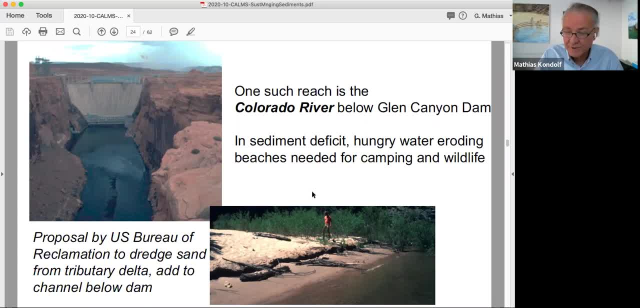 kind of system. It's really interesting. There was a record of a decision in the EIS and everything based on one interpretation of the science And that was later revised based on further information. The science, the conceptual model was changed. But now the way they manage it is when they have a high flow from the Perea River, bringing 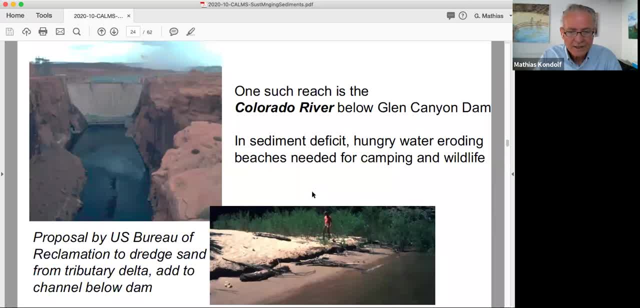 in sediment. then they make a release from Glen Canyon to suspend that sediment so that it will go out onto the sandbars and deposit on the sandbars, But as a way of actually increasing the amount of sediment available, not simply manipulating what's going on. it's a way of 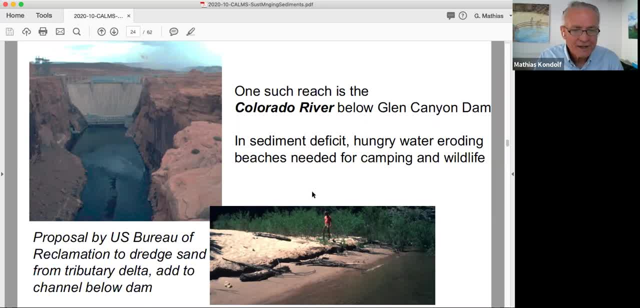 reducing the amount of sediment that's there. The Bureau of Reclamation developed a proposal to dredge sand from a tributary delta a few kilometers upstream of the dam, pipe it through a slurry pipe and then dump it into the river downstream of the dam. To build that would cost about 23 million to 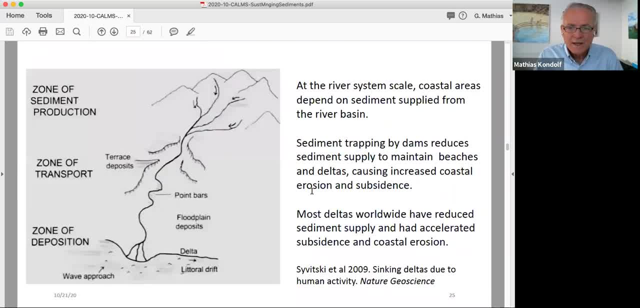 operate it each year would cost between two and three million. So, thinking at the river system scale, we have our coastal areas that are dependent on sediment supplied from the river. basin. Dams, of course, reduce this. Sand and gravel mining in rivers is also a big cause of sediment. 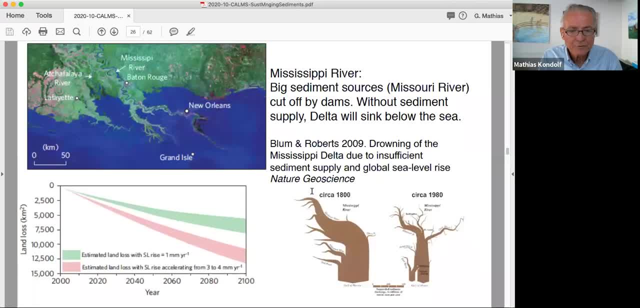 deficit. And, again, most of the rivers worldwide have had a reduction in their sediment loads. The Mississippi is a pretty good example of this. When you look at what the sediment loads were like, you know, let's say, a couple hundred years ago, And then today the Missouri. 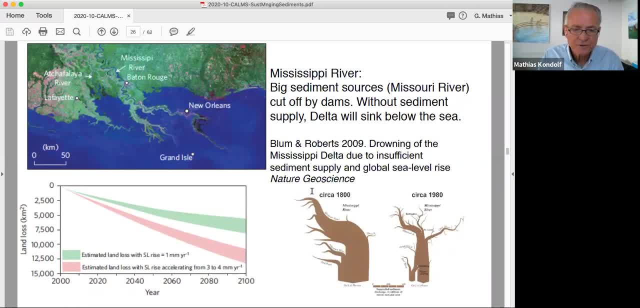 Missouri was of course the biggest sediment source to the Mississippi River system And with the series of dams on the Missouri that's been basically cut off. So when we look at the future of the Mississippi Delta it's not very encouraging. We can, you know, there are a lot of. 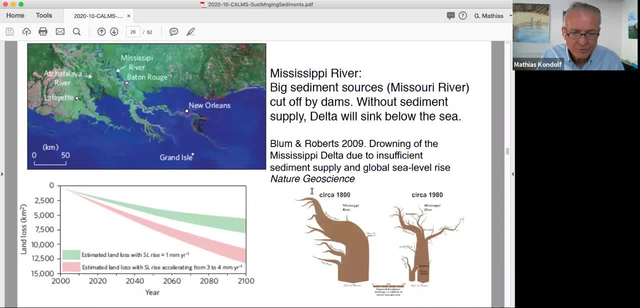 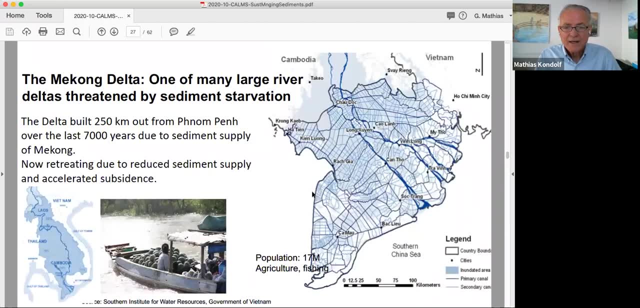 things we can do and we can have the sediment diversions and whatnot, But the amount of sediment coming into the Delta is way less than it was originally. I've worked quite a bit on the Mekong Delta, which is a really interesting place for a number of 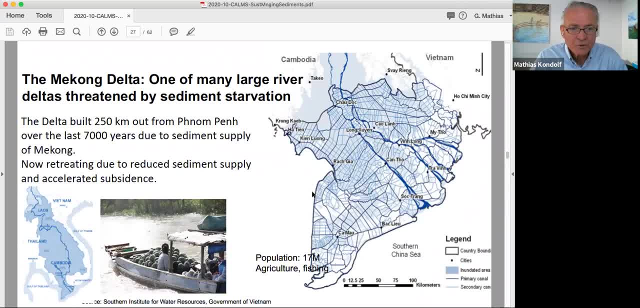 reasons, But it's one of the big river deltas in the world that is threatened by sediment starvation. 7,000 years ago, the coast was at Phnom Penh in Cambodia, And over the last 7,000 years the Delta has prograded to its current form because of the very healthy sediment supply. 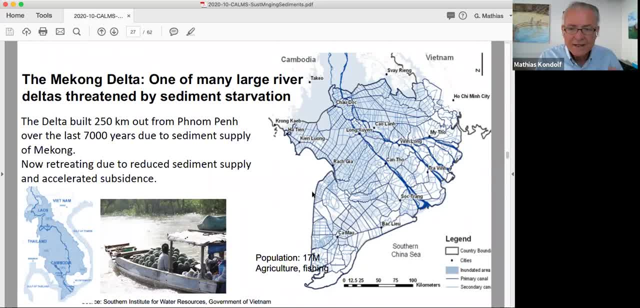 from the Mekong River, Now the Delta. for the last 10 or 20 years it has started retreating because of the reduction in sediment supply. Mostly the immediate cause of reduction is extensive mining of sand from all the channels of the Delta and the main river upstream coming into the Delta. 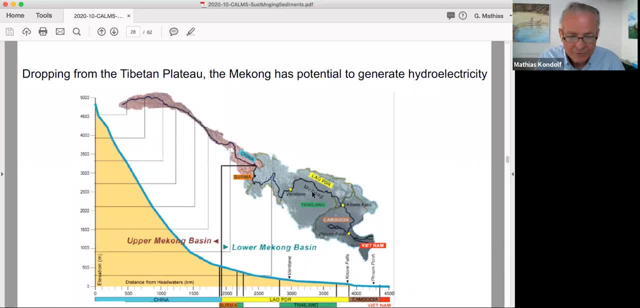 But the long-term problem will be dams, which will reduce sediment even getting down towards the Delta. The Mekong drops from the Tibetan Plateau, so it's got tremendous drop, tremendous head, and it's got a lot of flow as well. So it's got all the ingredients you need. 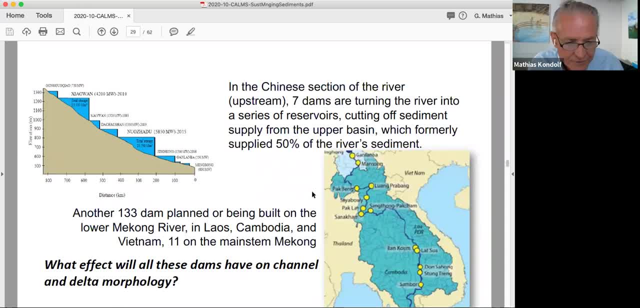 for hydropower And this has not gone unnoticed. It's fascinating just to see all the grand schemes for building out the hydropower potential in the Mekong: Ben Madrid, Joseph MusH, principle, Kelvin Mo masks, Maoro fighting Dao. Last night's talk about the Mekong hangar is part of 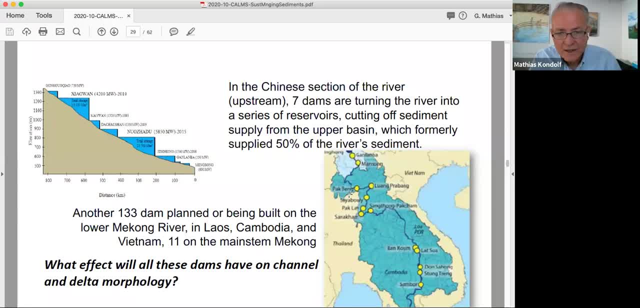 serum, And then, as you get into the Tibetan Plateau, there are tons more that are under construction And whole group of big dams are under constructionyou m ительно Texas. The Chinese have already done a lot. They've built 7 big dams on the main stem and there are dozens more. under construction on tributaries. This is in this lower reach of the mainstream, And then and then Father up as you get into the Tibetan Plateau, there are tons more that are under construction: This other part of the Mekong in China. 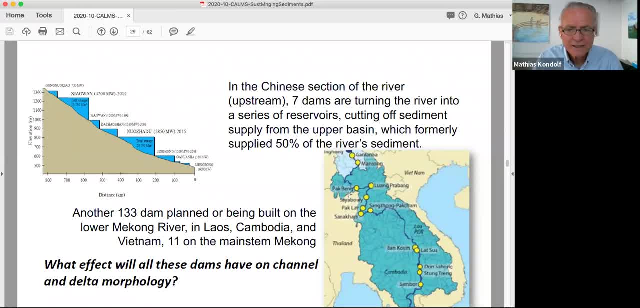 the river sediment. So we used to have something like 160 million tons per year, on average 140 to 160 million, which is based on some of the earliest measurements that we have, going back to the 70s, 60s and 70s, but also the long term rates of sediment accumulation in the delta and offshore. 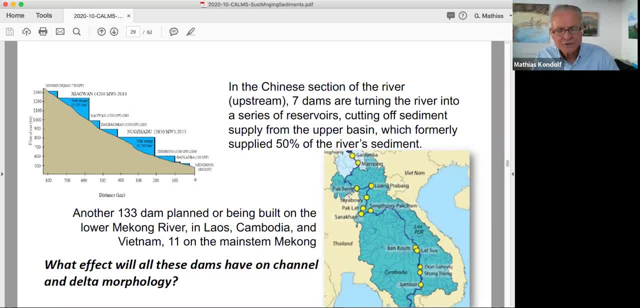 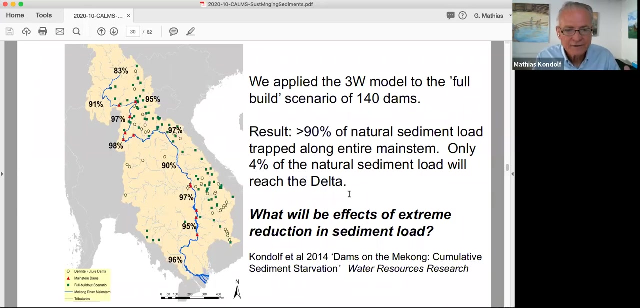 So, as we, as we see, these Chinese dams have gone in, and then in the lower basin, So that would be Laos, Thailand, Cambodia and Vietnam. We have more dams planned, a lot more dams planned, And we asked the question of all these dams were going to be built as originally planned? what would be the effect on the sediment delivery to the delta? 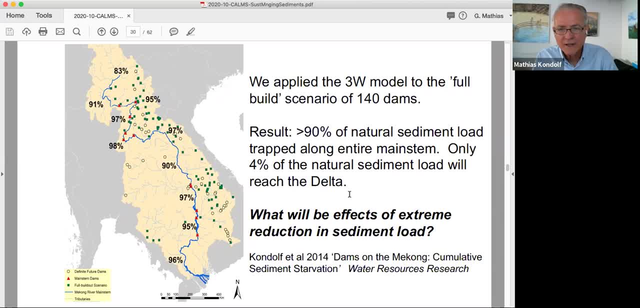 So we adapted our 3W model From California to the Mekong, which required quite a bit of adaptation because we didn't have existing reservoir sedimentation rates to to, to extrapolate. So we did it mostly based on geology and the few data that did exist, mostly measurements of set of transport. 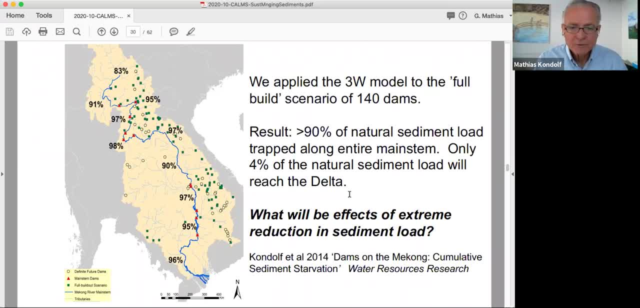 We found that well over 90% of the natural sediment load would be trapped along most of the main stem And by the time you get to the delta, there would be only about 4% of the natural sediment load that will reach the delta. 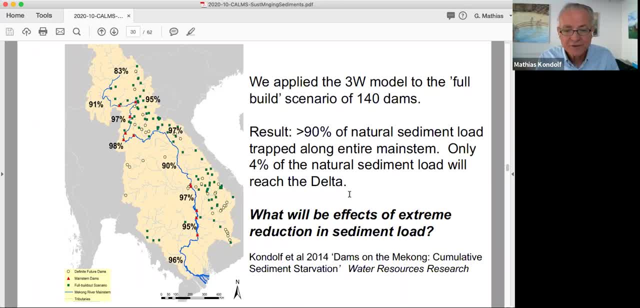 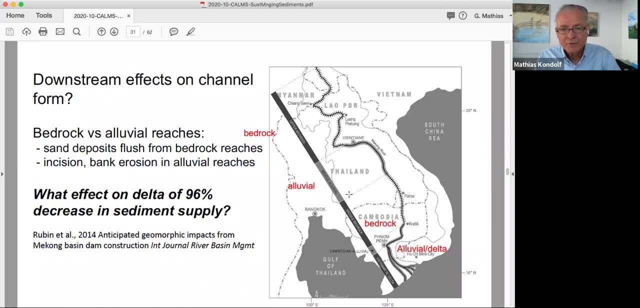 So of course you can ask, you know, what would be the effects of this extreme reduction in sediment load? And looking all along the river, we have an alternation of bedrock and alluvial reaches, but much of the river is bedrock. 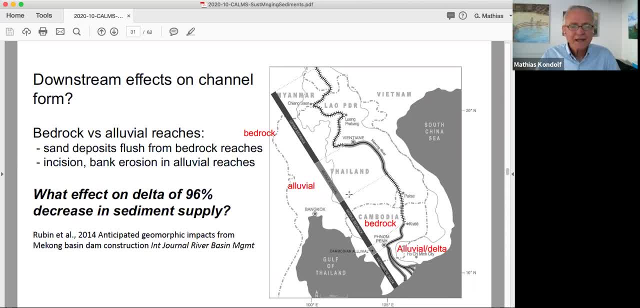 You know, there there are deposits of sand that you see, and when you look from, When you look at aerial imagery, you see a lot of sand, but when you're in the field you see that bedrock. There's a lot of sand. 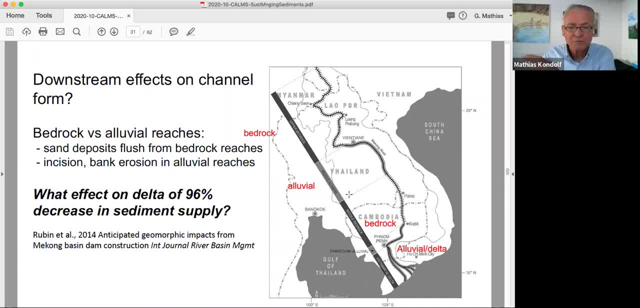 And when you look from, when you look at aerial imagery, you see a lot of sand, But when you're in the field, You see that bedrock. You see that bedrock. most of this is maybe two meters thick and it's not going to take long for that to get flushed out. 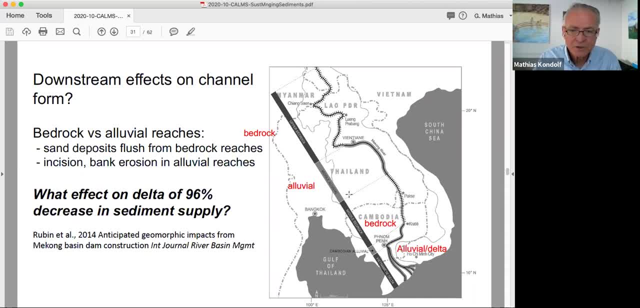 And so we will have, for example, the alluvial reach from Vientiane down to Savannakhet. That will certainly incise, but the bedrock reaches above and below. there's not that much sediment you can get out of those. So there'll be a pretty massive incision on the alluvial reaches. 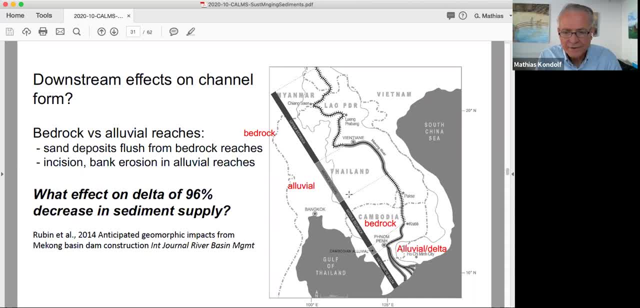 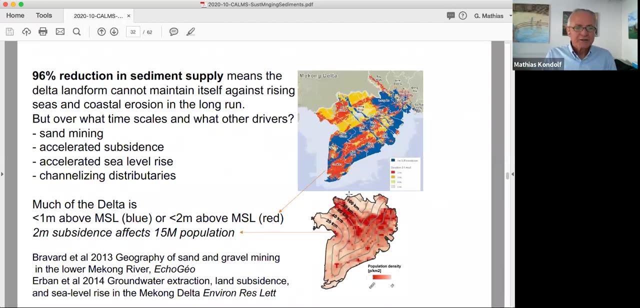 and getting down into the delta, And the delta itself will simply not have the sediment supply that's needed to balance natural subsidence and coastal erosion. And then on top of that, we have more problems, which I'll mention here. So this delta landform, like any delta, it can't. 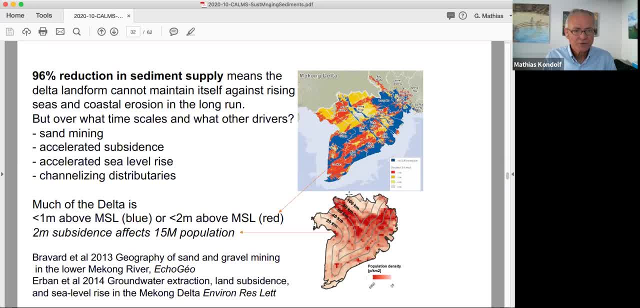 then maintain itself against the rising sea levels and coastal erosion of the long run. But there are other drivers, including much sand, which I mentioned. The subsidence has been accelerated by pumping of groundwater And then of course there's globally accelerated sea level rise And whatever sediment reaches the delta now 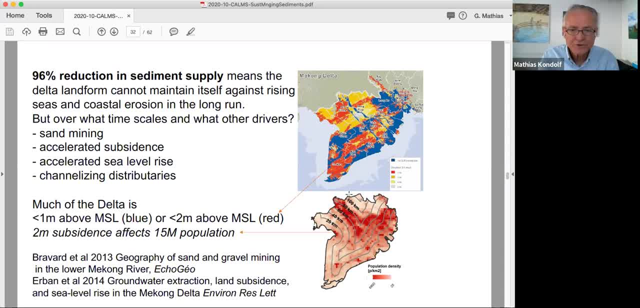 is increasingly shot out to the sea because the distributaries have been channelized and diked, So there's no way for the sediment to even get out onto the delta plane and deposit where, as it should be doing. The delta is virtually all less than two meters above sea level. 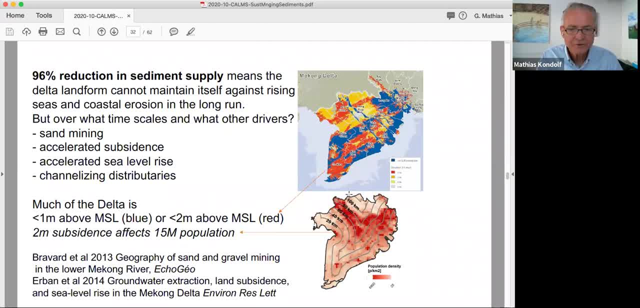 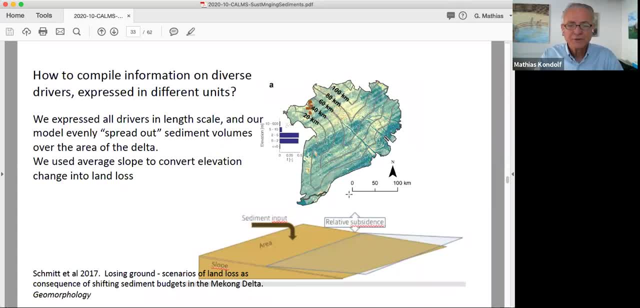 And when we project this into the future, we see that by 2100, about 90% of the delta will be underwater if business as usual continues: pumping the groundwater, mining the sand, building the dams as they are being built today, which is without any sediment management. 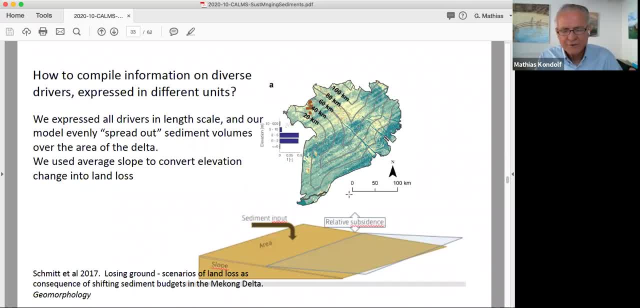 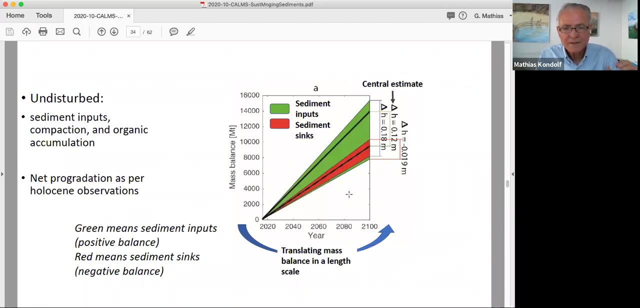 So we did this by combining different kinds of data- vertical subsidence data- with volumes of sediment Coming into the delta, and converting those all with this what we call the delta plane model. So not to belabor this, but when we apply the model using historical rates of natural sediment. 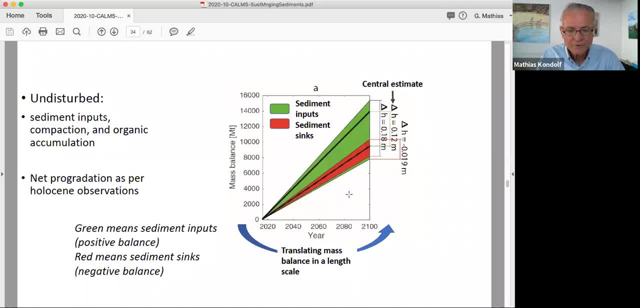 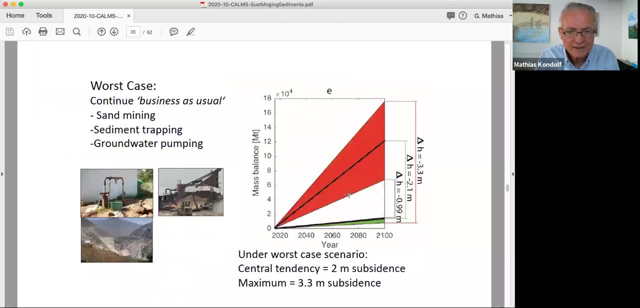 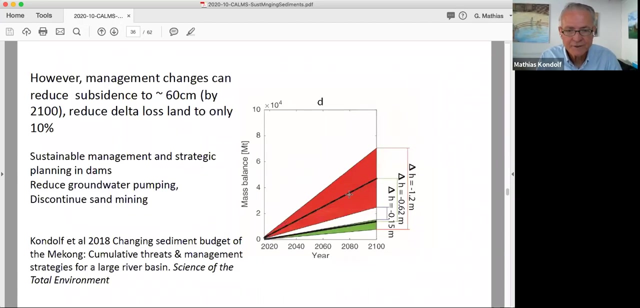 supply, we were able to replicate the kind of aggregation that we have seen over the last thousands of years. But when we run the model into the future with the current business as usual practices, we see this massive subsidence that will continue And, given the topography of the delta, that means that by 2100, 90% will be underwater. 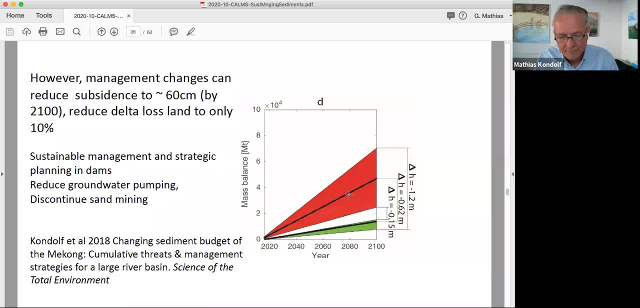 It would be possible to slow this down. if we were to stop this crazy pumping of groundwater, if we were to stop the mining of sand from the channels and if we were to build the future dams to pass sediment, we could, slowly, We could slow it down and prolong the life of the Delta. 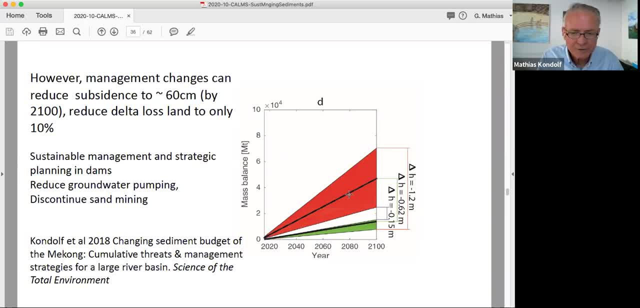 The Delta has a population, depending on where you draw the line, of 17 to 20 million people. It produces 95% of the rice that is exported by Vietnam, And that translates to something like between 2% and 4% of the global protein that's traded around the world. 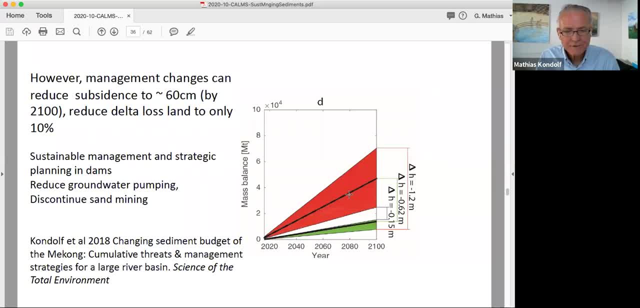 It's an incredibly important place And when you look at the official Mekong Delta plan, which was done with the Dutch and the Vietnamese, or the World Bank documents, they all just sort of assume the Delta is going to be there forever. 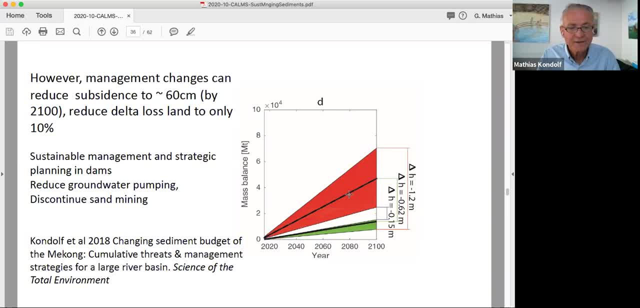 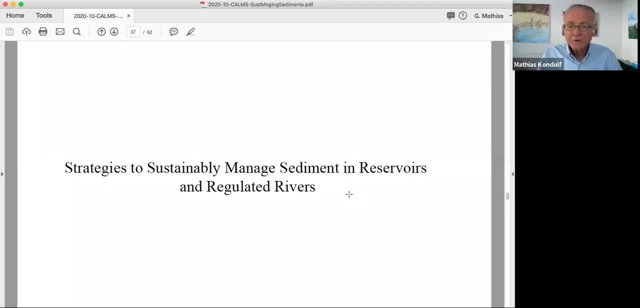 And we've been trying to argue. well, no, in fact, that's not to be taken for granted. A lot of these wonderful projects that are being done could be viewed as rearranging deck chairs on the Titanic, Because the very existence of the Delta is questionable. 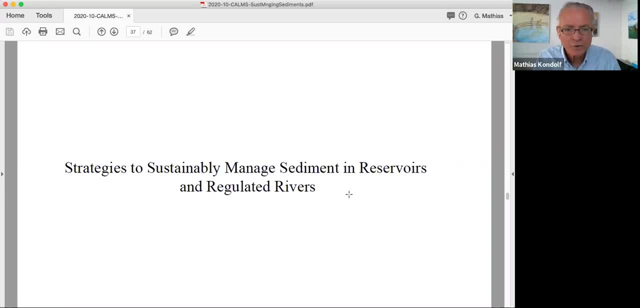 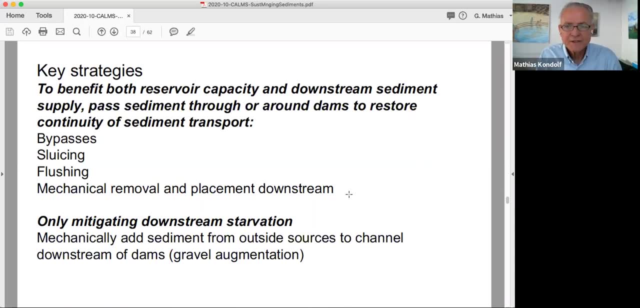 So what are some strategies to sustainably manage sediment in reservoirs and regulated rivers? So the real idea: if you want to both maintain reservoir capacity and compensate for downstream sediment supply, you try to pass sediment through or around dams to restore this continuity of sediment transport. 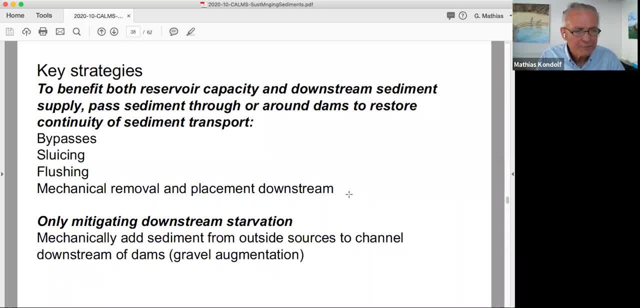 And you can do that with bypasses, by sluicing the sediment Or routing the sediment through the reservoir, flushing sediment that's been deposited in the reservoir, or mechanically removing it and placing it in the downstream channel. This latter option is done in Japan and some places in Europe. 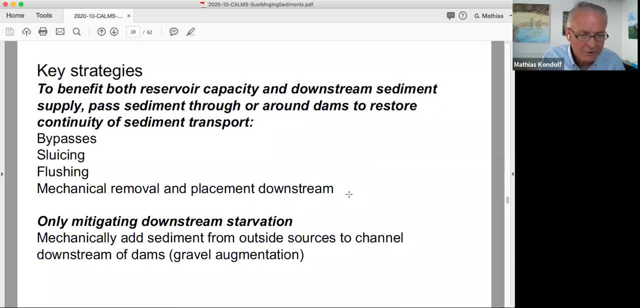 There are only two examples I know of in California where this has been done And because of the impacts on habitat downstream. there are a number of reasons: projects to mechanically add sediment to the channel below the dam, but usually it's easier to get that sediment from someplace else than the reservoir itself. so you are kind of dealing. 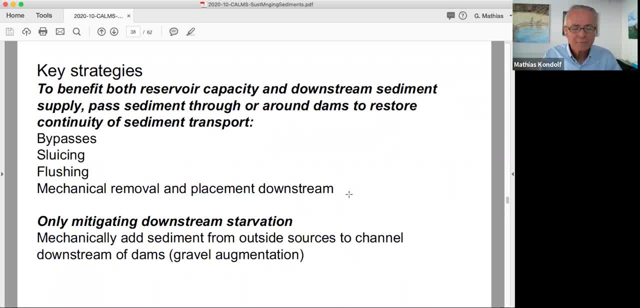 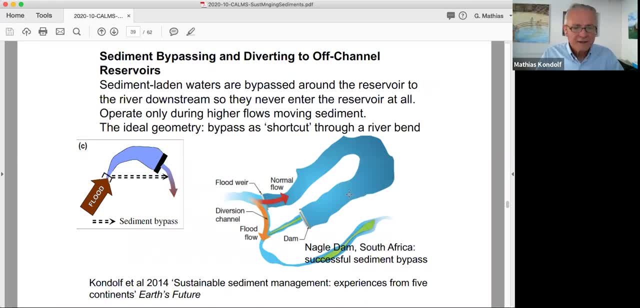 at least partially, with this downstream sediment starvation problem, but you're not helping prolong the life of the of the reservoir. so looking at some diagrams of these approaches, sediment bypassing where it works is a wonderful solution. this is nagel dam in south africa where the reservoir, the river, takes this big bend. the dam is here, so the reservoir is on the bend. 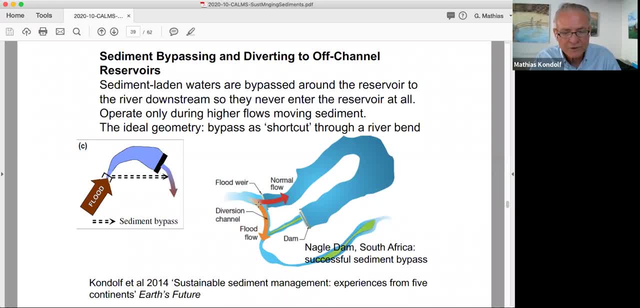 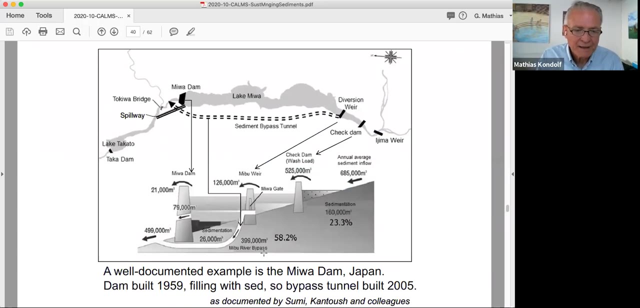 they simply cut a channel through this ridge which, through which they divert the sediment laden flood flows, and so those sediment laden flood flows rejoin the river below the dam, and so the continuity of sediment through the system is maintained and the reservoir is not filled with sediment. that's the perfect geometry to have a bend like that. 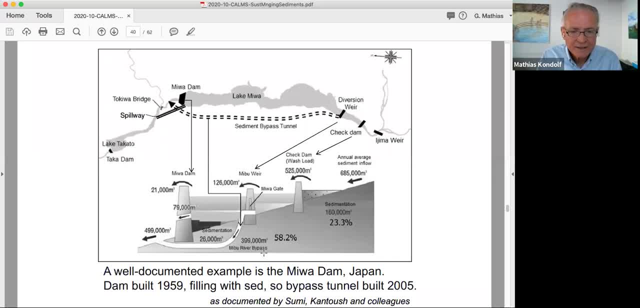 but even when you don't have that, you can still make it work with the right engineering. this is a bypass tunnel designed by tetsuya sumi and and his colleagues on the miwa dam in japan, and and this miwa dam was built in 1959, but it was filling with sediment. 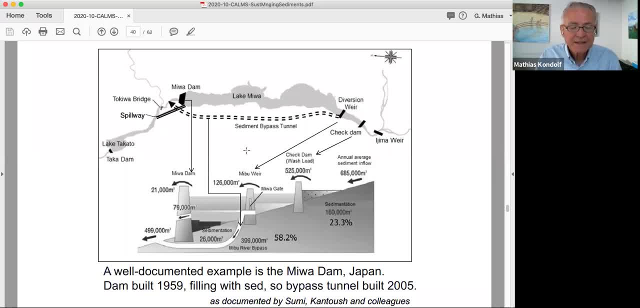 so fast that they built the bypass tunnel in 2005.. i mean, it's a shame they didn't build a bypass tunnel right off the bat, then they would have maintained their capacity the whole time. but but now they're able to maintain about half of the capacity by by using this bypass. so so the 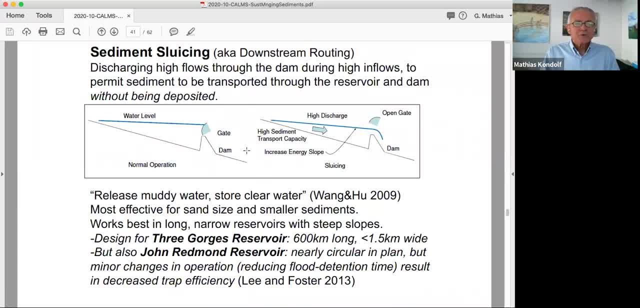 dam still functions. sediment sluicing refers to moving the sediment not around the dam but through the dam, and you basically draw the reservoir down so that the river flows in and through the reservoir, essentially as a river, and this requires large low-level outlets in the dam so that you can release the water fast enough for this to happen. 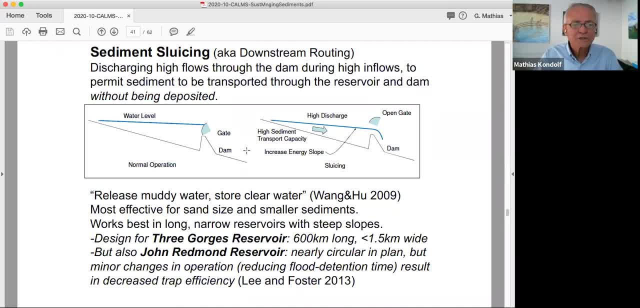 and this is following the, the chinese velocity release muddy water store clear water. of course it's most effective for sand size and smaller sediments that can be suspended through turbulence. it also works best in long, narrow reservoirs, usually small ones but with steep side slopes. but an exception to the small rule is three gorges dam, which is a very big reservoir, but it is very 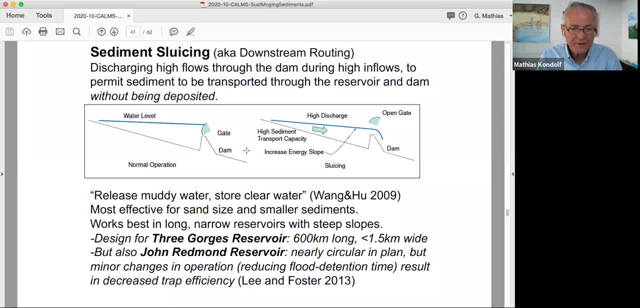 long, narrow and has steep slopes, and that's. that's basically the strategy that is intended to keep the three gorges from filling up with sediment over time. um, but you can even do some sediment routing through, sediment through or with a completely different geometry, like John Redmond reservoir in Kansas. 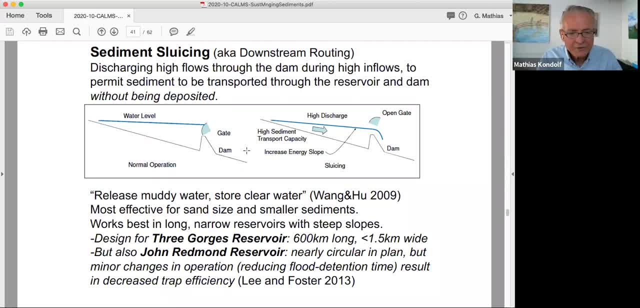 It's essentially circular in plan, but minor changes in the operation- simply reducing the flood detention time- have resulted in decreased trap efficiency. So prolonging the reservoir Here you're talking about like improvements of like one or 2%, but it's still something. 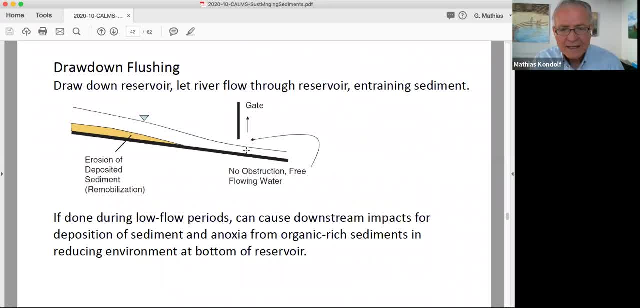 it's still worth a lot of money. if you cost it out, Then some of the sediment that's settled out already. it's still possible to flush that through the system And that's usually requires drawing the reservoir down And then often you have to get out there. 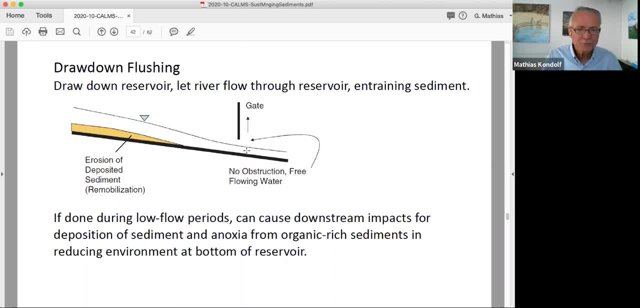 with heavy equipment to loosen up the sediment which has set in place over time. There are a lot of issues with flushing. One thing: it's been done often during low flow periods during the summer And there been a lot of controversy of PG&E. 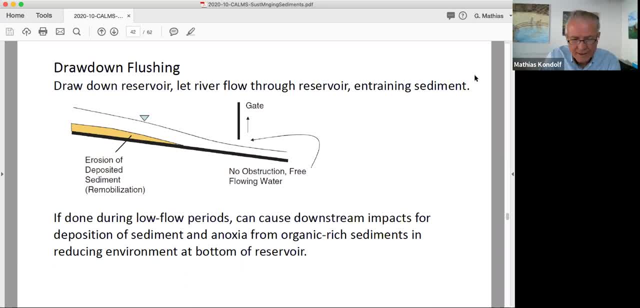 doing this And some of their hydroelectric dams And a lot of the sediment often will. from the bottom it will have a lot of organic material, So it be anoxic and this anoxia can kill everything for a couple of kilometers downstream. 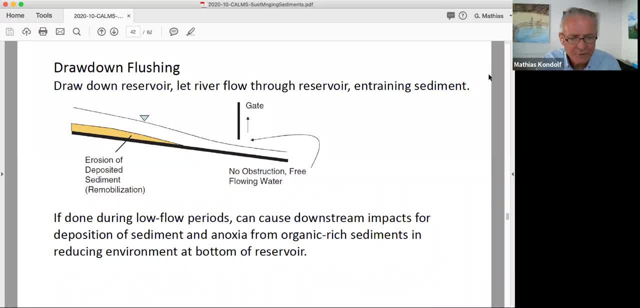 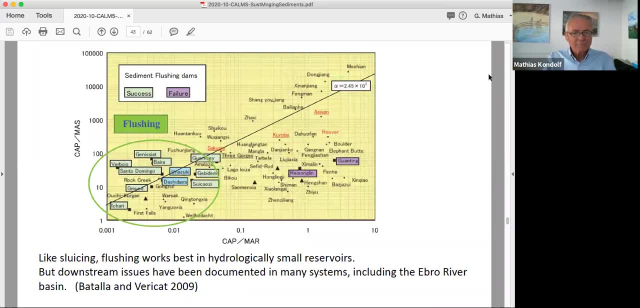 So flushing has gotten a bad rap because of this. but if it's done at the right time of year at high flow, it's not necessarily so bad. And like sluicing, flushing works best in hydrologically small reservoirs. This is a plot by Tetsuya Sumi. 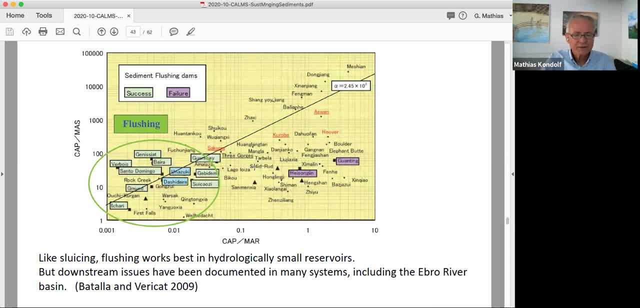 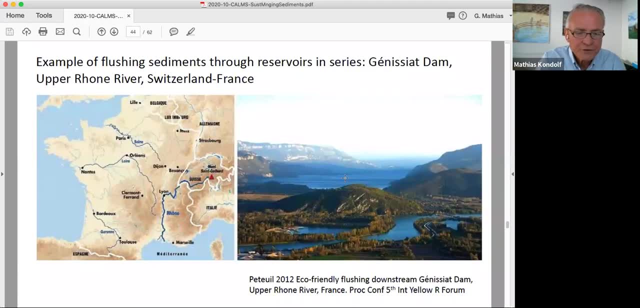 but the issues have been documented with many systems, including the Ebro basin On the Rhone river, going from Switzerland to France. the sluicing, or flushing rather, has been done to get rid of the accumulated sediments, And this is largely motivated. 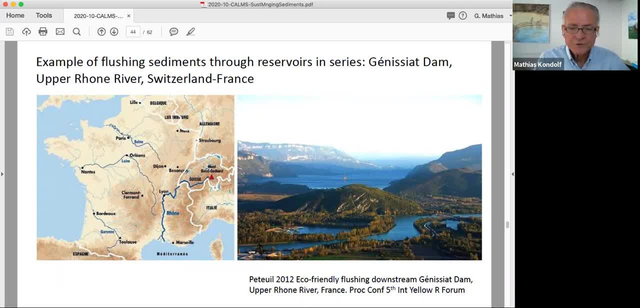 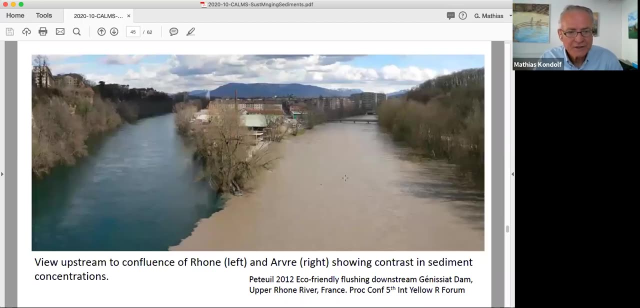 Because the Jeunesseat dam, which is in Switzerland, just above the French border, if that fills up with too much sediment, it creates backwater that floods Geneva at the downstream end of Lake Geneva. So, and here you see, this is the Rhone. 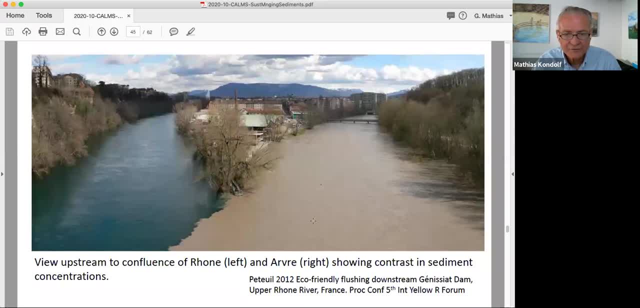 coming out of Lake Geneva and this is the Aue coming down from Mont Blanc, And so this is glacial meltwater with tons of sediment, And that's really where the sediment that accumulates- It's in the Jeunesseat dam- comes from. 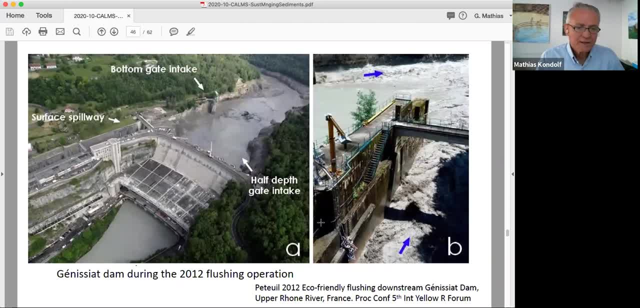 So they flush this every few years. This was from the 2012 flushing operation And you can see the accumulation of all this fine rain sediment in the dam, upstream of the dam, And then they're releasing it through here. Now this is. you know, unlike some parts of the world, 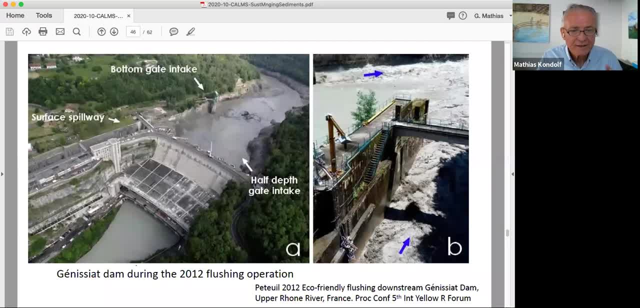 this is a place with a lot of attention, a lot of scrutiny And so, as a result, the Compagnie Nationale du Rhone, which operates the French dams just downstream. they basically put everybody into action, Even the. you know the person that answers the phone. 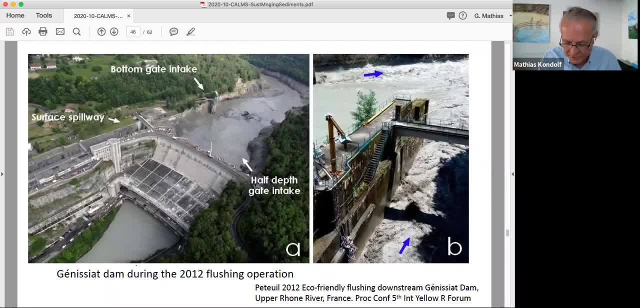 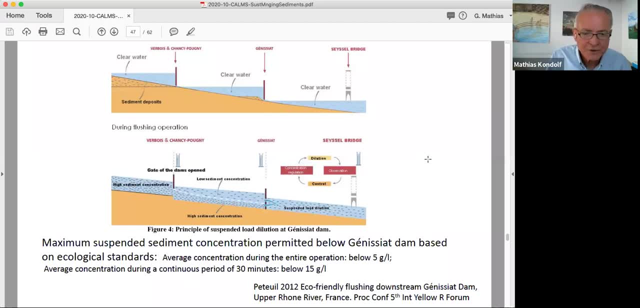 and sorts the mail, they all. they're all pressed into service to go out and monitor different parts of the system, And similarly on the Swiss side, And basically they're allowed a certain concentration of sediment that they can do, And so they have to play around with the. 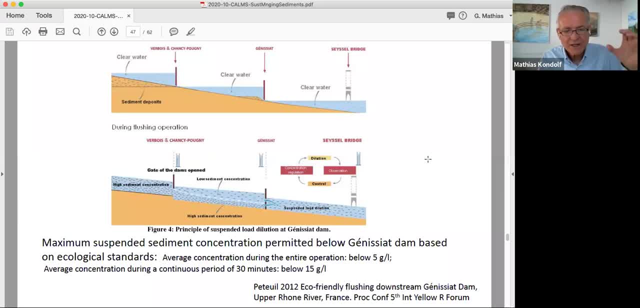 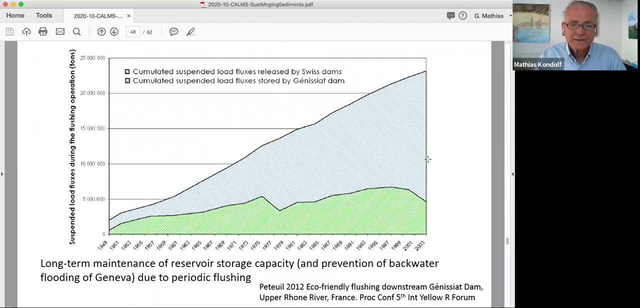 with releasing water from the bottom outlets, which would have a lot of sediment against water, that they're released from the top outlets, which are basically sediment free, so that they can maintain the sediment concentrations below the requirements. And this, this has worked. the system has worked. 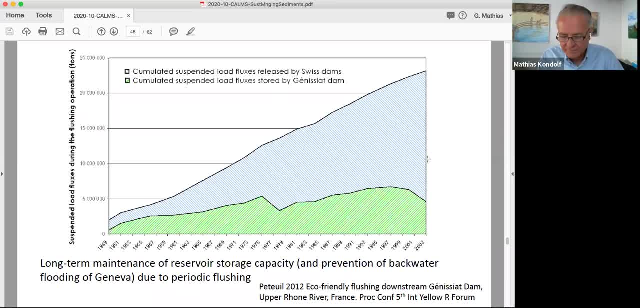 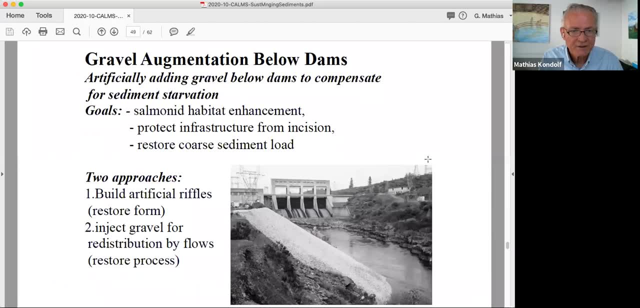 It's over time. it has prevented, you know, the, the, the, the bed from aggregating too much in Genesee at them, and has prevented flooding in Geneva. Now I won't talk too much about this, but I think it is kind of interesting. 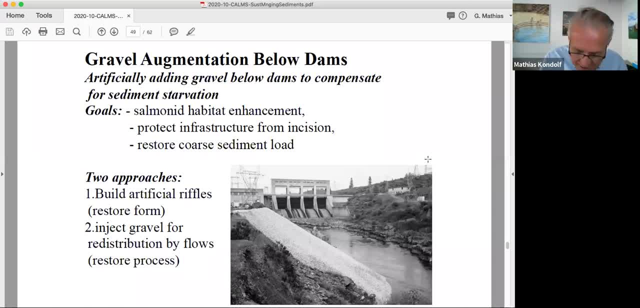 This is not as interesting to the lake manager but but for me, a river guy, I'm fascinated with how the changes in the sediment load have affected habitats and channel geomorphology, And and so there were a lot of projects to you know. 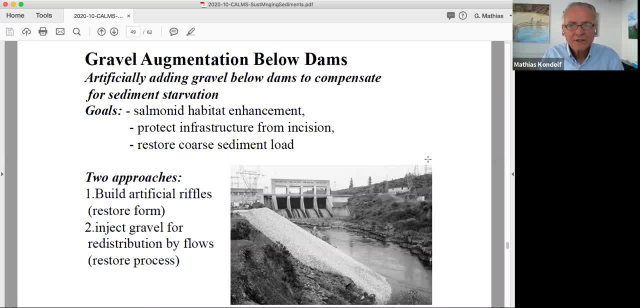 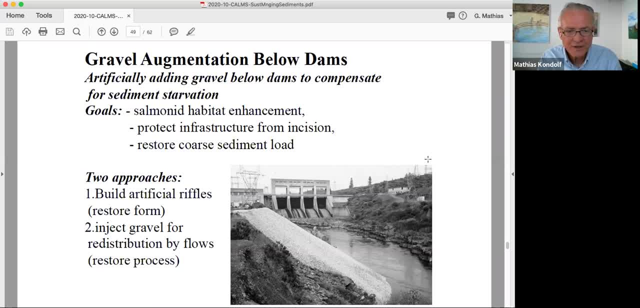 And most of the projects have been done to restore fish habitat. Originally, these were usually building artificial riffles where they would go in and try to create a form that they wanted, But of course you know, rivers being rivers, those things usually wash out at some point. 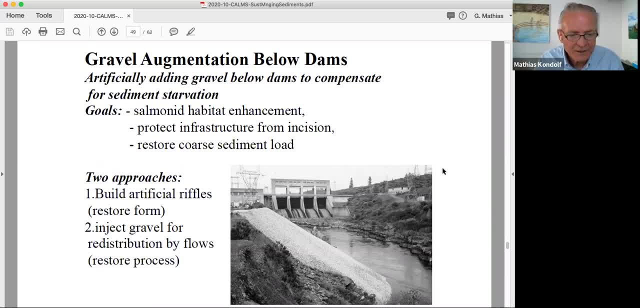 everyone gets upset, So more and more the approaches, as illustrated here, to inject gravel for redistribution by flows. This is a Keswick dam, the re-regulating reservoir below Shasta, And here you've had dump trucks have been dumping this tongue of sediment into the river. All right. so in Northern California we have added gravel below many dams- well over 500,000 cubic meters of gravel Gravel added and it's going up all the time, And the biggest projects in the Sacramento River, Clear Creek, Middle American and Trinity. 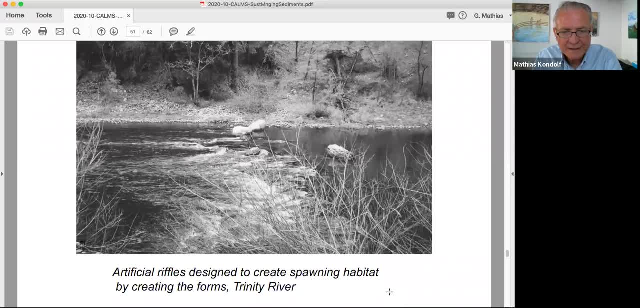 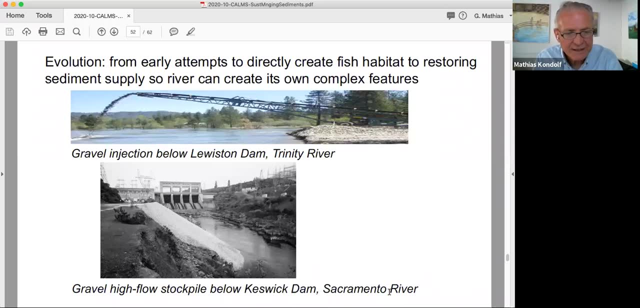 These are some of the early projects: artificial riffles designed to create directly spawning habitat, But again, these tend to wash out. So now we have more the injection either the kind of a stockpile that I showed you before there below Keswick. 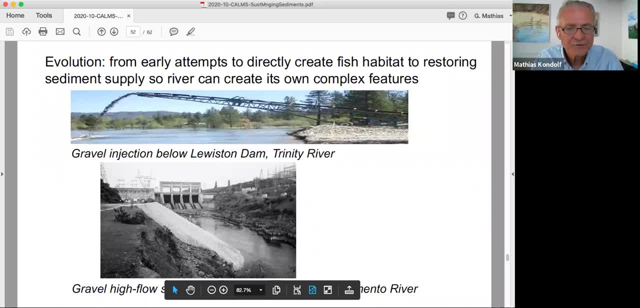 or during the high flows themselves. this is a conveyor belt that's dumping gravel into the Trinity River below Lewiston Dam. It's relatively easy to set this up because the high flow releases there, these are deliberate flushing flow releases that are made from the dam. 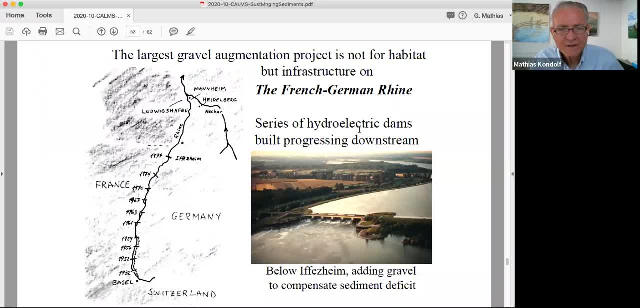 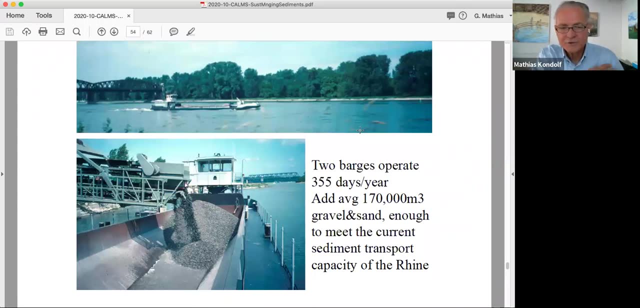 But the biggest gravel augmentation project that we have anywhere is not for habitat, for infrastructure, so it's kind of unusual. It's on the Rhine, below the barrage Ifesheim, and there they add gravel to compensate for the sediment deficit from the series of dams upstream. 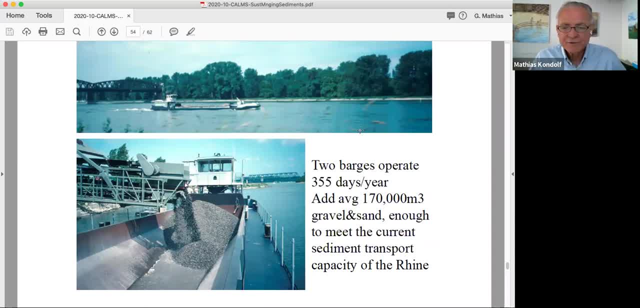 There are two barges that operate 355 days a year. On average, they add 170,000 cubic meters of gravel and sand, and that's enough to meet the current sediment transport capacity of the Rhine. The actual amount of sediment that they add: 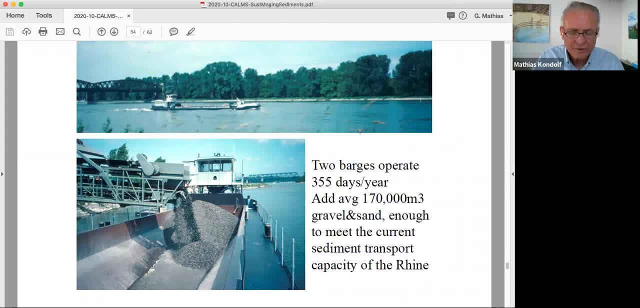 depends on the number of days over a certain threshold. I think it's a 1,250 cumec, something like that, But it's all. this is actually from the Treaty of Versailles. Germany was required to build these dams, hydroelectric dams, for the benefit of France. 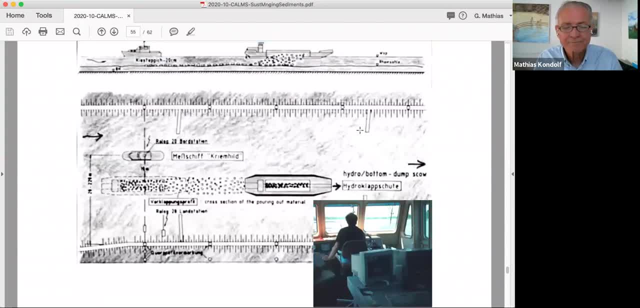 and this below this lower one. So this is now written into the treaty. the composition of the gravel and sand and so on is pretty fascinating. So here's a diagram of the barge dropping the gravel. It goes downstream when it comes abreast of this pilot boat. 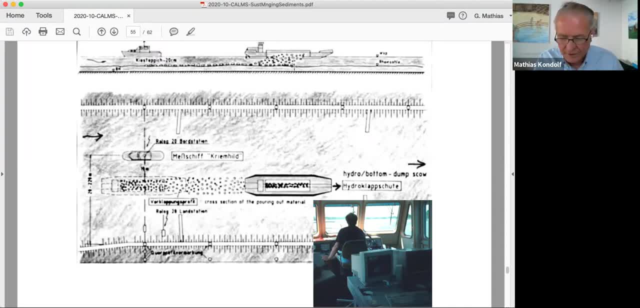 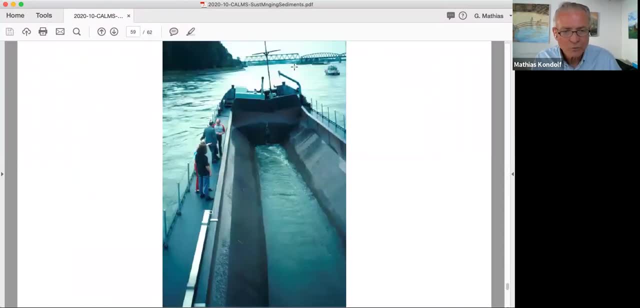 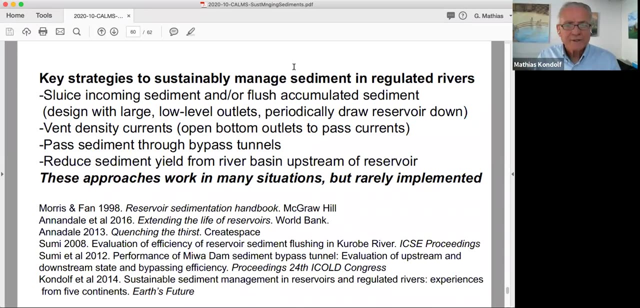 then the barge operator knows you should start opening up the barge and releasing the gravel, And that's what we see happening here. And whoosh, there goes the gravel, and then the barge turns around and goes and gets another load. Okay, so just recapping these strategies for sustainably managing sediment in regulated 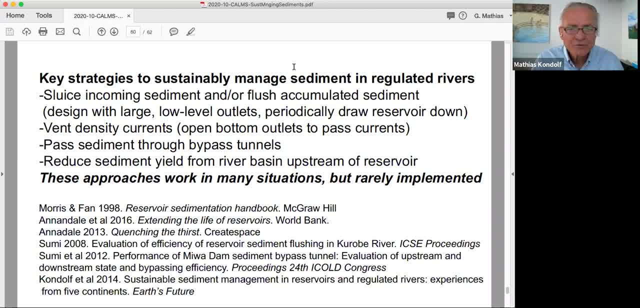 rivers If you can sluice the incoming sediment or flush the accumulated sediment, and this usually takes large low-level outlets and it requires that you periodically draw the reservoir down. I didn't include a slide in here mentioning that there's another kind of flushing, that 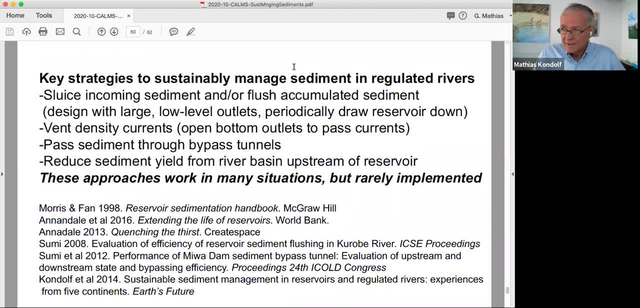 you can do, which is it's called turbidity current venting. So if you know a turbidity current is coming into your reservoir, you can open your large outlets in the dam and let that turbidity current pass through. And this is a phenomenon that happens more often than you might think. 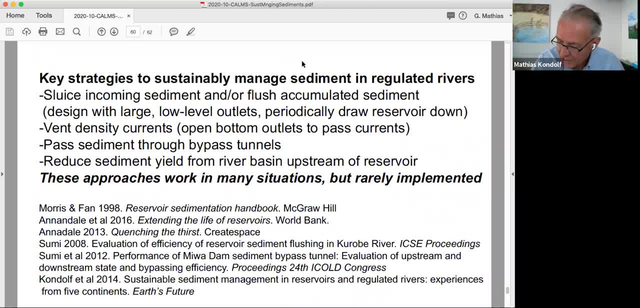 And the Chinese have really perfected this. in the Xiaomanxia Reservoir, the Yellow River, They get these turbidity currents frequently and they have worked it out where they are able to vent these and get rid of the majority of the incoming sediment they can pass downstream. 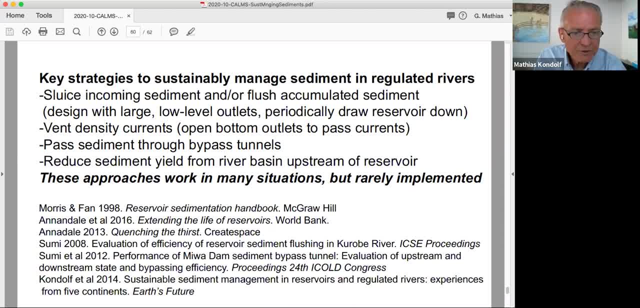 through that, And then you can pass sediment through bypass tunnels, as we saw the example in Miwa Dam and also in San Francisco, South Africa, And reduce the sediment yield from the river basin upstream of the reservoir. Okay, I didn't talk much about that because this is something that there are many other 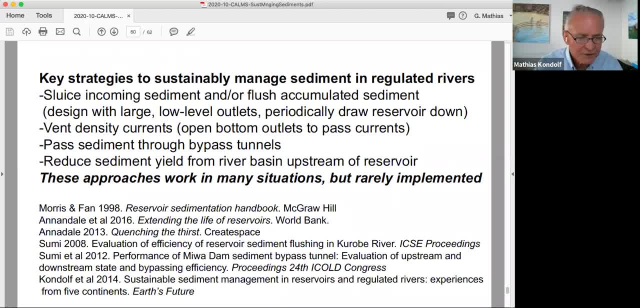 benefits from doing this. you know, if you have conservation of agricultural land, approaches like this to retain the soil fertility, there are a lot of benefits of that. But it's very difficult to get these approaches to pencil out For the river, The reservoir itself, for sustaining the capacity of the reservoir. 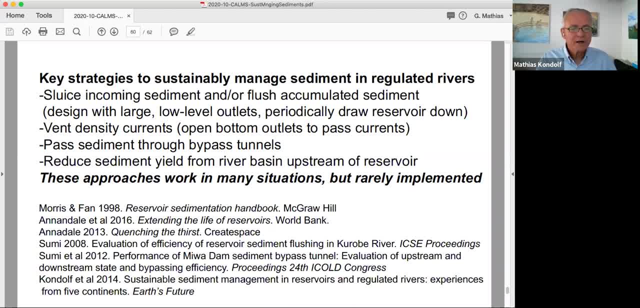 Now. so we have this toolbox of things that we can apply, but they are very rarely implemented, And I think the reason is really just the way dams are designed: the problem of the economics. I'm not going into that in this talk, but dams are usually designed based on the discount. 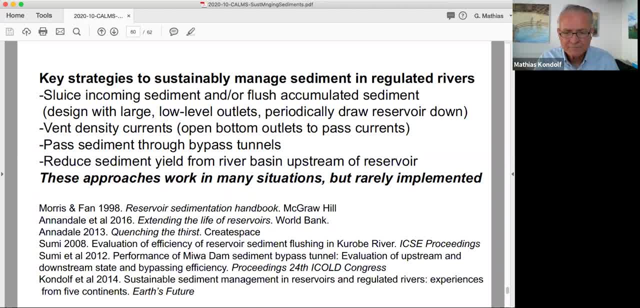 rate And the whole approach ignores the fact that good dam sites are a very limited resource. They are a non-renewable resource And most of the good dam sites, certainly in the developed world, have already been taken. You know, when you look at how CalFed was struggling to find good places to build another. 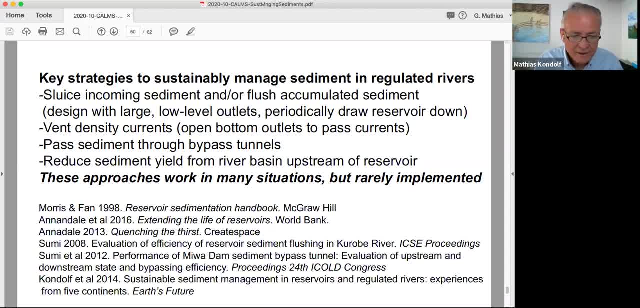 reservoir. You know, it's pretty clear that we're just fooling around with the dregs now. I mean, we had the really good dam. sites are already taken, So there's a lot of reasons why we should be trying to maintain our reservoir capacity. 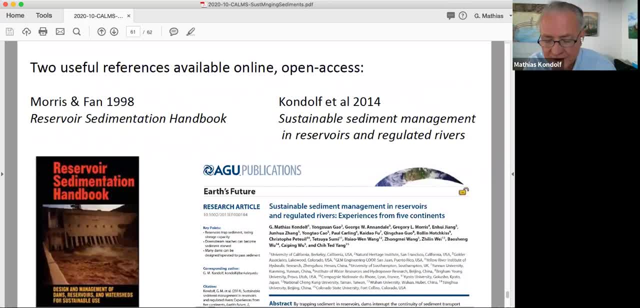 And I would say that you know one of. certainly in California, one of the first things should be having some information about what is the remaining reservoir capacity. You know what is the remaining reservoir capacity? How quickly are we losing it? 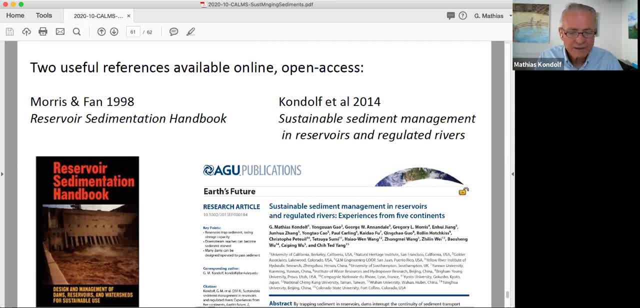 Get a little more information that might then inform us of a way that we can maintain this. We can't just blindly assume that we fill up the existing reservoirs we're going to build new ones. No, that's not going to work. 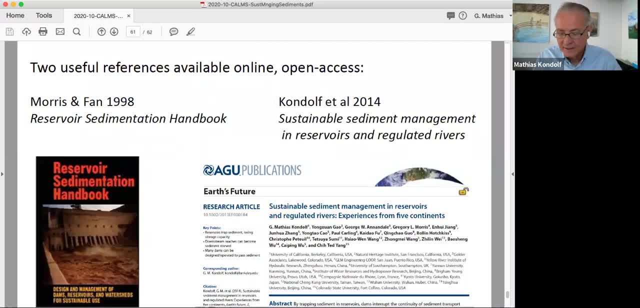 Or it's going to be really expensive and there'll be a lot more impacts to do it. Plus, you know, try building a big project nowadays with the permitting requirements Okay. So I draw your attention to these two questions. They're both references. 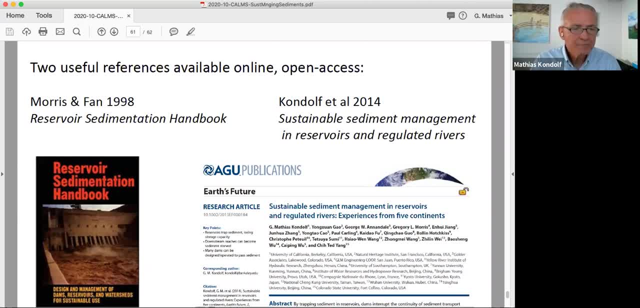 They are both available online, open access. Greg Morris: his book Reservoir Sedimentation Handbook is really. it is the classic in the field And it was published by McGraw-Hill and their- whatever their- rights to the book expired. 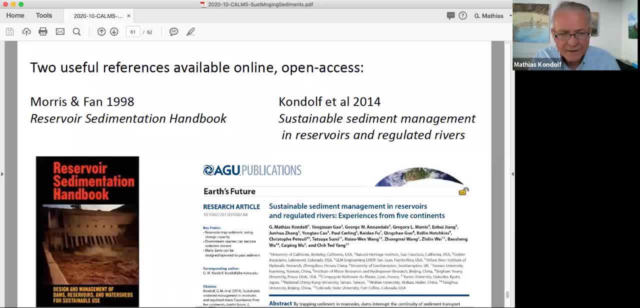 about five or 10 years ago And Greg said: well, you know, go get it. Okay, I'll take the rights. And then Greg just had it scanned and put it online as an ebook. Anyone can download it, And that's been a great resource for people all over the world. 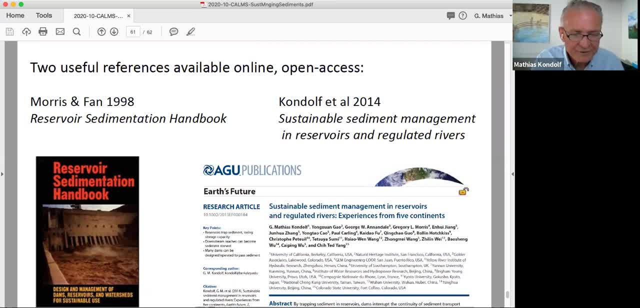 And you have to fill out a little form. you know where you're from, So Greg has got this tally of you. know people from all over the world getting this book. More recently, this paper that we published with Greg and George, Annandale and Tetsuya. 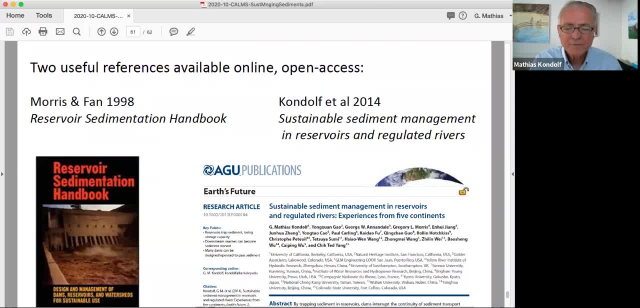 Sumi and others. It's called On Sustainable Management of Sediment, Reservoirs and Regulated Rivers. This is in the first year of the AGU publication, Earth's Future, And this is an open access journal, So if you just type this title in, it'll come right up and you can download it for free. 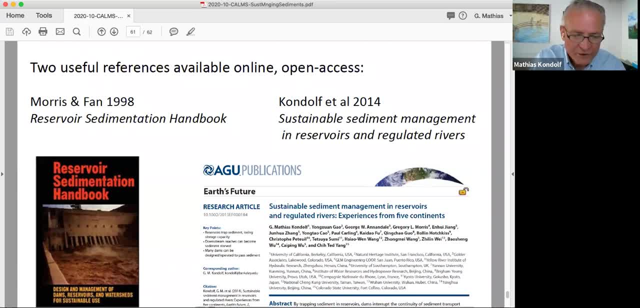 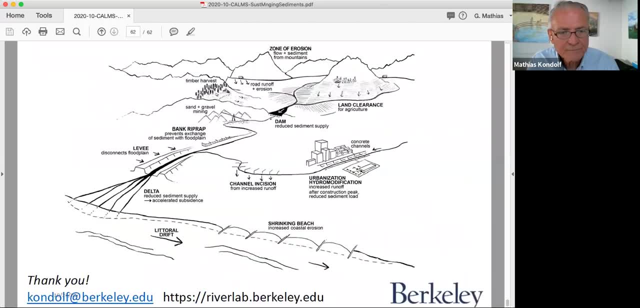 This is, you know, somewhat updated and, of course, way shorter than the book, So it's a good sort of introduction to the kinds of things that I've been talking about here. So thanks for your attention. I'll be happy to answer any questions. 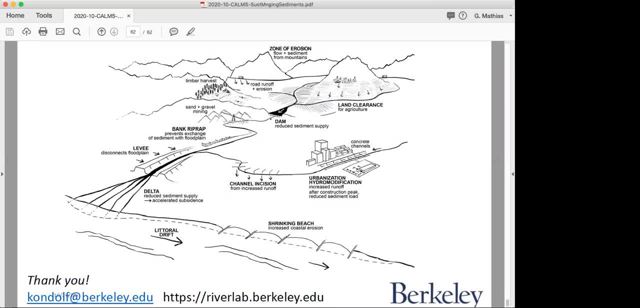 Thanks, Matt. that was a great talk. We got some questions in the chat and so I'll just kind of be going over those to you, But I had a. I had a quick question at first. What are some of the political objections to measuring sediment capacity in reservoirs? 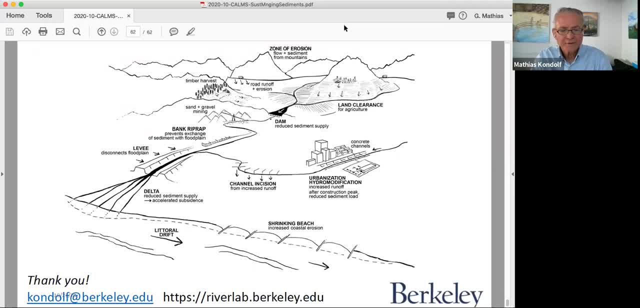 I wasn't involved in in in that, But So what I was told is that some of the districts didn't want problems to be exposed And I don't really see why. I would think that you know the problems are exposed. That would be motivation for them to get more money to solve them. 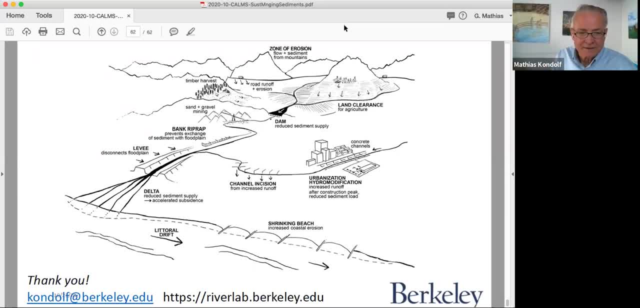 But, but apparently that was it. I guess it's not there if you don't see it Right? Yeah, Yeah, Thank you, Casey Walker. Casey is a potential UCSB master student interested in research on the Ventura River and the Matilha. 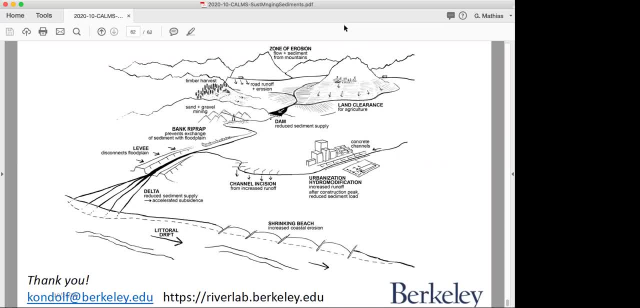 Dam, Wondering if you have any ideas for research, any research ideas or research topics involving Matilha Dam. And in my river restoration class now I have a student who's who's from Ventura County and and she's she's been trying to figure out it. 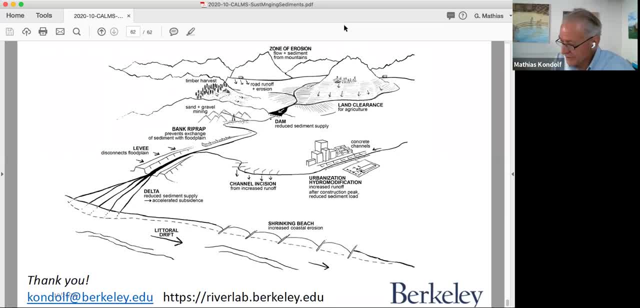 Is there something to do for her term project on on Matilha. Well, one thing I suggested to her- but you know it's not going to be a little too unrealistic- is you have the models that are that are done, predicting how much aggradation there's going? 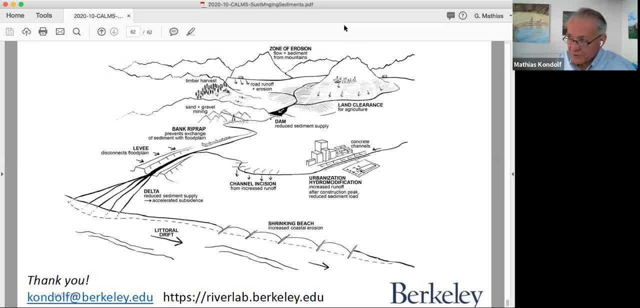 to be, and so on, And, and, and. the one thing you can be sure is when you have a flood, if you know one of these mansions gets destroyed, One of these mansions gets damaged in the flood, They're going to hire an expert and and and attorneys who are going to say it's because 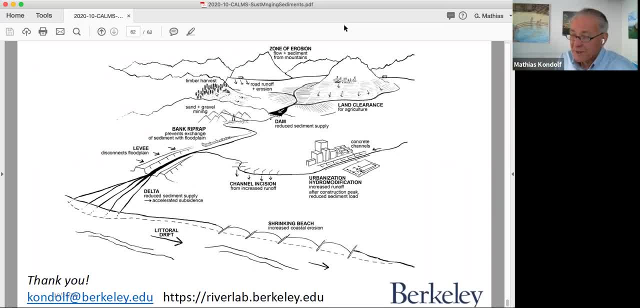 of whatever you did at the dam, you know. But doing doing an inventory of what's downstream could be quite interesting. And there's, you know, usually when these models are run, people maybe they go in the field and they have a look up and downstream of a couple of bridges. 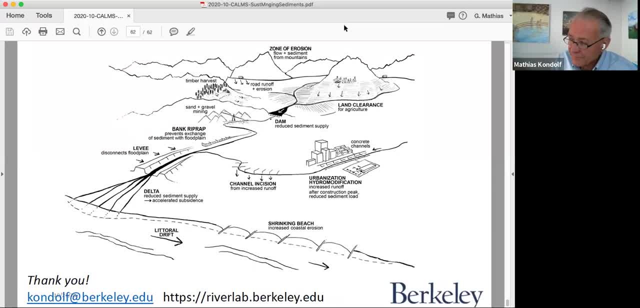 But they don't walk out the whole thing. So so that's that's something I find is often really enlightening. It's just to walk the whole region and and see what, what you discover. But I'd be, but Casey would be happy if you wanted to get in touch sometime. 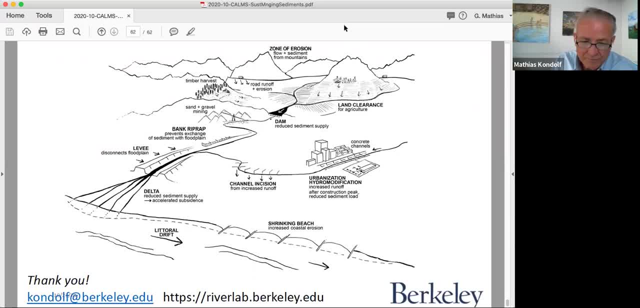 I'll. I'm sure my brain will engage on the topic a little bit more and might have some other more substantive suggestions for you. Joe Sullivan asks: are there any success stories of using sediment bypass channels in California? No, not in California. What the the biggest success of any of these kinds of strategies, I would say, is on the? 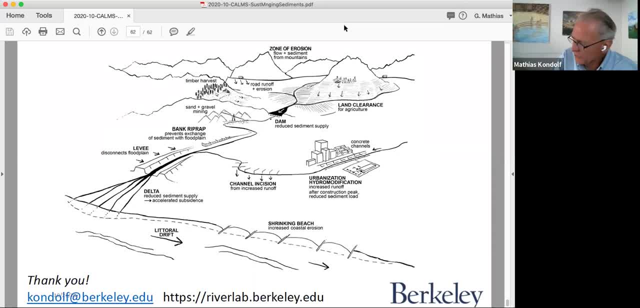 middle American at Ralston, after Bay, before Bay. I forget what that one is, but but there they. they had a problem of, of of sediment accumulation in the reservoir. They excavated about 50,000 cubic yards. about half of that they put in the river channel. 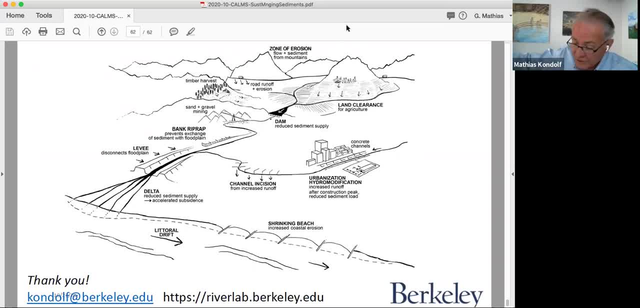 downstream and the other half they they put in, you know, like a disposal site. You know it was just like a waste product. And the reason they didn't put the whole thing in there is they were a little afraid- you know that- that there would be too much. 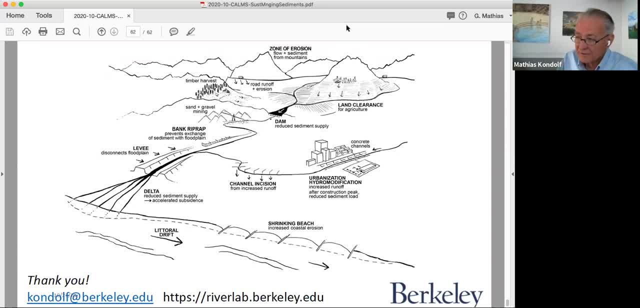 Anyway, the, the, the. the sediment washed out with the first high flow. I forget if it was the next year or a couple of years later, So that's that's the only example we have of actually taking sediment out of the reservoir and mechanically putting it in the channel downstream on the San Gabriel River in the. 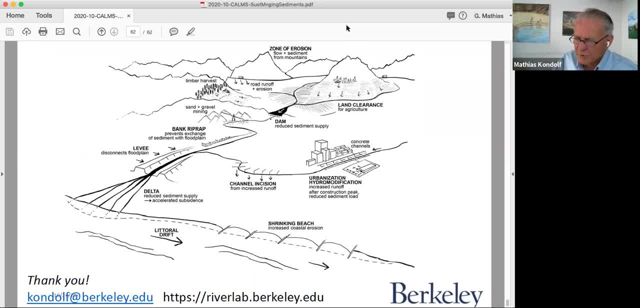 Los Angeles County. They actually have been pretty forward thinking about managing sediment in the San Gabriel River but they got too many objections from people. but they actually were flushing sediment out of the upstream reservoir. There's like three or four reservoirs in a row. 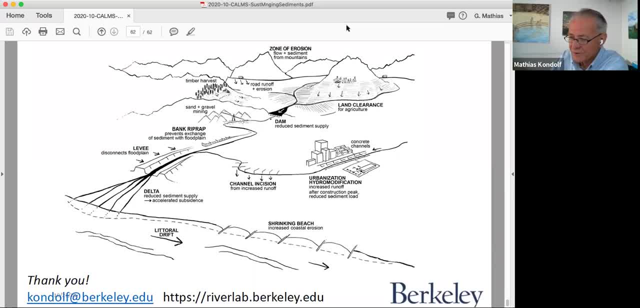 They were actually. they were actually doing this, and you could see that the reservoir sediment accumulating in the next reservoir and then they flushed into the next one. So, anyway, I think I think they were on a pretty good track, but, but but people objected there. 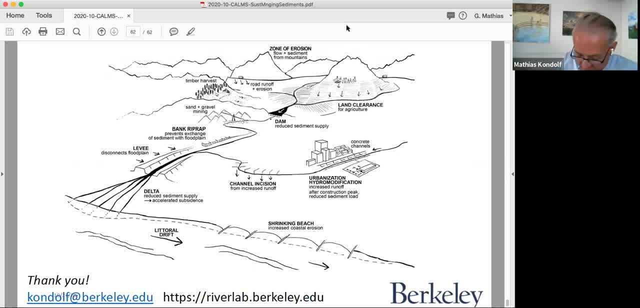 You know, there's always something that changes when you, when you release sediment especially, people get used to having no sediment and nice clean, you know clear water and nice clean river And then suddenly there's all this sediment That's. that's too many people in many people's eyes. 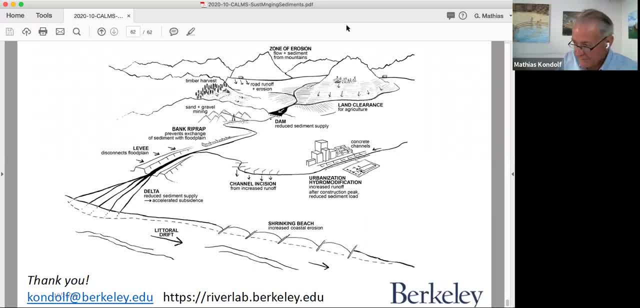 That's like a you know an environmental problem. So we need education, public education. sediment's good up to a point. Kerry Austin asks what a biblical storm like the one that occurred in 1861 to 1862 would mean for sediment loads into an existing reservoir. 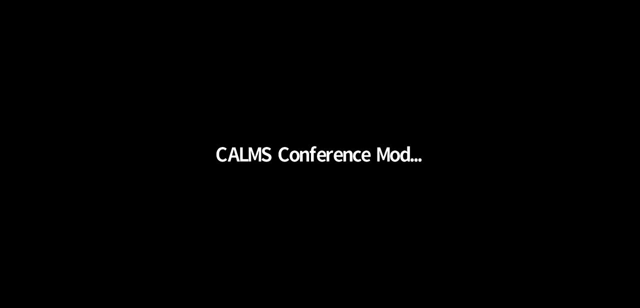 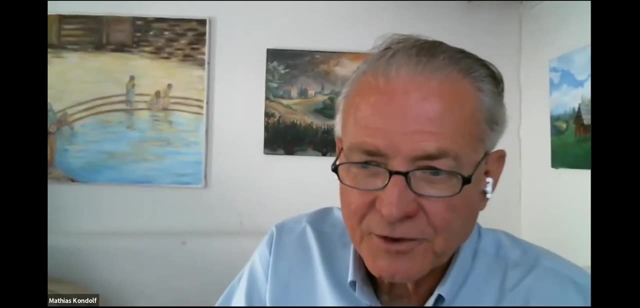 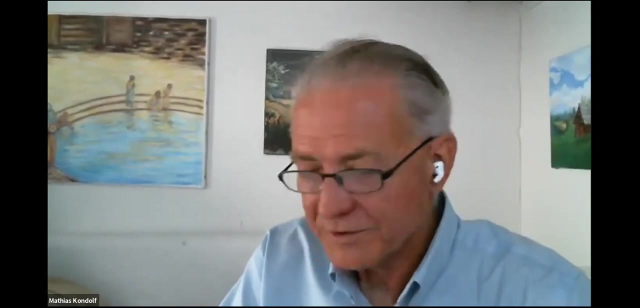 And will they hold up? Hmm, Very good question. Well, I think you- your answer is implied in your question- There will be. I'll go on record of predicting that there will be some reservoirs that will fail in a in a repeat of the 1862 storm. 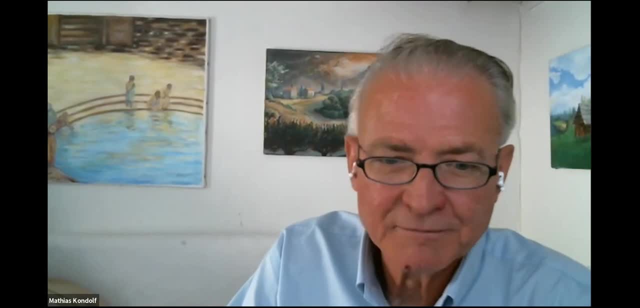 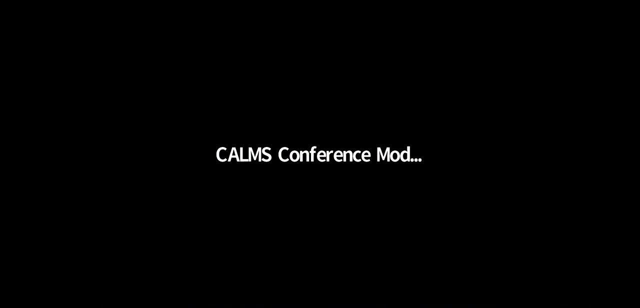 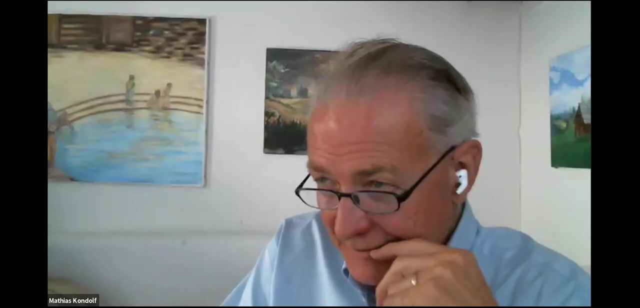 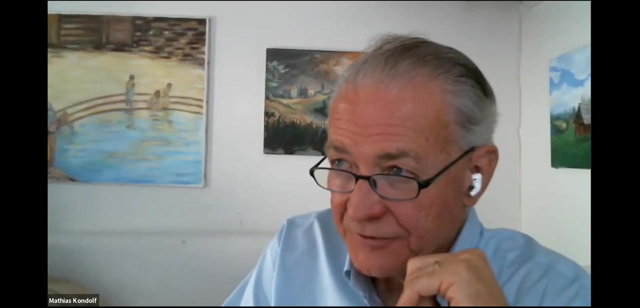 Probably not. I'm probably not going out too far on a limb to say that. Mike Cox asks: should gravel mining return wet screen fines to the stream rather than impoundment Interesting? A lot of that, I'd say, depends on when, If you return the fines. during the winter high flows, it's probably okay. It would probably just get lost in the noise. If you do it during the summer low flow, it would be probably a disaster. Next from Bill Taylor: what's the cost effectiveness of digging bypass tunnels? versus the age and structural integrity of older dams. I'm not sure, if I follow So, how much it would cost to build a bypass tunnel. I'm not sure, if I follow So, how much it would cost to build a bypass tunnel. I'm not sure, if I follow So, how much it would cost to build a bypass tunnel. 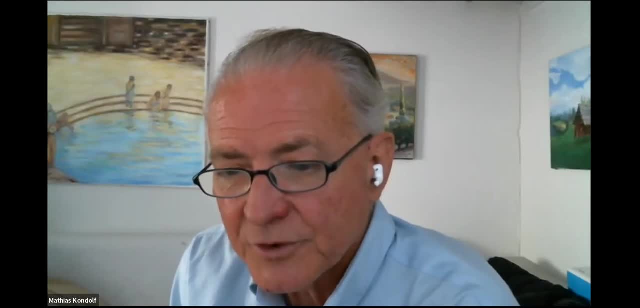 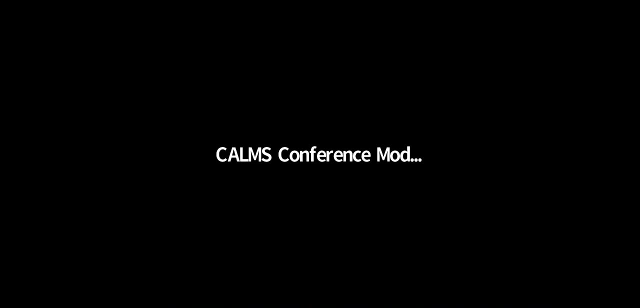 In other words, is it worth it, given that some of the dams are so old and questionable? integrity Bill, could you unmute and clarify? Yeah, that'd be great. Yeah, that's about it. Dams are really expensive to build. And we have tunneling machines that can do a pretty good job of going around them. But eventually these things, like you say, you can only build so many dams and then you run out of options on them. So if you want to save them- and I know, there's all different sizes and capacities. 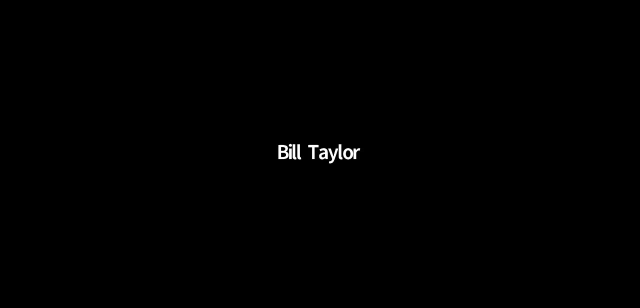 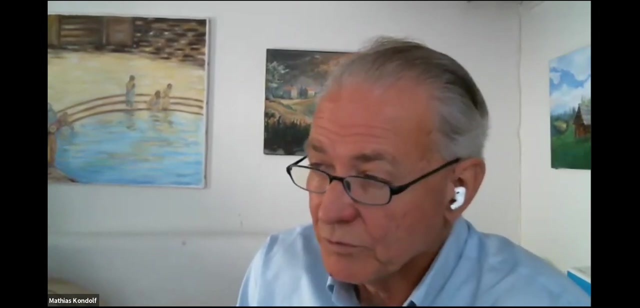 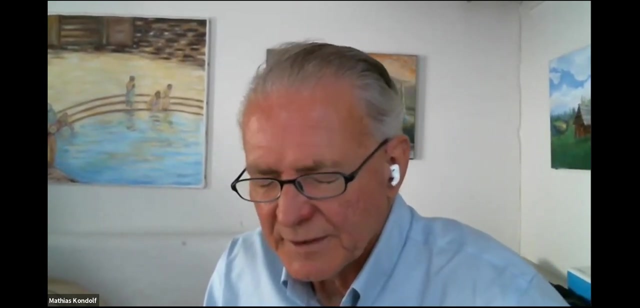 and all of that, but would there be a point where that would be cost effective to work around? Yeah, Yeah. Well, just thinking about the Miwa example, they let it roughly fill halfway with sediment by the time they got motivated to build that bypass tunnel. This is Miwa Dam in Japan And it still functions. It still generates. 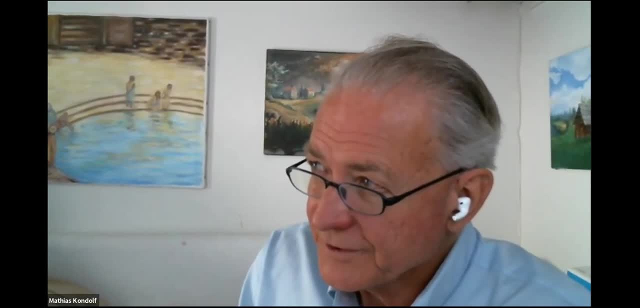 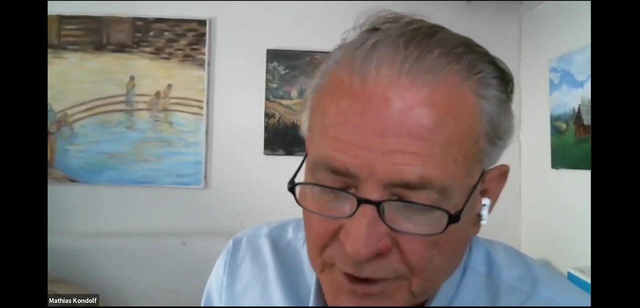 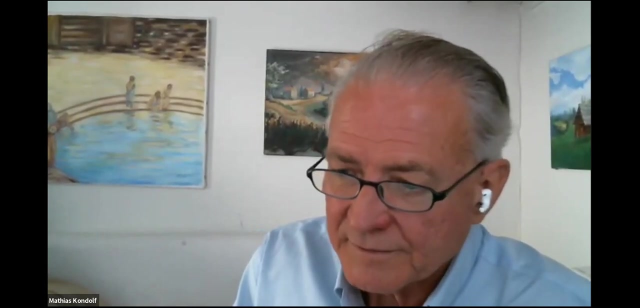 power and diverts water and so on. So I guess it's probably, of course, a case-by-case analysis, But given the lack of good dam sites sitting out there waiting for us to build in, I think that all the dams that we have now we have to treat as important assets that. 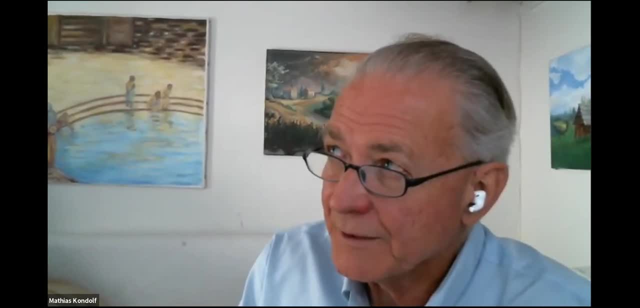 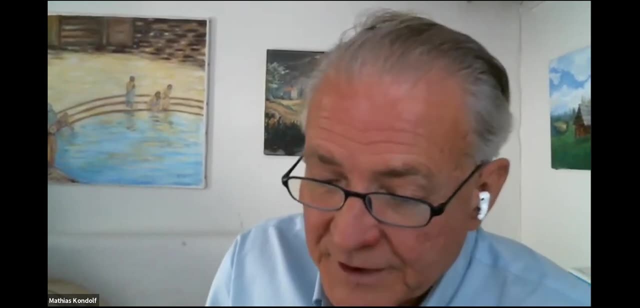 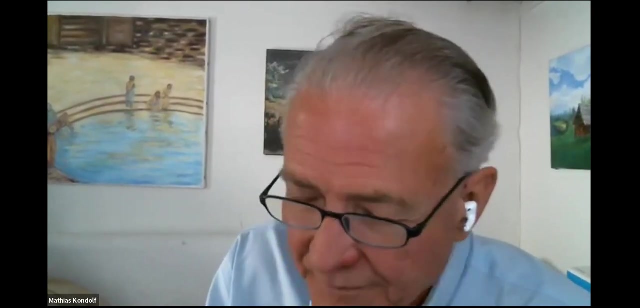 we should prolong their life as much as possible. So I would think in many cases it would make sense, But this would be a great thing. I think the first thing is have DWR figure out which reservoirs are filling with sediment, how fast, and I know there was some discussion. 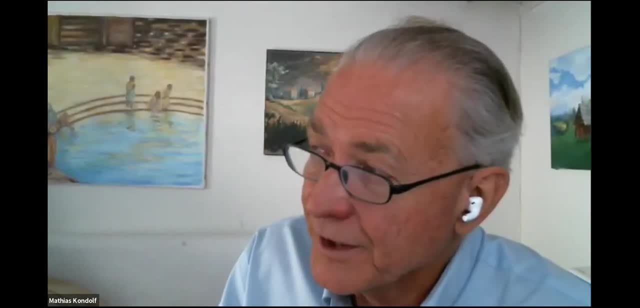 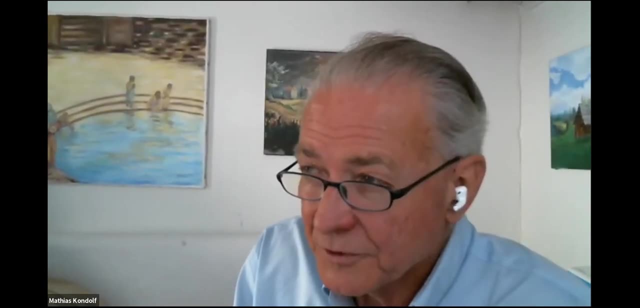 back and forth where they didn't want to do all the dams in the state, but they were going to to try to prioritize certain ones, which is fine. but then I think a next step could be trying to answer your question and for a lot of these, you know a lot of these dams. I'm sure it does make. 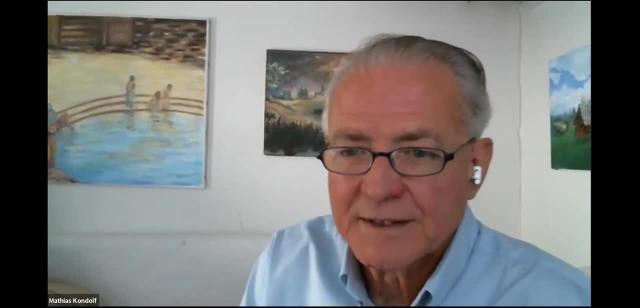 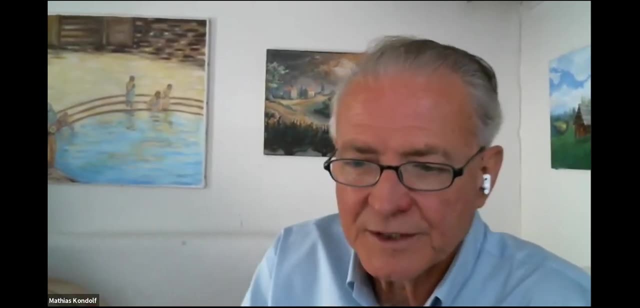 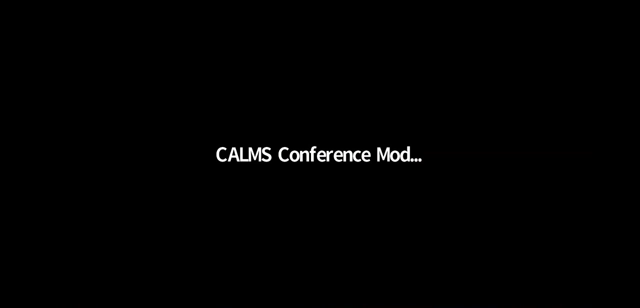 economic sense, and for some others it probably doesn't. but there, but we could probably figure out ways of making a fairly quick assessment of that initially, before doing a detailed study. Kenneth Leroux has two questions, So the first one is: what are your thoughts on the long-term? 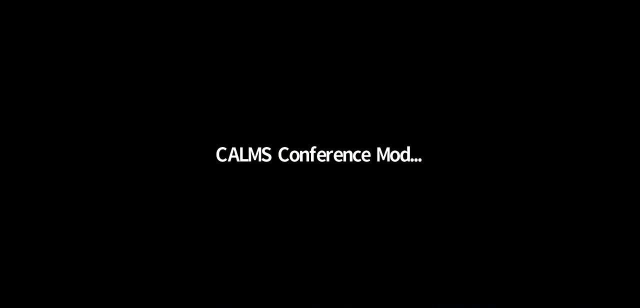 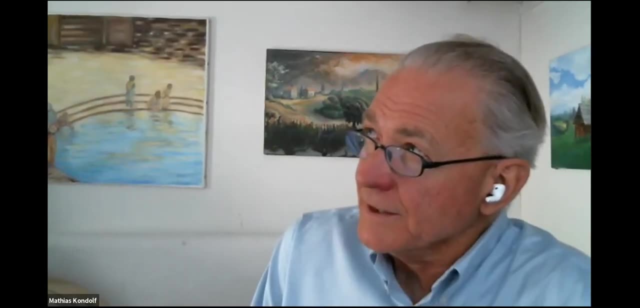 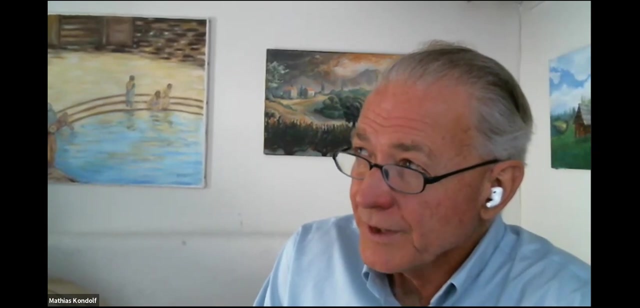 viability and implications of gravel augmentation, since this method leaves the water starved of fine sediments. Yeah now, so there are. in some cases it below smaller dams. the smaller dams can pass more of the sediment than the smaller dams- The smaller dams can pass more of the sediment. 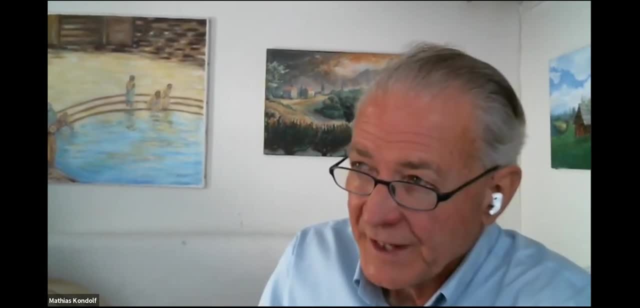 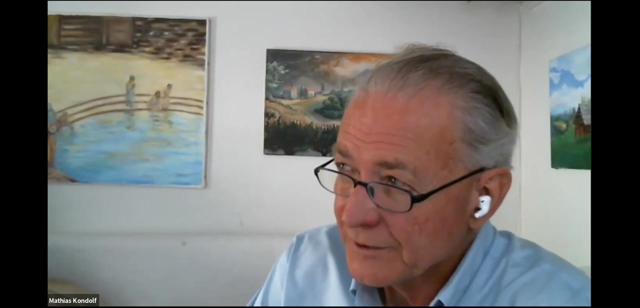 So it just depends on what's the capacity of the dam. It's usually we talk about the impoundment ratio. if the dam is impounds, you know, five percent of the annual flow or less, usually it can pass a certain amount of the fines around. So it might not be fine sediment starved so much and the fines 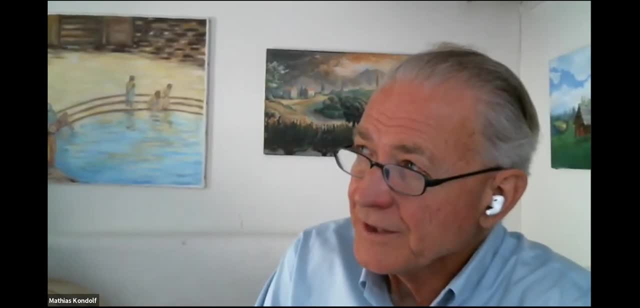 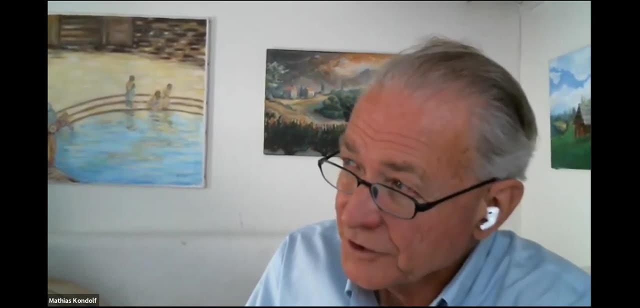 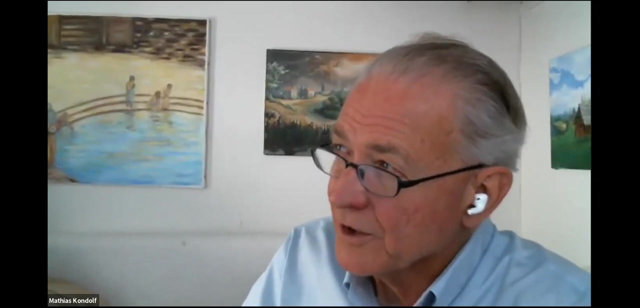 would be moving at the natural time of the year, I would say the. but your broader question of how sustainable is this? I think that's really a good question. You know, I did my dissertation research on gravels and I love gravel and I am always excited to see gravel being put in rivers. below dams. but you know how sustainable is that really, and it was. it was only the mid 90s when Fish and Game stopped buying gravel to to put in the Sacramento River for for salmon, and they stopped buying it from gravel miners who were taking it out of tributaries like Cottonwood Creek. You know so. 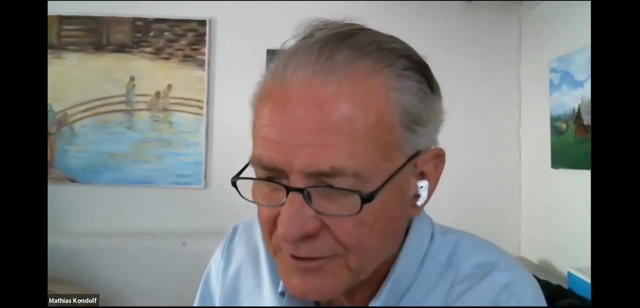 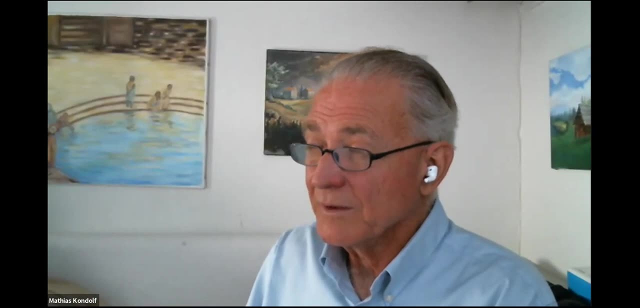 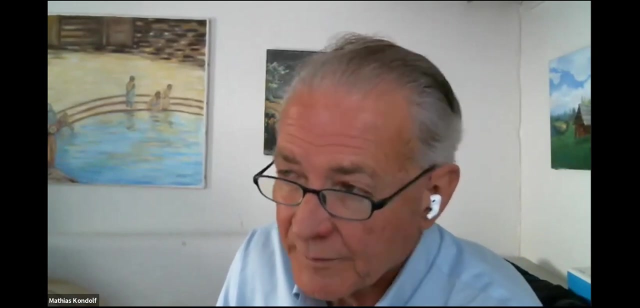 so there are impacts on where you get the gravel for this augmentation project and well, one great source that that we've had are the old dredger tailings, like along the Merced and Tuolumne Rivers and a lot of these projects to to isolate some of the old gravel pits. 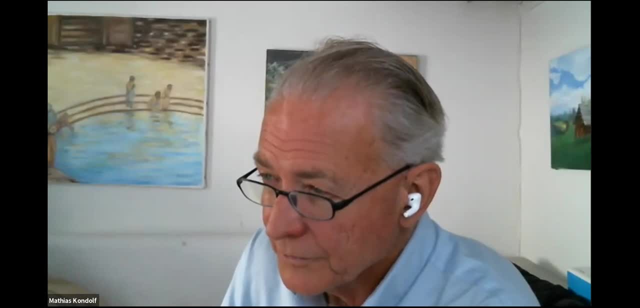 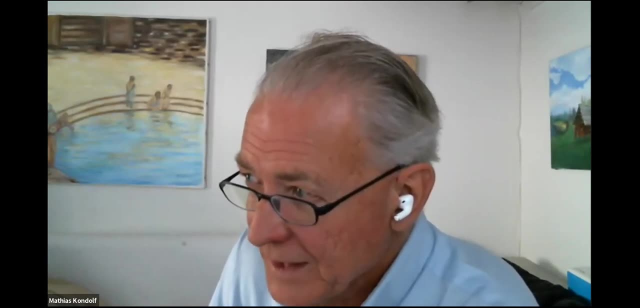 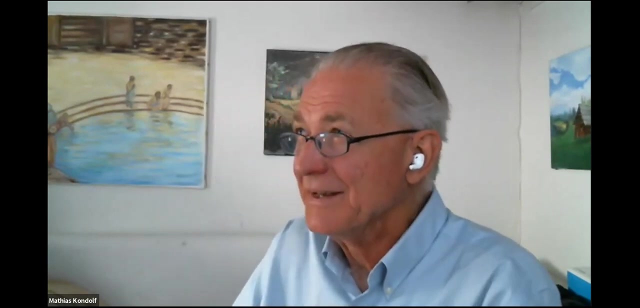 and and to add gravel to the system, were, were conceived and priced out based on these dredger tailings being worthless, which is what they were, but the, the, these restoration projects created a market for this stuff and then and then the prices of course went up, but but it does highlight that 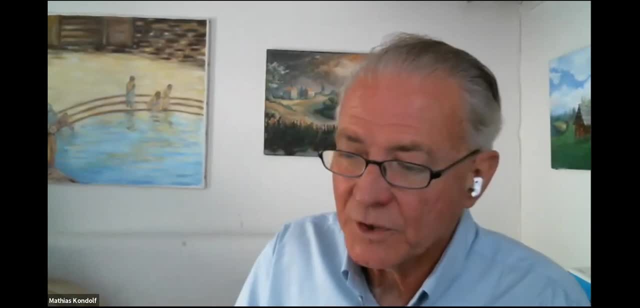 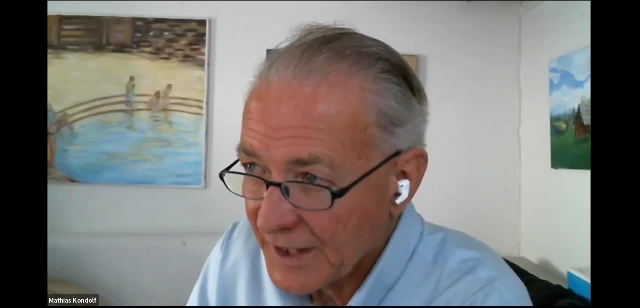 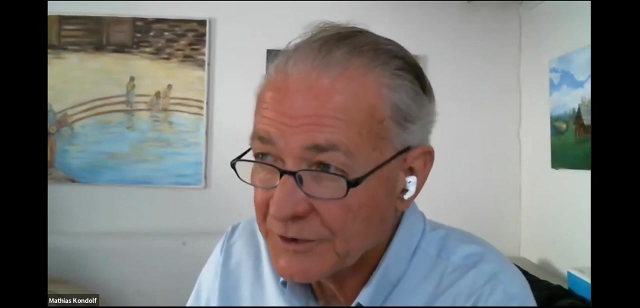 you need to get the gravel from somewhere And where you have dredger tailings, that's a pretty good source. If you have to take it from other places, you're competing on this aggregate market for this aggregate, which is increasingly expensive, So I think there are questions. 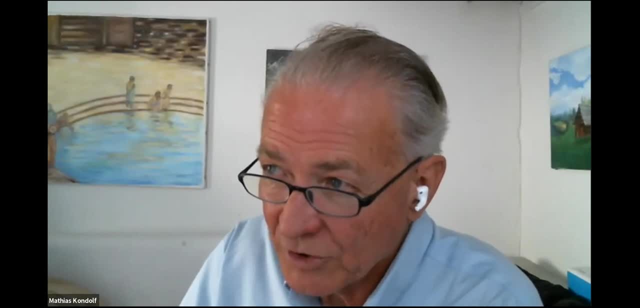 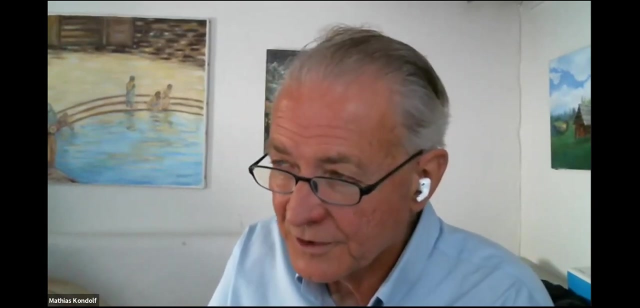 about the long-term viability of the gravel augmentation, unless you take it from the reservoir itself. And then you get into all the costs of removing it, trucking it around and you have all these other institutional issues. A lot of these reservoirs were set up. 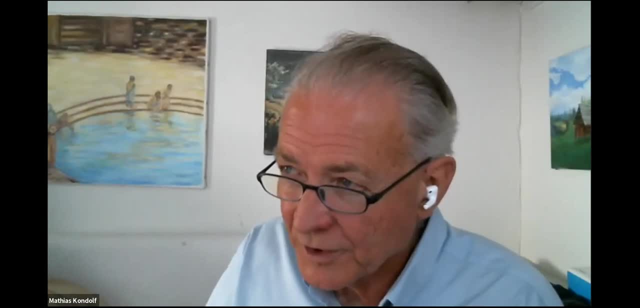 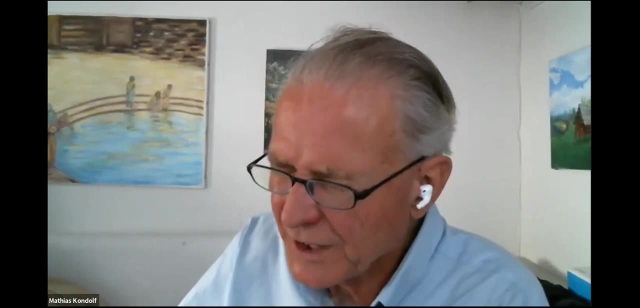 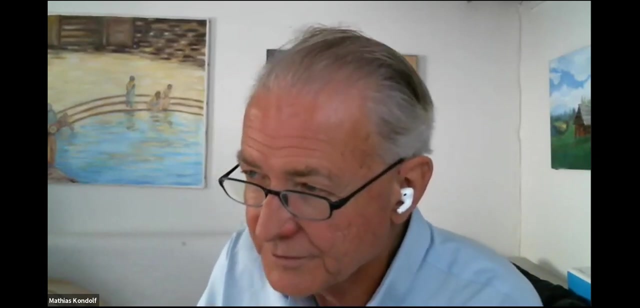 to pass their cost-benefit test, They had to make the reservoir a recreation area, And an industrial activity like mining, extracting the gravel and sand from the head of the reservoir- that conflicts with it Use as a recreational area. So there are all kinds of conflicts that arise with that. But that's the sustainable ways. taking it from the reservoir itself Just hard. So the second part of the question was: mercury contamination also complicates dam removal and sediment management. in California, Sediment flushing or bypassing doesn't appear to be viable in these reservoirs. So how might we deal with mercury-contaminated reservoirs nearing? 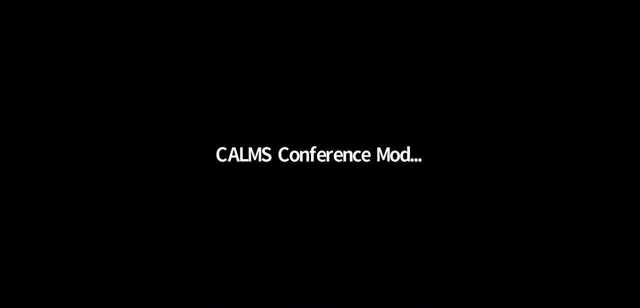 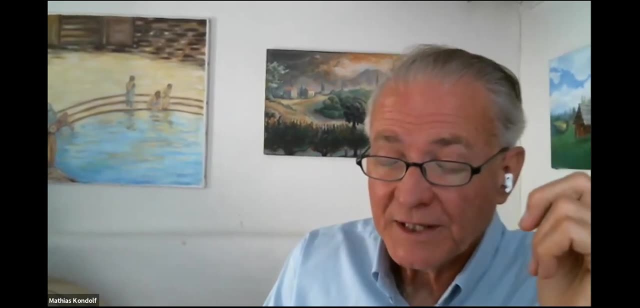 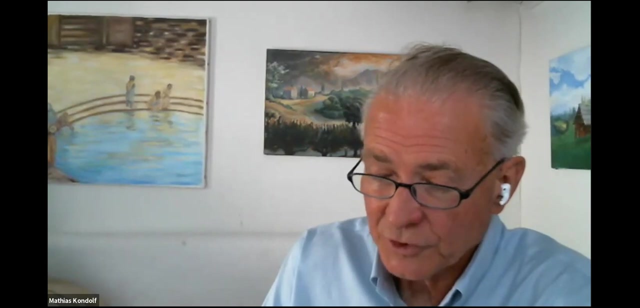 capacity. Well, first, maybe the incoming sediment is not contaminated at this point. You probably need to check that. But if it seems like the incoming sediment is not so bad, perhaps a bypass or even a sluicing option, sediment routing might work. But how you deal with, 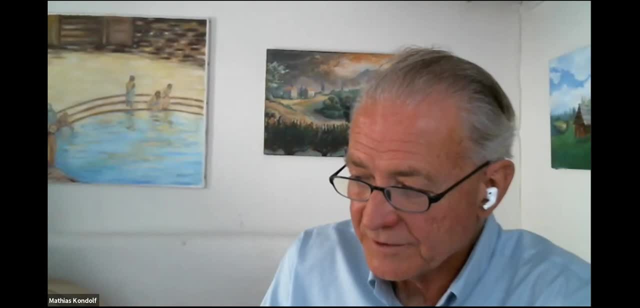 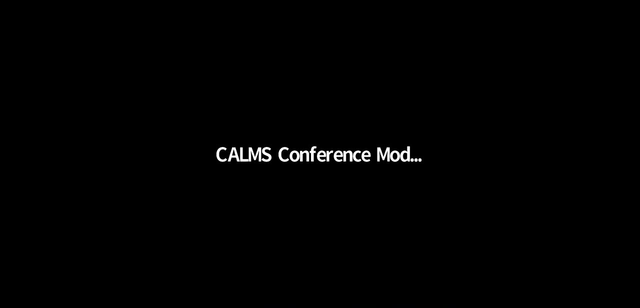 these reservoirs and how do you deal with these reservoirs? you know decades of accumulation of mercury-contaminated sediment. that's the kind of problem I would turn over to someone like Mark. And that is a problem. I would turn over to someone like Kerry Austin. 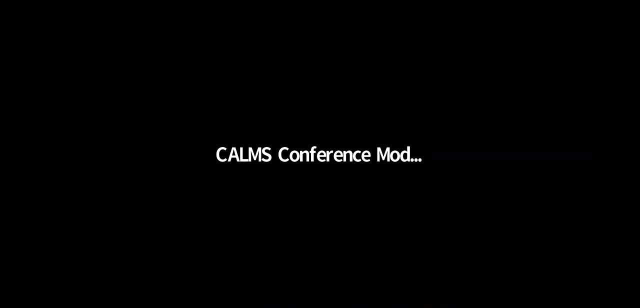 Yeah, we, you know. so my agency, Valley Water, manages reservoirs that are contaminated by the New Almaden Mining District, which is North America's largest historic mercury mine. A lot of these reservoirs are built on old mine waste materials And they've received mining. 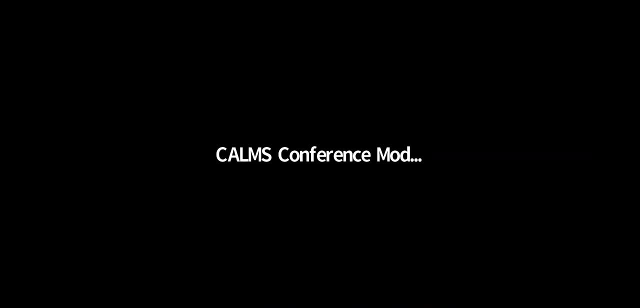 wastes over land throughout the years since, you know, the early 1900s, And a few of these reservoirs have seismic retrofit projects planned, And so that's one of the things that we're considering, you know. is it more appropriate to cap, Do we want to remove some of the sediment to? 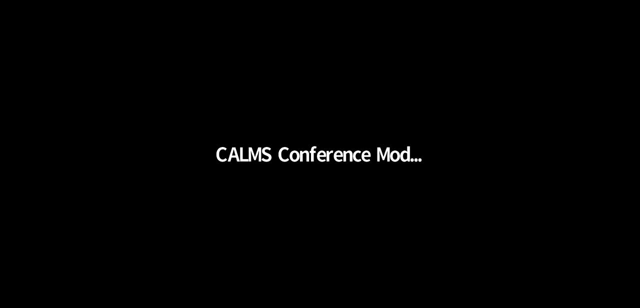 get some of the capacity back. Do we have to send that sediment out to Nevada and have it buried in the desert? At a certain point it gets prohibitively expensive And it goes back to that cost-benefit question: is it actually worth it? It seems like capping kind of seems to be the preferred method. 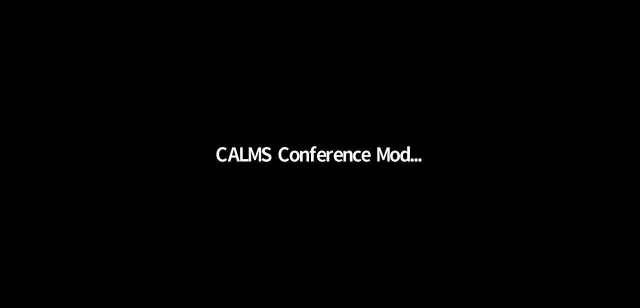 right now, given that- And yeah, what Matt was talking about with cleaner sediment coming in is definitely true. If you look at coring data in the reservoirs, we definitely see that you can see a pretty predictable decrease in sediment mercury concentration with time. 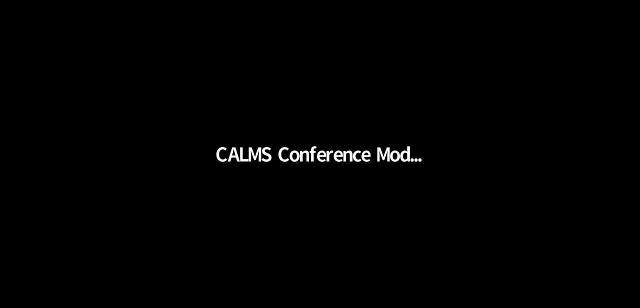 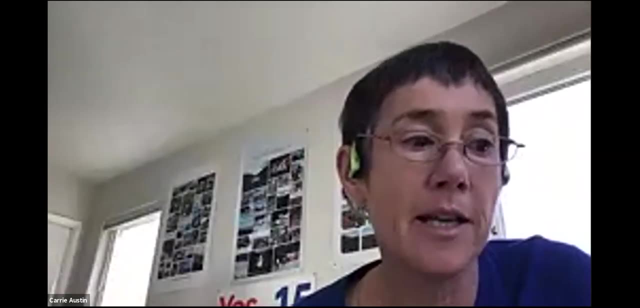 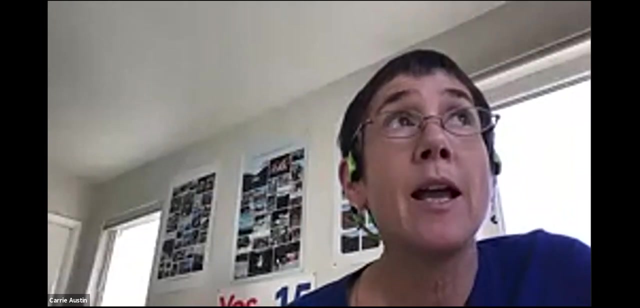 Carrie, I don't know if you want to chime in on that. Yeah, I do. Thank you. I was thinking about Lake Combee, which is up in the Sierra Nevada, so outside of the region where Mark and I work. Lake Combee has a project to do some dredging out of it. 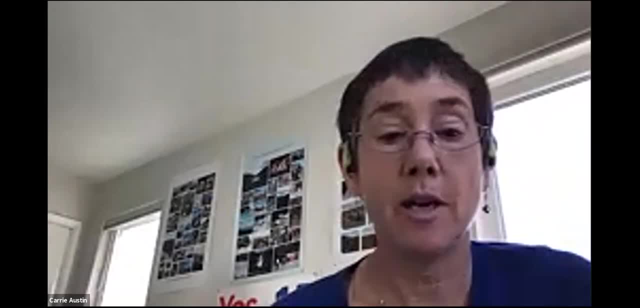 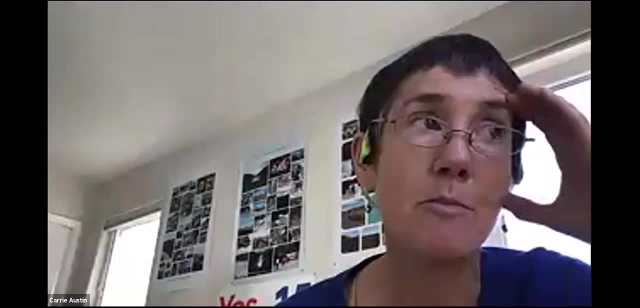 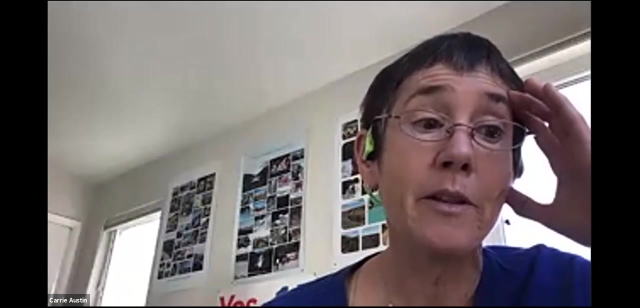 But the mercury issue is extreme there. I was trying to look up- I don't remember how many gold mines were upstream that used mercury, but it's a very large number. And so this problem with reservoirs with contaminated sediment, if it still is coming in. 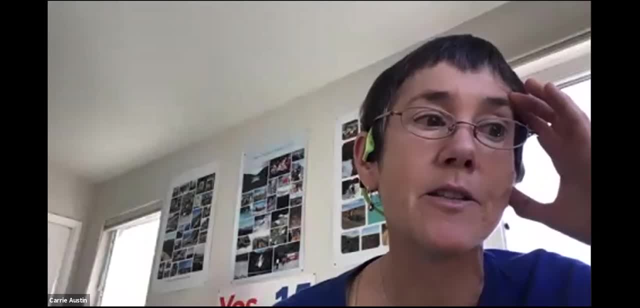 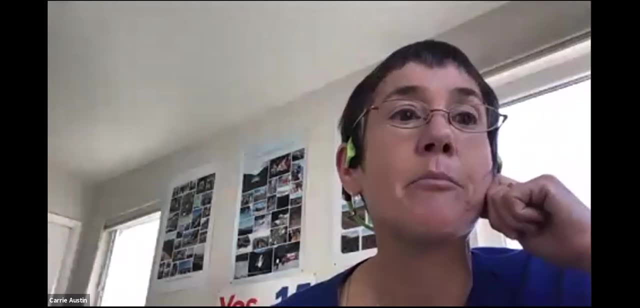 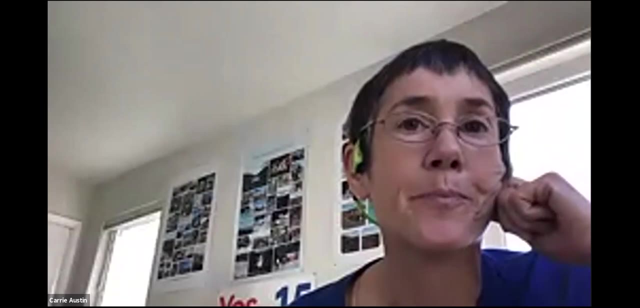 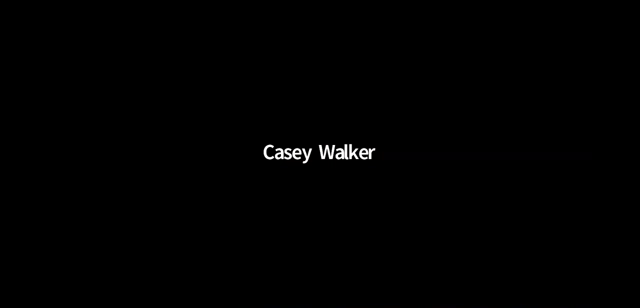 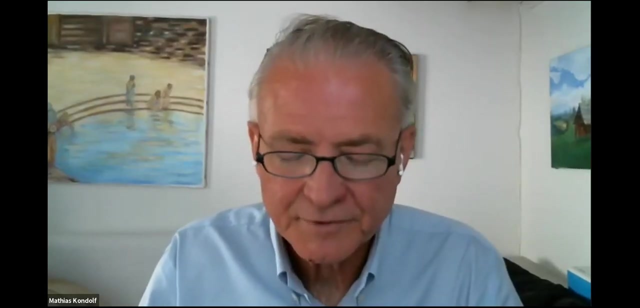 then what you do within the reservoir to manage the sediment could quickly be erased in the next four over the next decade. So there's some real considerations and there's no perfect solutions, as we all know. Yeah, I know Combee is a good poster child, like you said, I know. 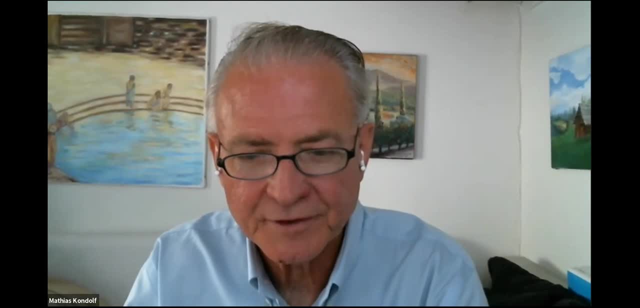 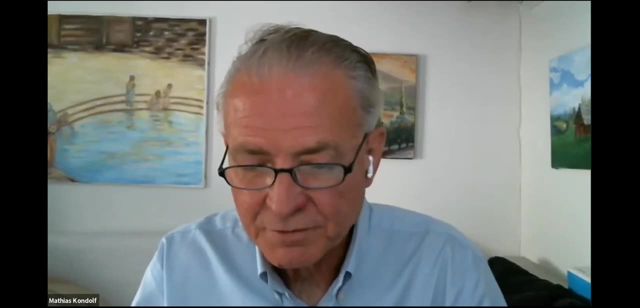 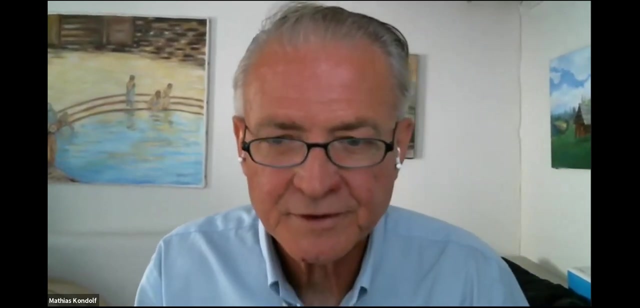 the bro that I saw. I know another Carrie. Carrie Monahan, with the Sierra Fund has been working on that project And it's a huge problem. Mercury and mercury methylation is beyond my area of expertise so I can't really offer a solution there. 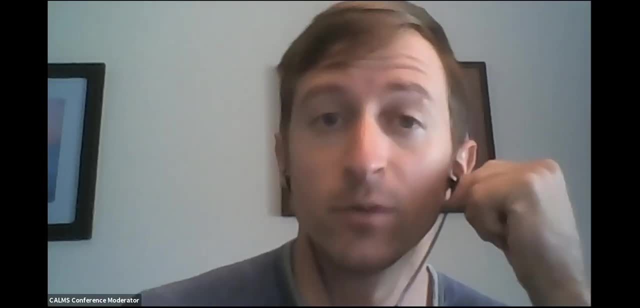 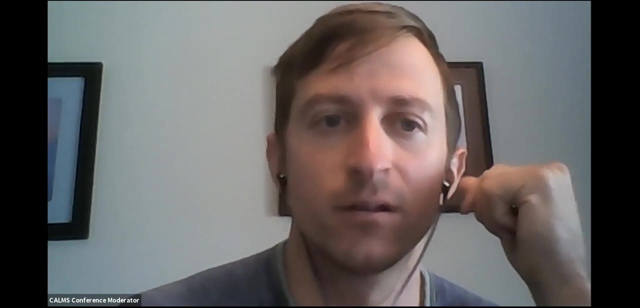 Yeah, I guess. one more thing I'd mention is regarding sediment removals in mercury contaminated reservoirs. Yes, Yeah, You want to be careful that you're not exposing hotter sediment when you remove sediment, So that might be another reason for just maintaining the lower capacity and dealing with it. 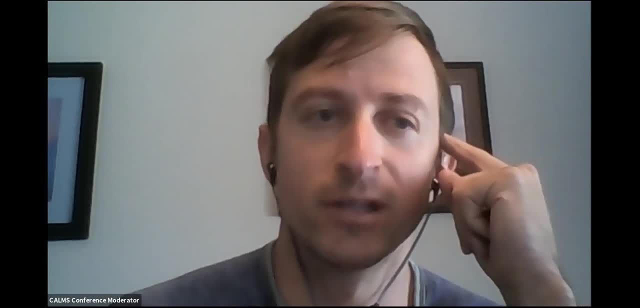 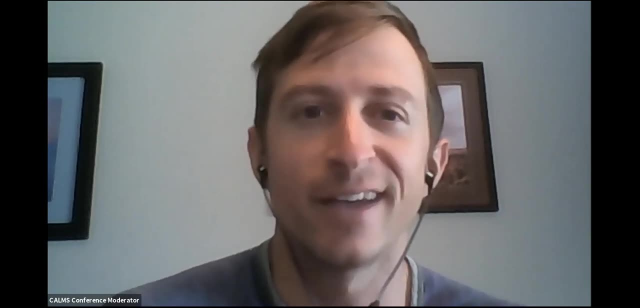 Because it might be the case that you know, you think you're removing a bunch of contaminated sediment, but then you end up removing a few meters and you actually have that. you know that 1890s sediment instead of the modern day sediment. 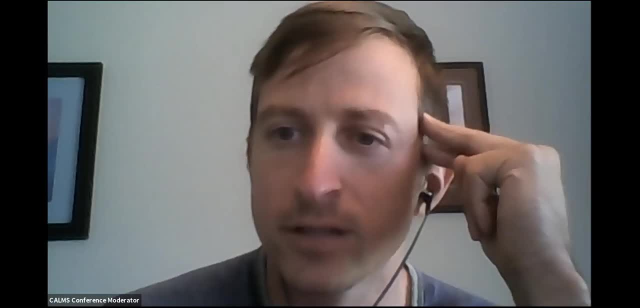 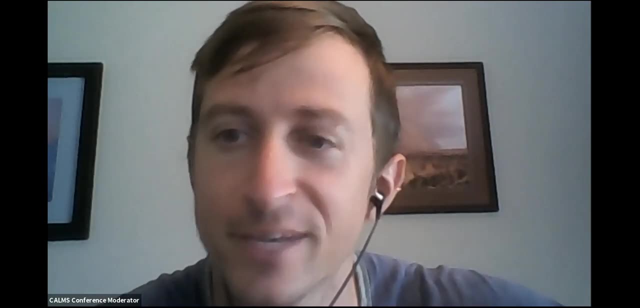 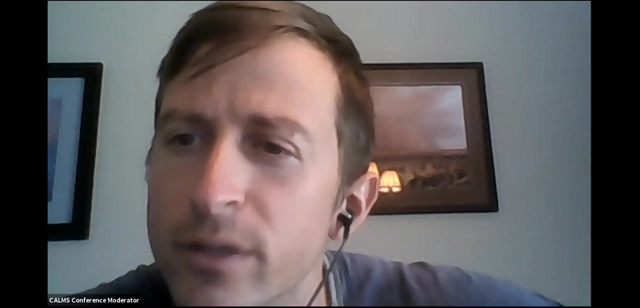 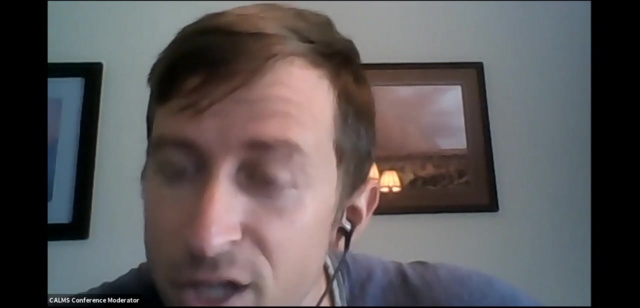 And so that might be a good segue into Mike Cox's next question, who I believe actually lives downstream from a mercury contaminated reservoir. Has any government, has any government- accomplished tort reform and insurance fund for downstream property impacts? Has anyone used dynamic compaction to stabilize dam removal bottom sediments? A couple more questions in there. Maybe we'll start with those. Okay, I think this question of liability for downstream, that's really key And I don't think that's been addressed head on. So I think the answer is no. Like in the case of the San Clemente Dam, I was a little surprised that it actually went through when you consider how wealthy and litiginous some of the downstream. 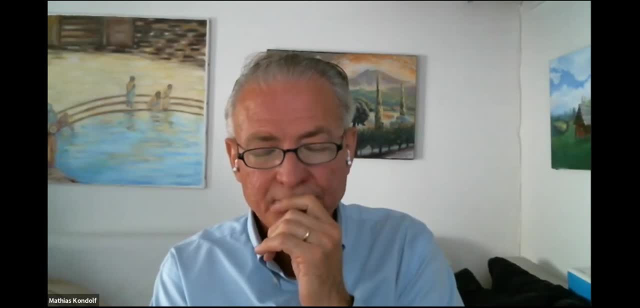 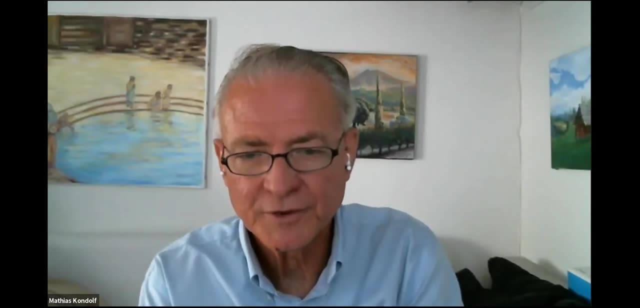 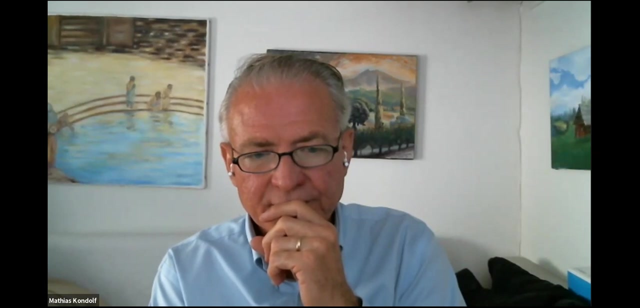 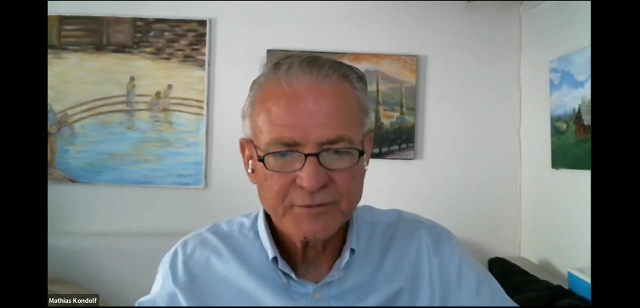 Property owners are. But the model showed that you know it wouldn't be, sediment contributions would not be so serious and would not be creating flooding problems. In terms of dynamic compaction for sediments that are left behind to be stabilized, Well, I guess the main example would be San Clemente. I know that at the edges, at the ends, the downstream, the upstream ends, they were certainly were doing some kind of compaction because they created these, you know these walls and then they protected them further, hardened them further. 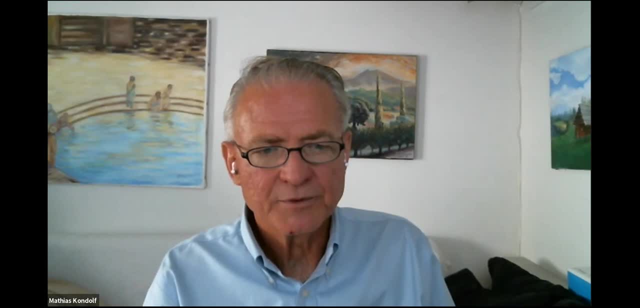 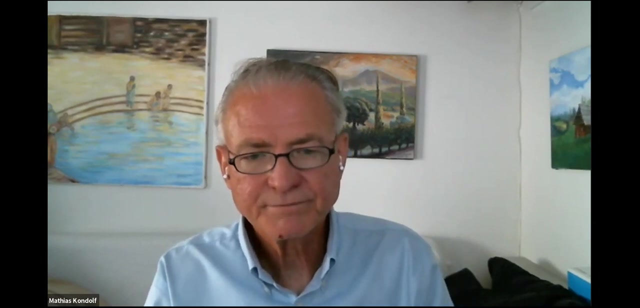 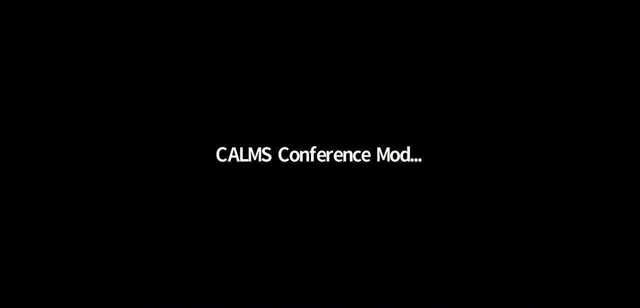 I got another question just come in from Mark Butel. Mark says the Mekong Delta case study was fascinating and scary. What is the long-term diagnosis for the Sacramento- San Joaquin Delta? Is it sediment starved and will it get flooded out with rising sea level? Yes and yes, It's sediment starved, but it's a little different in that some of it is self-inflicted. The Delta itself in 1850 was full of fluffy sediments. It was supporting plant life and everything, but there was a lot of organics. 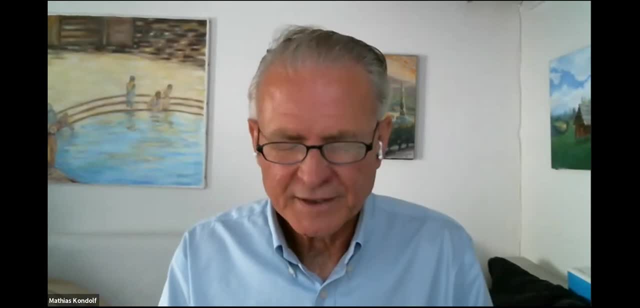 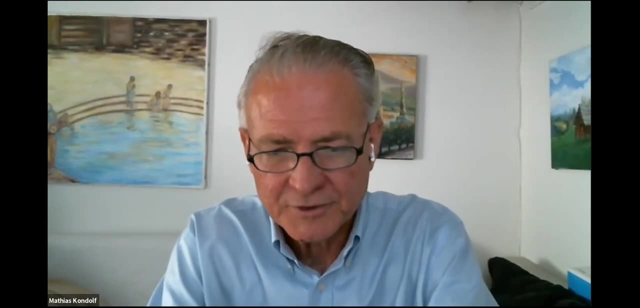 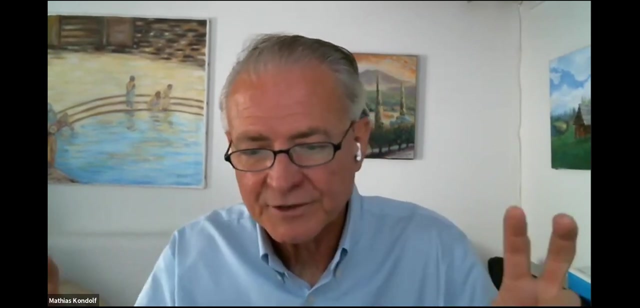 Just by- as you know the story, just by by diking it off and draining it and running the pumps so that you could farm on the surface that was gradually subsiding that. it was resulted in these islands so-called being far below sea level. 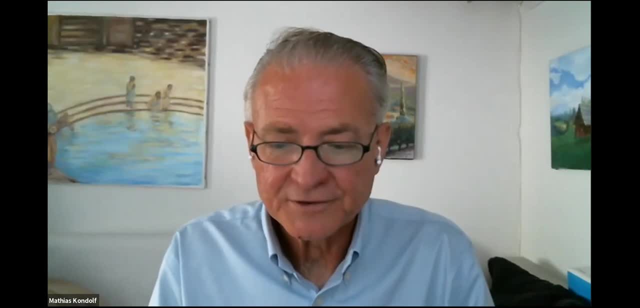 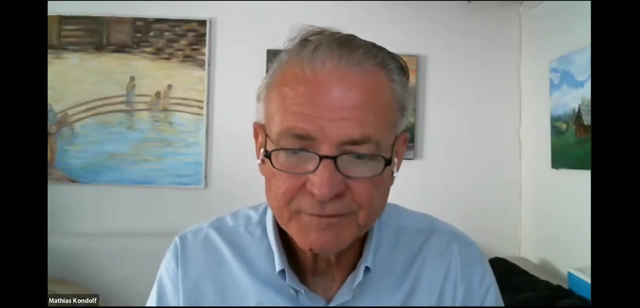 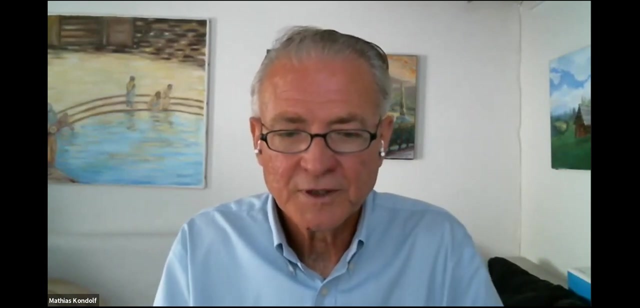 I think it's pretty clear to everybody that this is a disaster that's waiting to happen And we don't really have a good solution for it. We have some experiments that have showed some positive results for regaining elevation within these quote islands, where you convert it back to wetlands, and 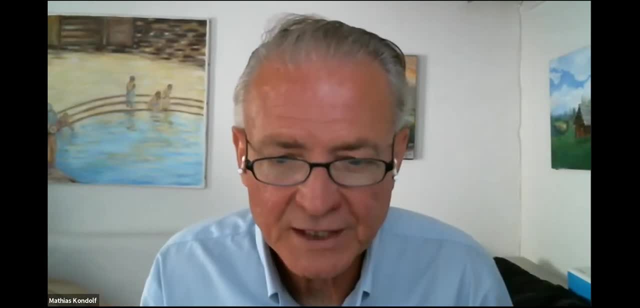 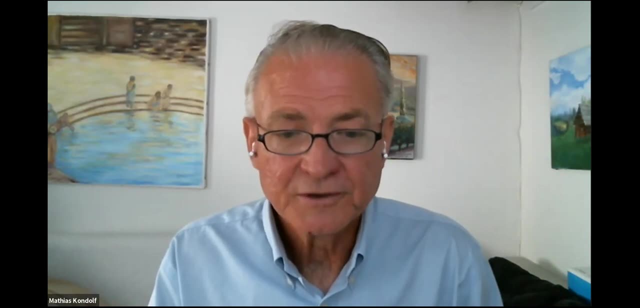 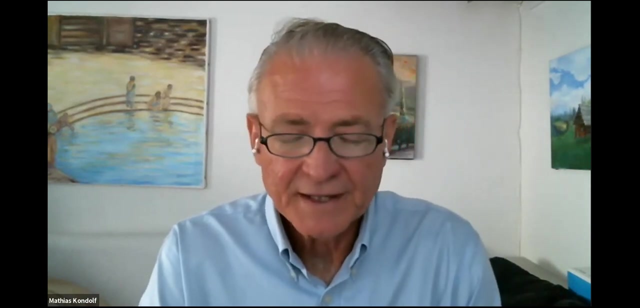 you can get plants to grow and you can start regaining some of that lost elevation, But a lot of the islands are still being used as agriculture and, by definition, those are still subsiding. So all we need is a good earthquake and I think it's inevitable that a lot of these dikes are going to fail. 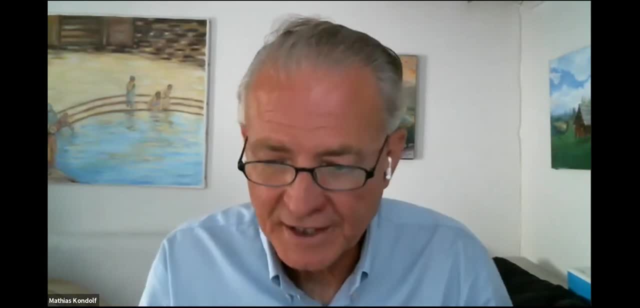 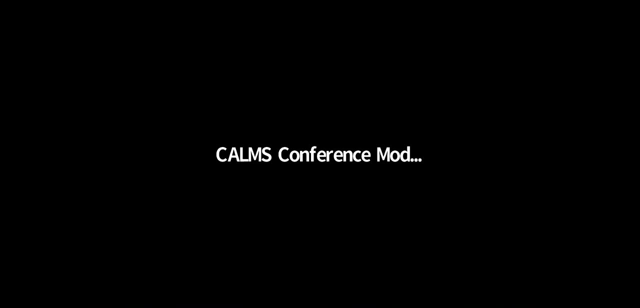 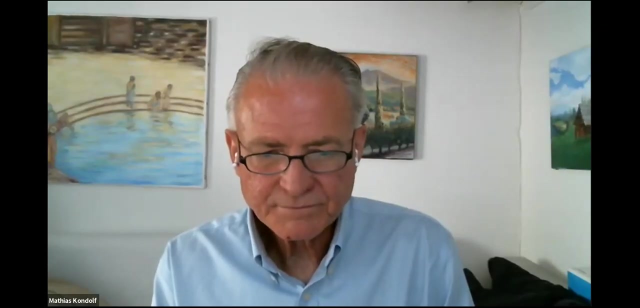 And rising sea level is just the icing on the cake in this instance, I think. Another question, Matt: I was wondering if new reservoirs are being built with sustainable sediment management in mind or if that's more of like a reactive management. Great question. In the Mekong, for example, I was working with the Mekong River Commission and 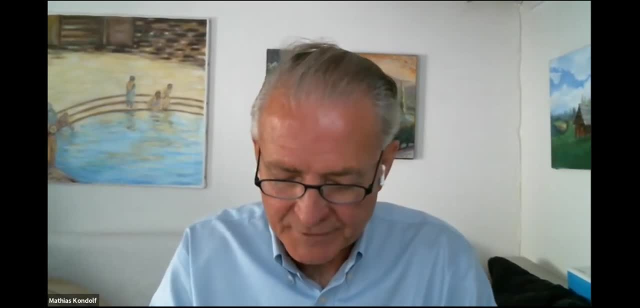 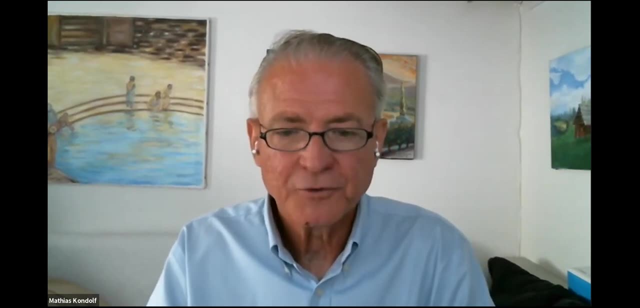 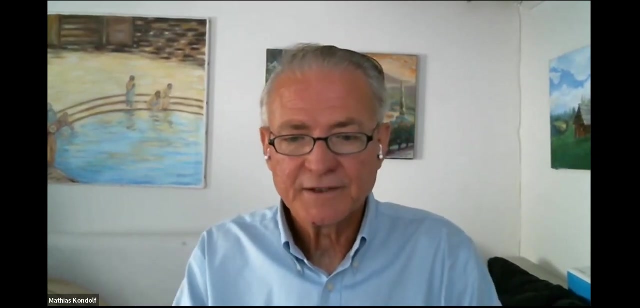 wrote the sediment section for their guidelines for main stem dams And these apply to the lower basin countries that are part of the Mekong River Commission and only for the main stem dams. But the first two main stem dams that you know, one is built and one is being built. 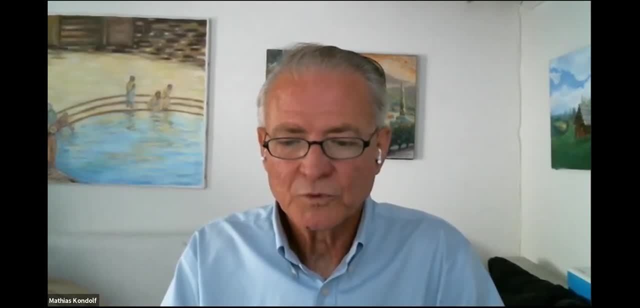 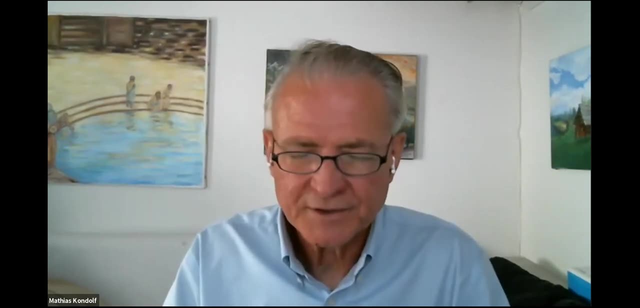 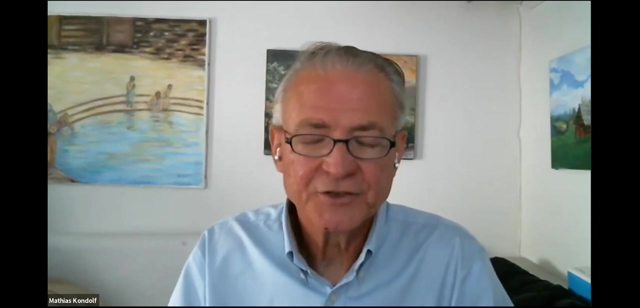 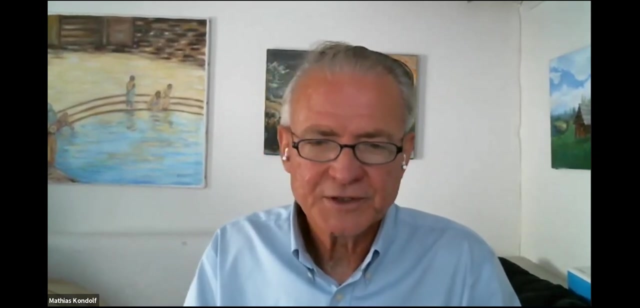 and it's a relatively new project. Two are field subs and one's already been build needed and I think the cost per square centimeter I just see the two such dams touched play really well results in some of theウ Today. on their plans and their documents they accepted these principles that you want to pass. the sediment through, And so, at least in their case, they did design some features like that, But questions still remained about how effective they would be and some of the details of the design. But you know, you could say in that case they would be on site. 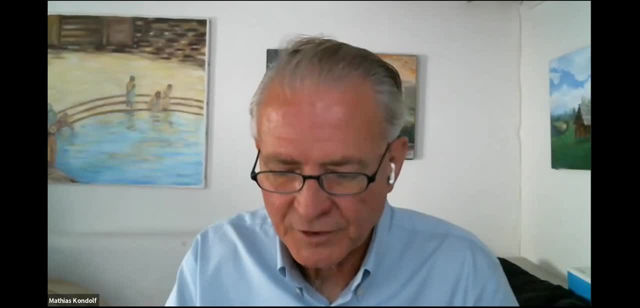 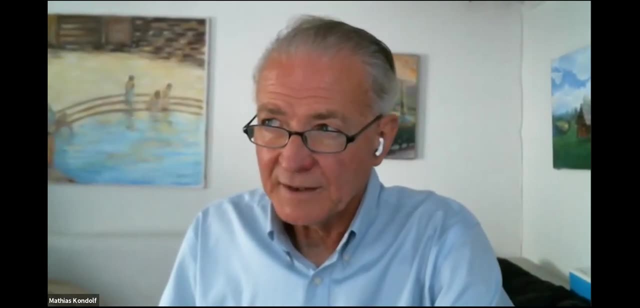 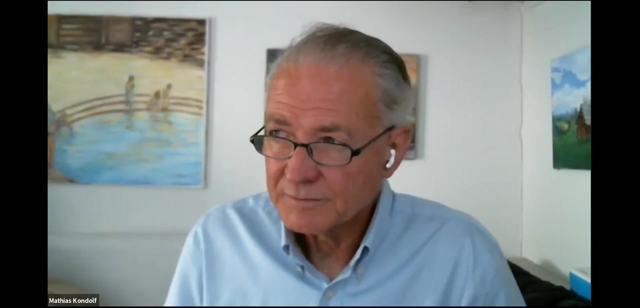 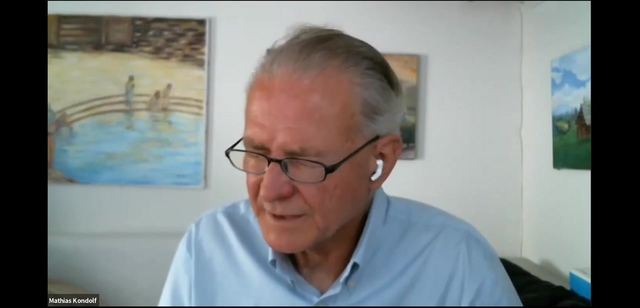 you could say in that case they were certainly. you know they're certainly an intent, or at least a stated intent, to pass sediment through. There are a number of examples of dams built this way: sustainable sediment management in South America, Nepal and Africa. There are a bunch of examples. 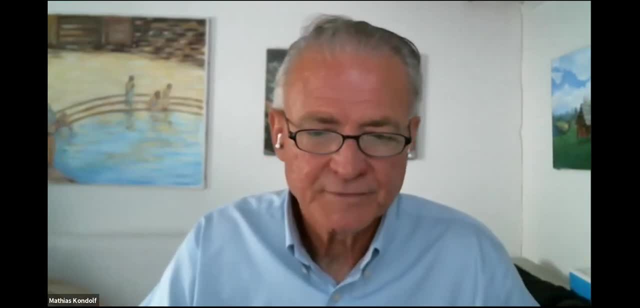 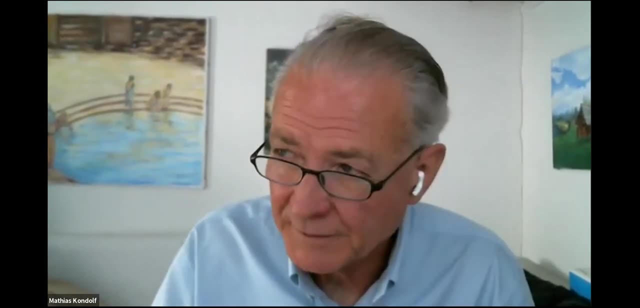 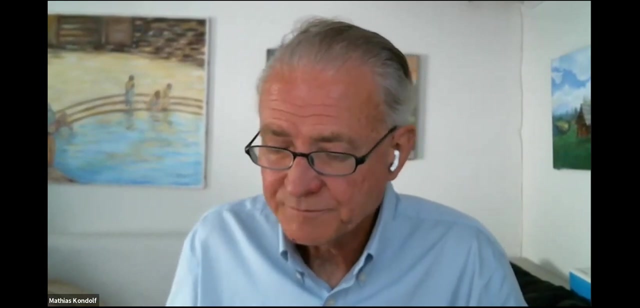 all over, and certainly Japan. Japan and Switzerland are, like the two you know, leading countries for sustainable sediment management innovations, But Taiwan also. I did a study with my former postdoc, Xiaowan Wang. We were looking at how the Taiwanese Water Resources Agency 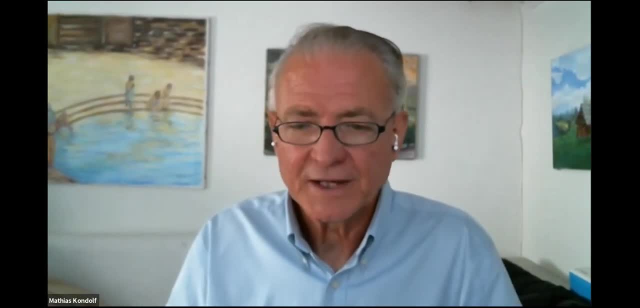 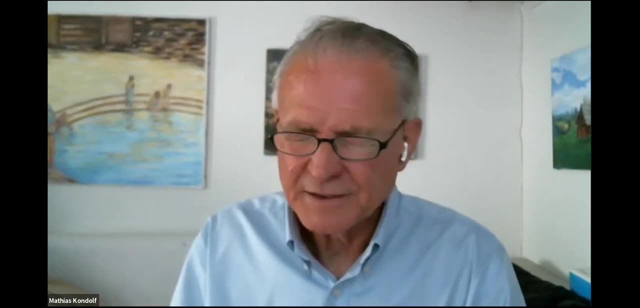 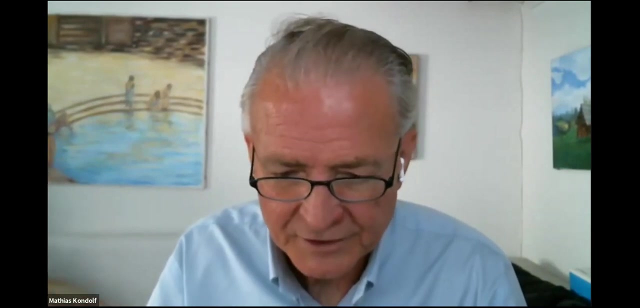 has been trying to implement some of these techniques now and it's been forced on them. They were in denial for a while But it's been forced on them because Taiwan, the central range of Taiwan, you know it's uplifting a few inches a year and it's being eroded at the same rate. I mean they have just 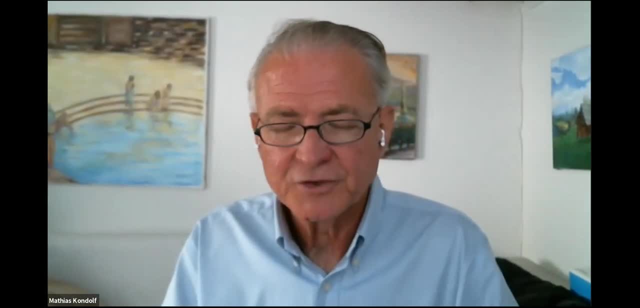 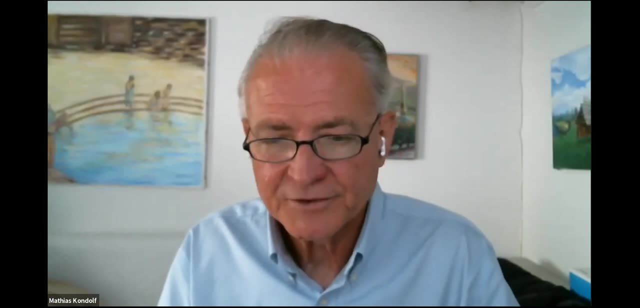 massive sediment loads And, like us, they have seasonal rains. In their case it's monsoonal, typhoonal rains in the summer and it's dry winter. But they depend on sediment, on reservoir storage, just as we do, And so they've been implementing some of this as well. 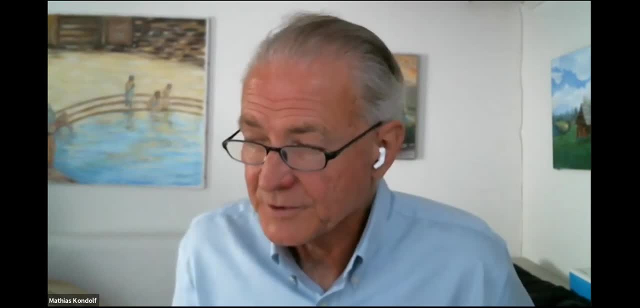 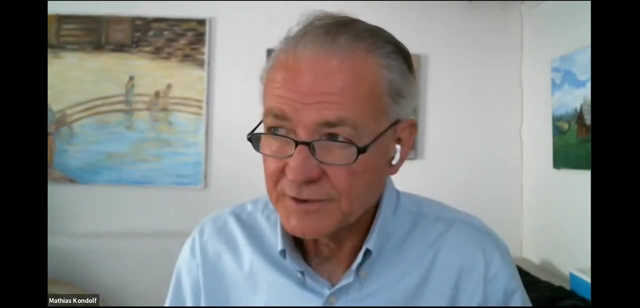 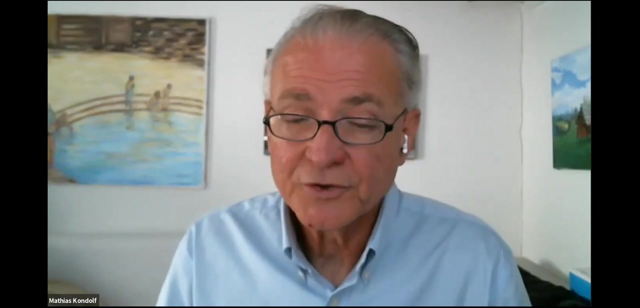 In their case mostly retrofits, But certainly in the case of Japan, some of it's been new dams And some of these other examples I mentioned, like on the Mekong, Nepal and some of the dams in Peru and Colombia, these are new dams that are being built with sediment passage. 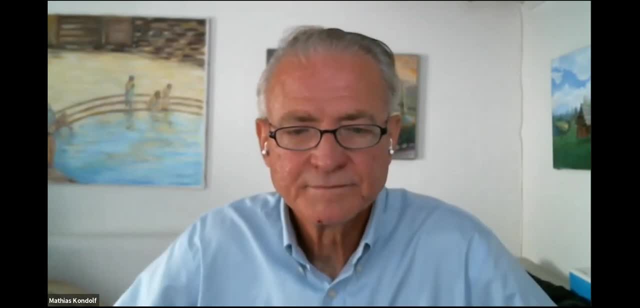 in mind. Thanks. So it looks like I have two more questions from Mike Cox and that's all I see, So if anyone else has any questions, please feel free to ask them in the Q&A box, And I'll see you next time. 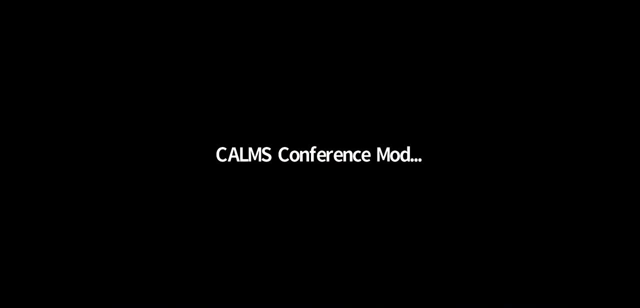 Thanks. So it looks like I have two more questions from Mike Cox and that's all I see. So if anyone else has any other questions, feel free to drop them in the chat right now. The first one is: is there any role of old soil conservation maps in your predictive models? 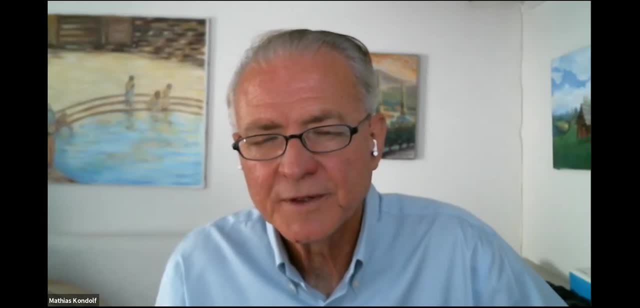 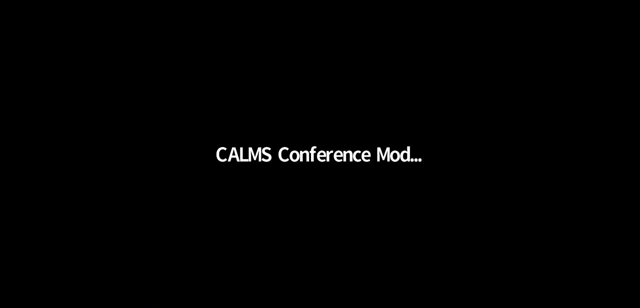 I don't think I quite follow that. Soil conservation maps or spoil. Did you want to chime in on that, Mike? Yeah, thanks. Well, I seem to recall for a while, and at least in the US, they used to produce maps of the susceptibility of soils to erosion. I don't know what they were called or which agency produced those. 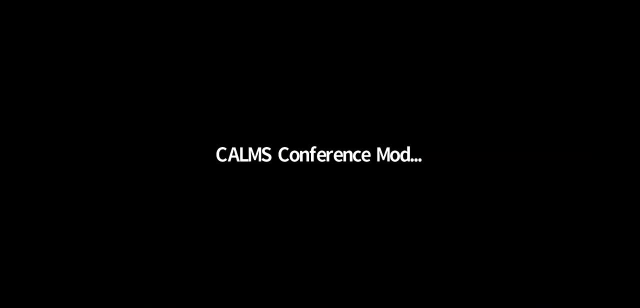 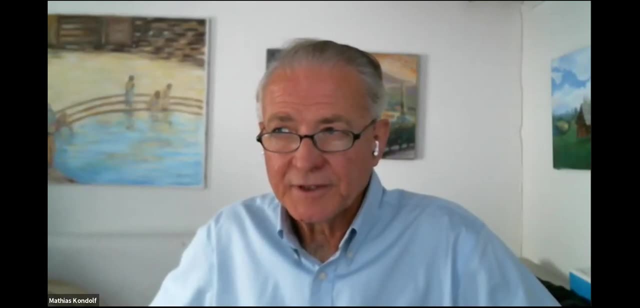 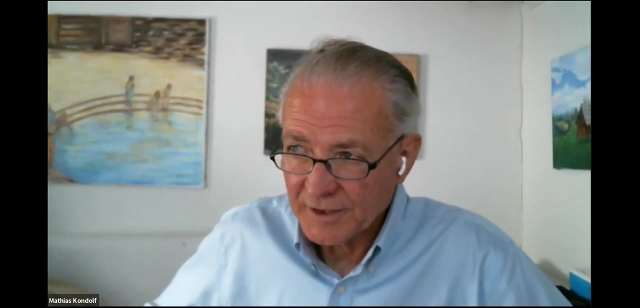 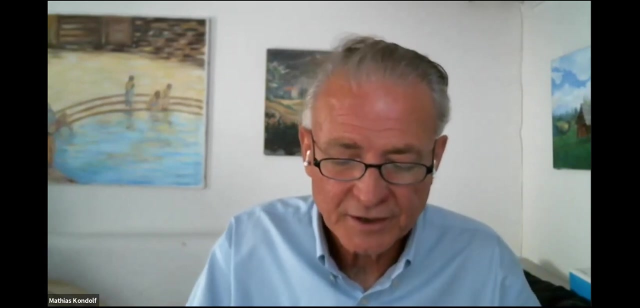 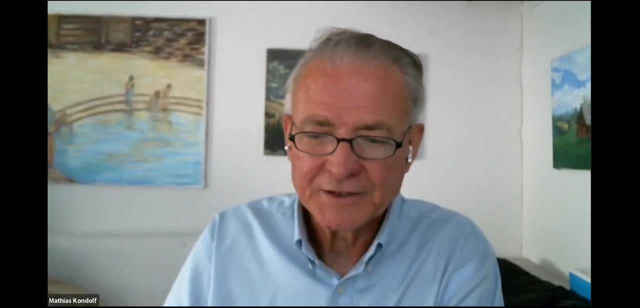 The NRCS maps. Okay, there you go. Yeah, Interesting. Yeah, there certainly could be. That would be a level of detail and- how should I say, a determinism much greater than we employed in our 3W model. We were very empirical and just sort of taking the results. We you know where we had data on how much sediment accumulated in these reservoirs. we converted those to sediment yields based on trap efficiencies and so on. 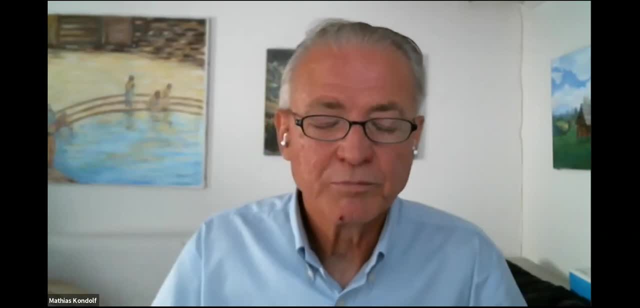 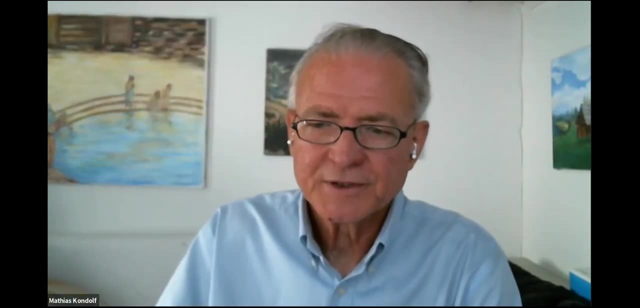 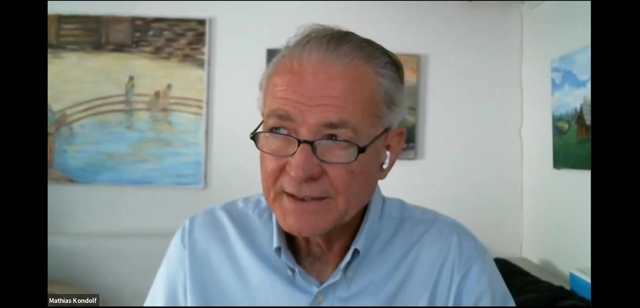 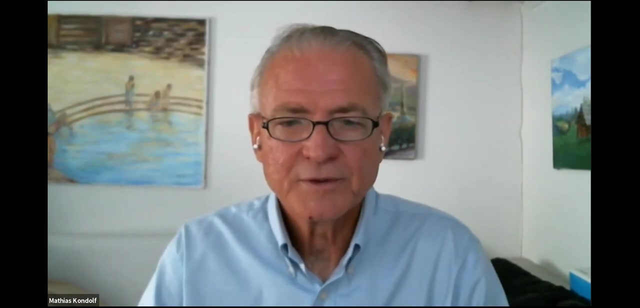 So so so we were, we were really black boxing the whole process. What you're suggesting would be looking more deterministically at where we would expect sediment to be coming from, and how much, And so yeah, so you could certainly improve the models with trying to incorporate some of those kinds of 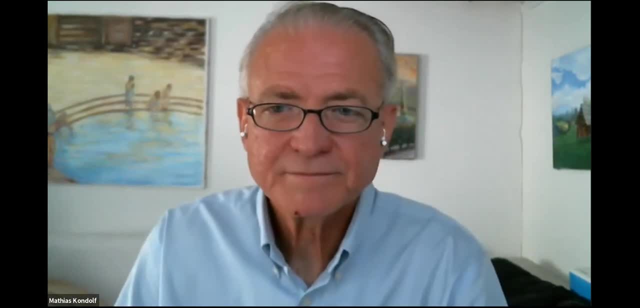 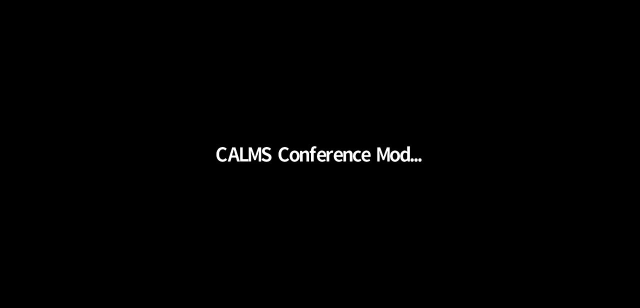 analyses, but we didn't do it And it looks like the last question for you is: Do you use sediment as a source of sediment? Do you use sediment as a source of sediment? Do you use sediment as a source of sediment? Do you feel like sediment total maximum daily loads help, hurt or don't matter in the context of dammed stream sediment management? 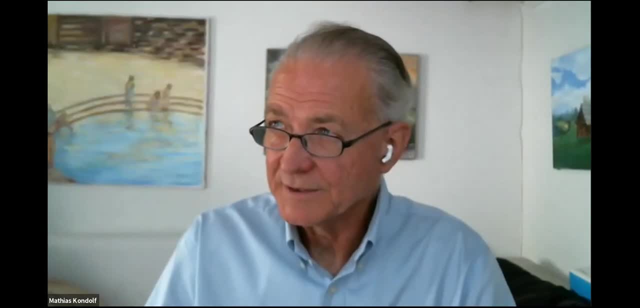 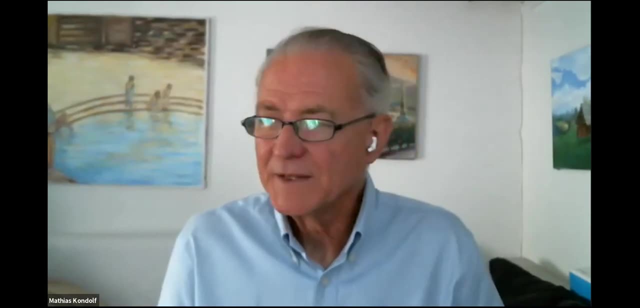 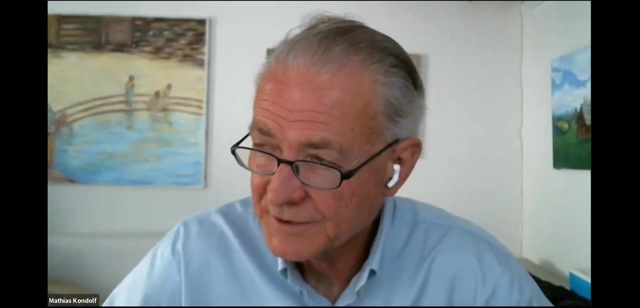 Oh, good question. That's a whole different topic, since we know that total maximum daily loads are not total, they're not maximum, they're not daily and they're not loads. But you know they have served a good purpose in many cases, but I'm not sure that would be the best. 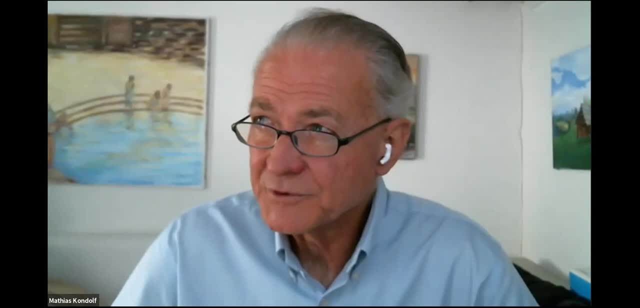 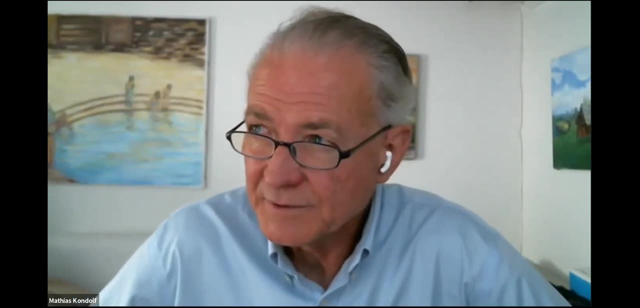 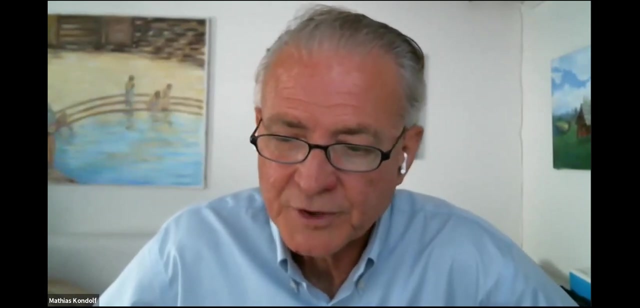 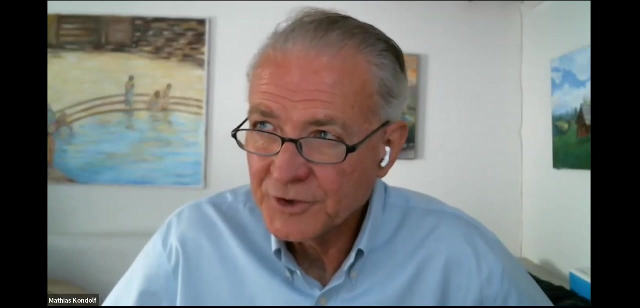 But you know they have served a good purpose in many cases. but I'm not sure that would be the best framework for trying to analyze some of these reservoir sedimentation issues. A lot of it would go back to the conceptual models that people had in mind when, when the Clean Water Act was written, and no sediment was pretty much treated as a pollutant at that point. And now you know we're trying to say there's, you know there's good sediment. we need sediment in some cases. So